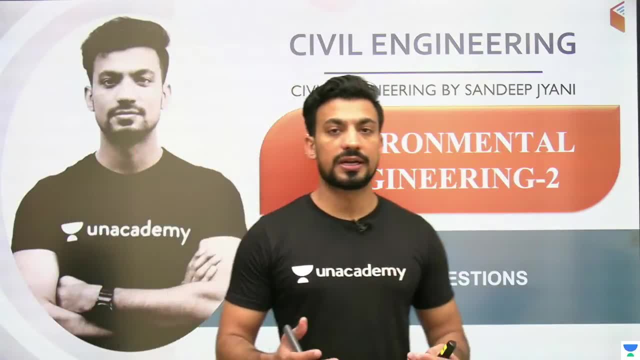 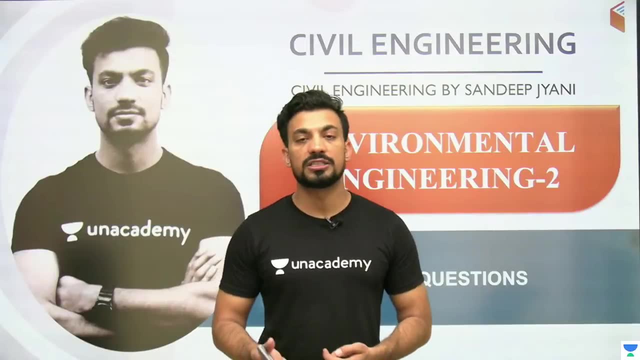 Let's study about this. If you are working in industries, if you are producing anything in industries, then some of its by-products, they will become waste. How are we going to manage it, Whether it is domestic, whether it is there? 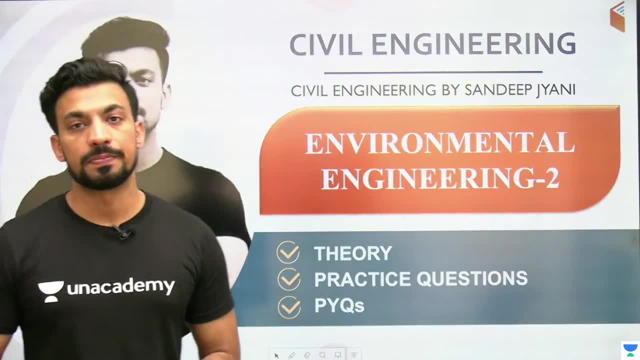 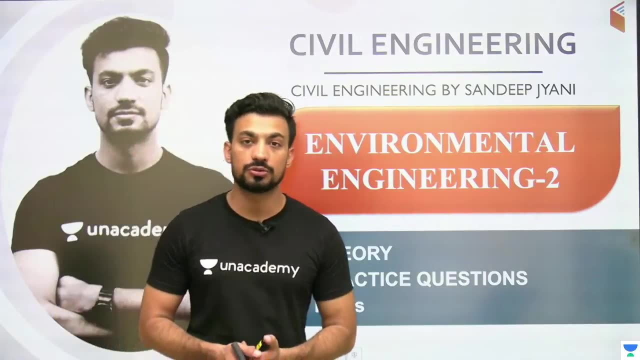 the solid waste that is being generated? how will we handle it? What about the air that we are polluting? How will we handle it so that our environment is not spoiled? We will talk about all these things. So till now, we have covered the part of wastewater engineering. 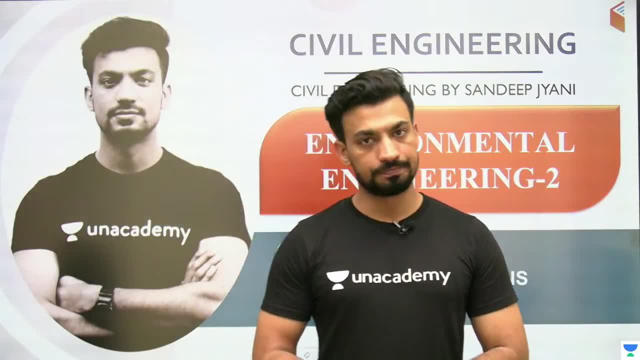 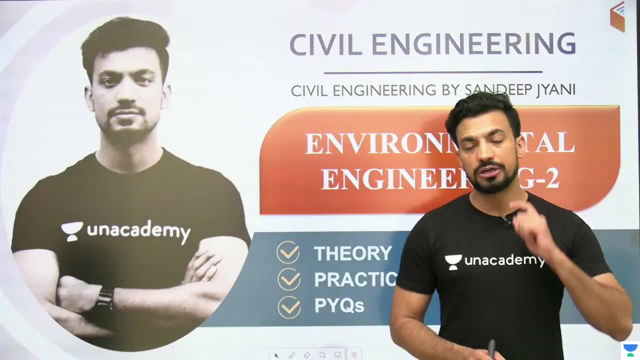 If you have not studied it yet, then you can study it. And now what we are starting? that is all about solid waste management, which is generated by solid waste. We have already talked about liquid waste. We have already talked about sewage. 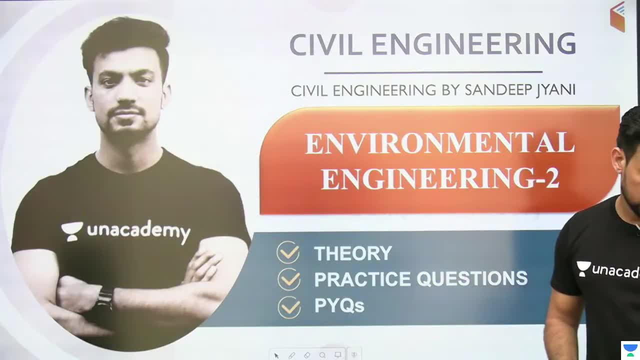 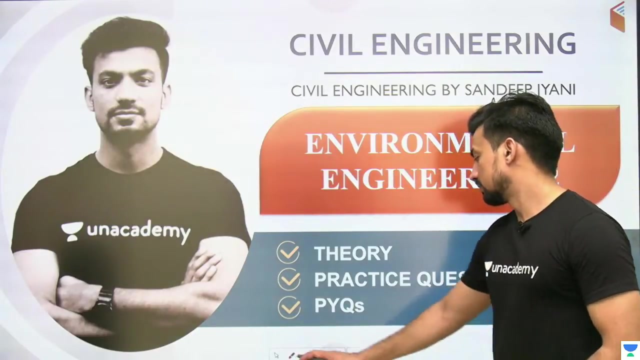 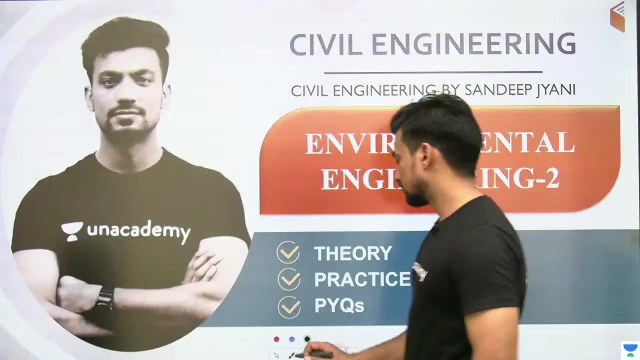 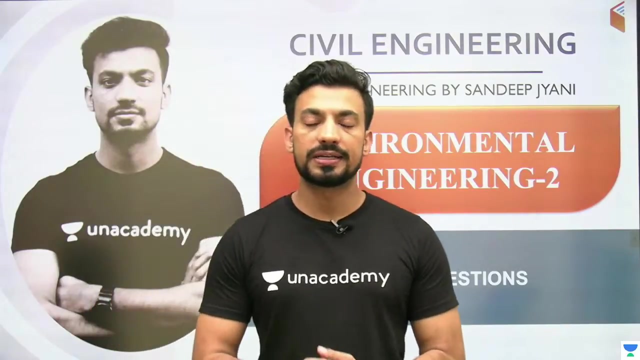 And now we will talk about solid waste management. We will talk about solid waste management. So, friends, as you all know, Unacademy is India's largest online learning platform where you can prepare for your dream exam. For this, friends, now, 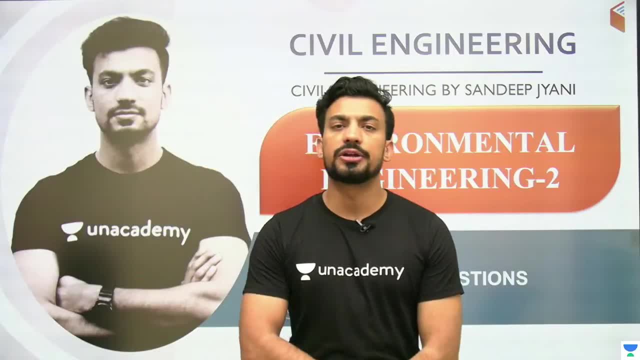 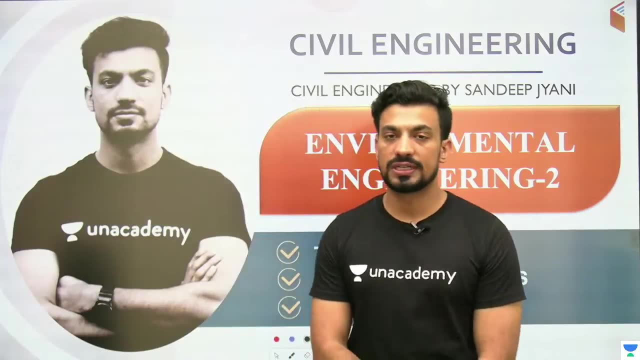 SSC, JEE. you know the result of paper 1 has also come tomorrow, 2020,. I hope you have checked it, And if you are preparing for paper 2, then for this. today we are talking about friends, how we are going to proceed further. 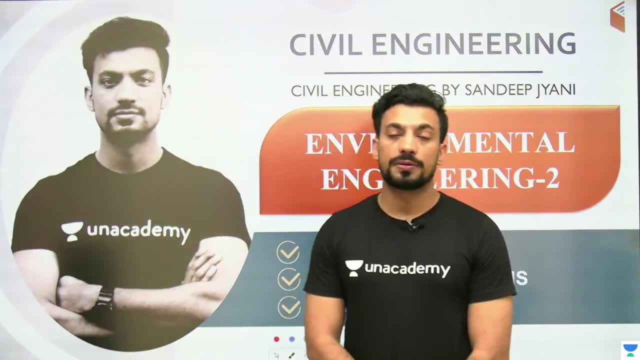 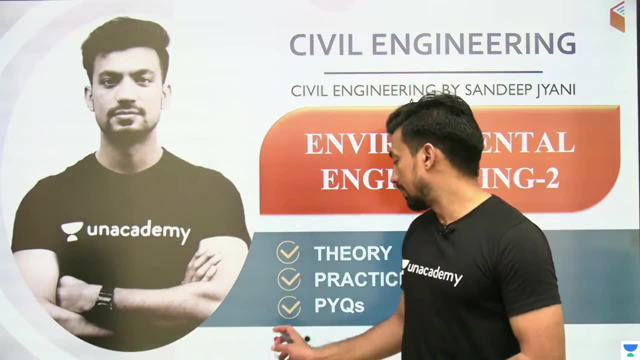 After this session we will talk in another session And along with that, friends, you can read the new subject, Highway Engineering, which we have just started on Unacademy. You don't have to do anything to read it on the Unacademy app. 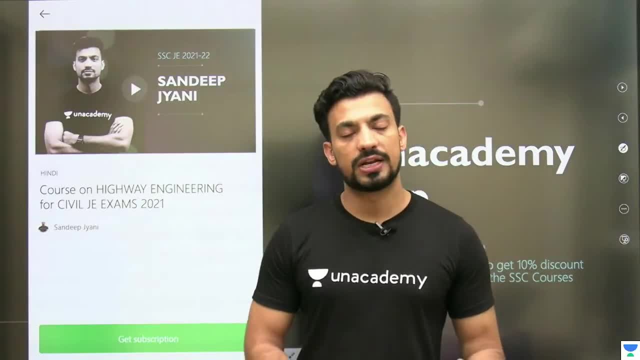 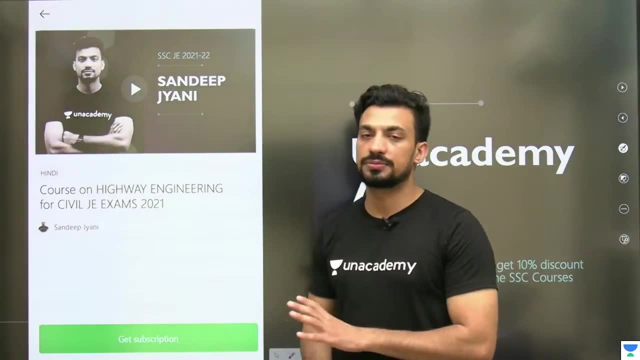 Here you will see the course. If you have a subscription, then you have to click on Get Subscription. If you have a subscription, then you will see the enroll button. If you don't have a subscription, then you have to click on Get Subscription. 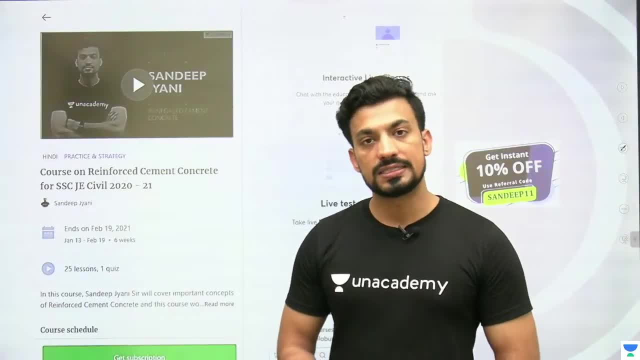 Then you have to select the duration. After that, you have to use the code Sandeep11.. As soon as you use Sandeep11, you will also get 10% off And along with that, you will get access to. 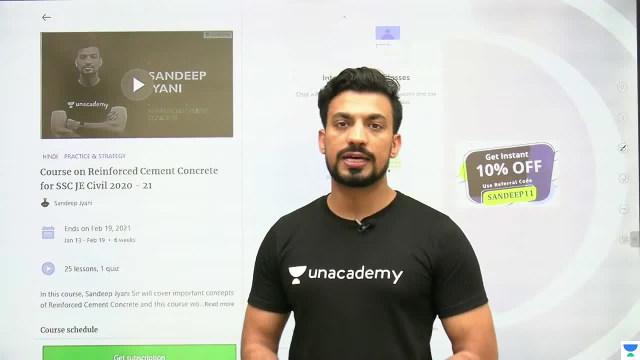 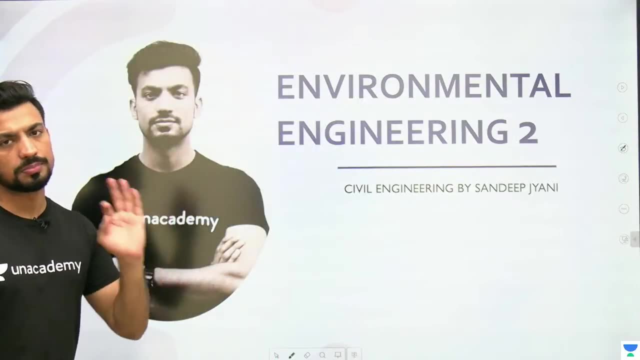 Unacademy platform. throughout the category You can see any class of any educator. Friends, let's talk about Solid Waste Management In Environment Engineering 2, there is a very small and very simple topic which you can relate easily, which you can understand easily. 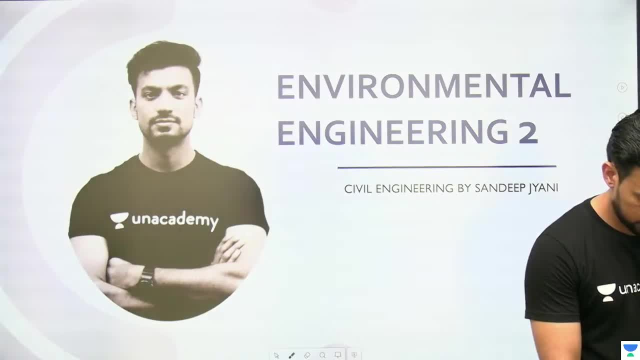 So much in it, Let's go to Solid Waste Management. I will talk about Solid Waste Management. Ok, now, that's fine. No, class is not today evening. Today is only the morning class. There is no class today evening. Ok, so we are talking about. 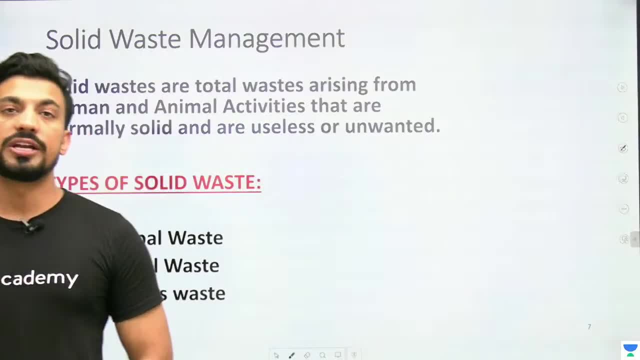 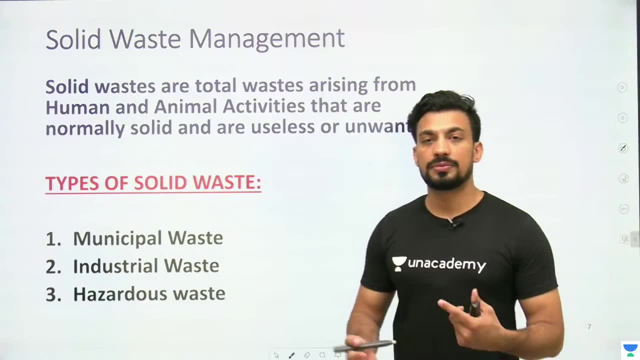 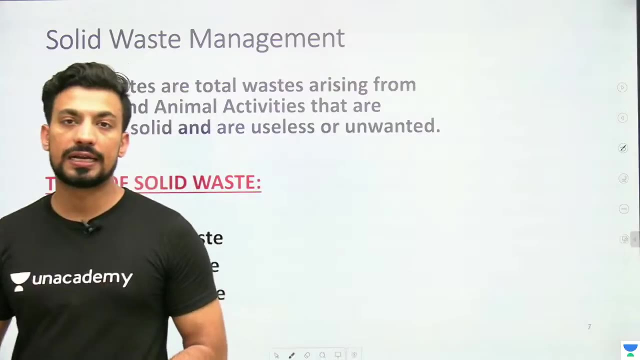 Solid Waste Management. In Solid Waste Management, what we talk about. What is Solid Waste? Solid waste, whatever you are, either for domestic purpose or for industry purpose. whatever solid form waste is generated, How to handle it. What will be the solid waste generated in the house? 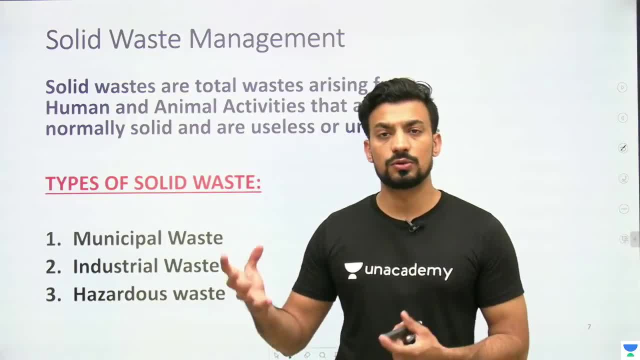 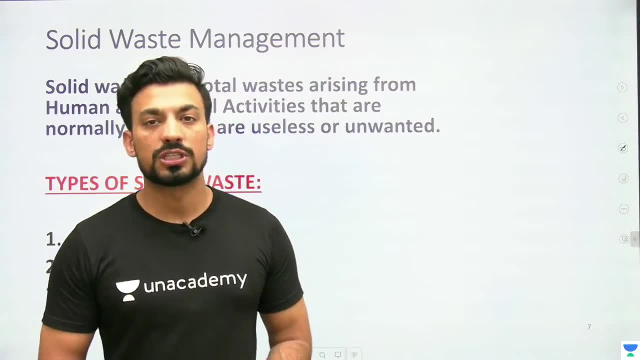 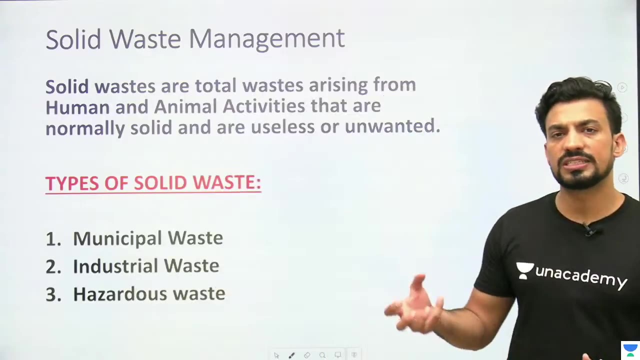 In solid waste. you will say that when cleaning or dusting is done, then the dust that comes out of it will become solid waste for you. If you burn something, then what happens to the ash that becomes solid waste for you. If vegetables are cut, then what is the waste generated by them? 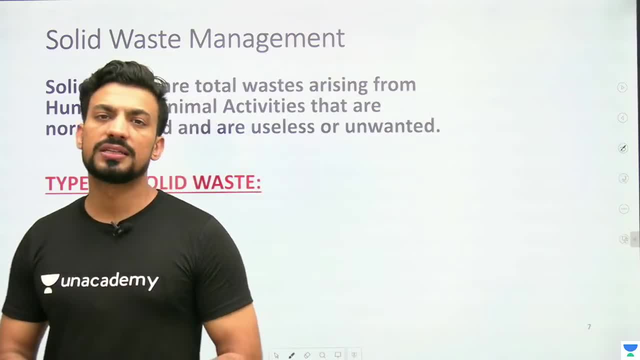 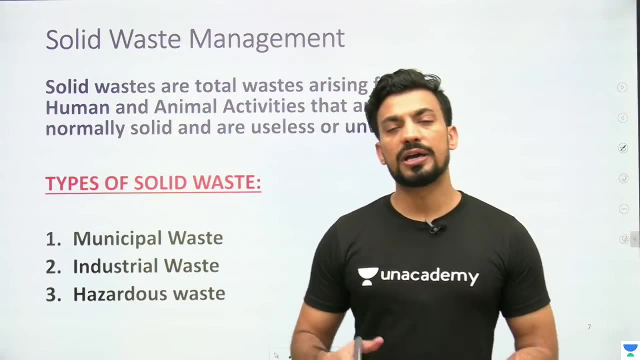 What happened to you? Solid waste happened. You bought any packaging material, any snacks. then, whatever the wrapper is, whatever the plastics are, what happened to them? Solid waste happened. So if we talk inside the house, if we look inside the domestic area, 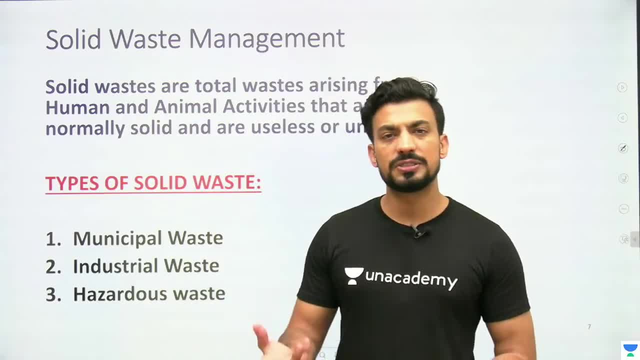 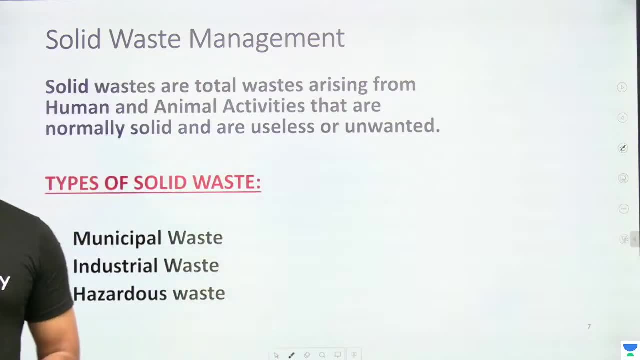 then a lot of solid waste is generated here, Whatever we put up in the dustbin. what is all that Solid waste, or whatever we put in the dustbin? So how will it be managed? Let's talk about this. So we categorized solid waste in three ways. 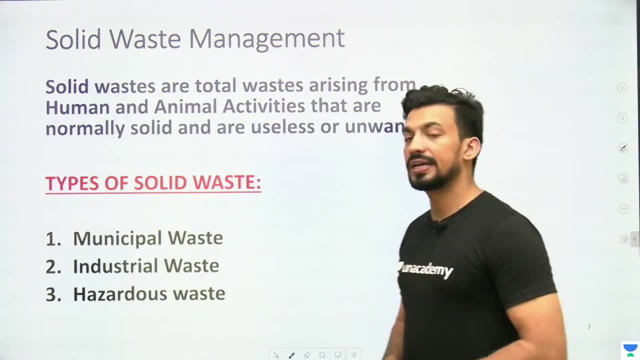 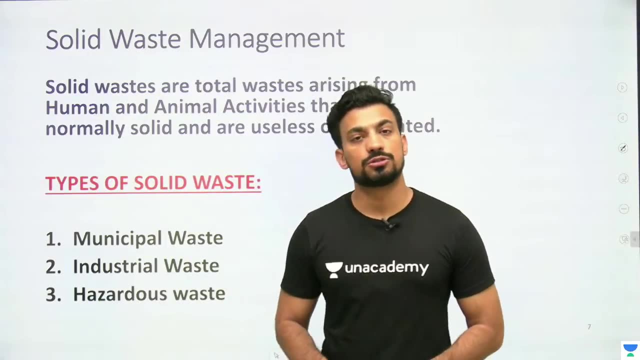 How did we categorize it? in three ways: One is municipal waste, One is industrial And one is hazardous waste. The simplest objective question that has been asked so far is that: what are the types of solid waste? So there are three types. 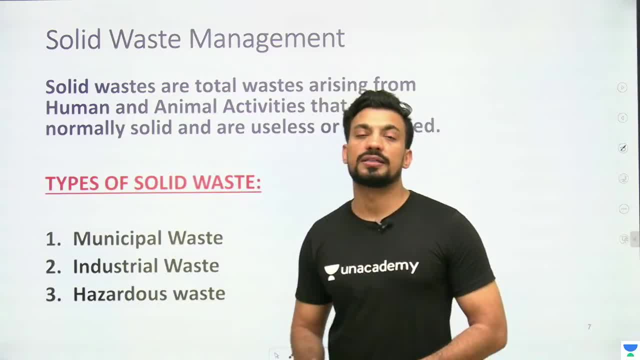 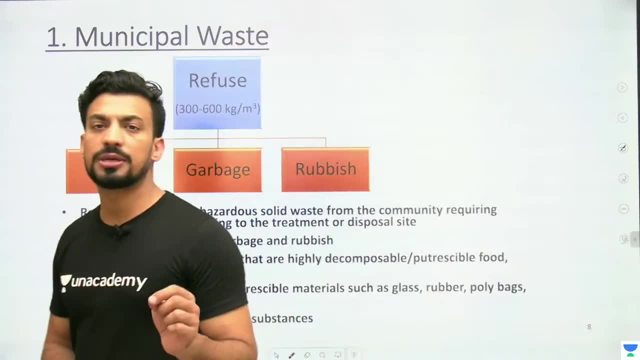 Municipal, industrial and hazardous. These are your three types. If we talk about municipal waste, then any waste that is not of use. what is it? It is refuse. What is not of use, what is it? It is refuse. So if we talk about refuse, then municipal means we are talking about the domestic one. 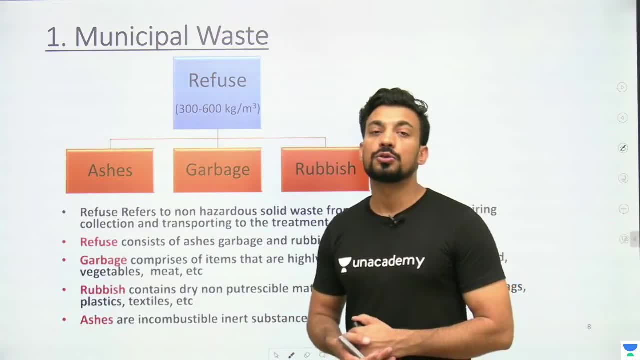 If you look around your house, then what are the things that are refused in it? What are the things that are refused in it, What are the things that are not of use to you? So the first thing that comes is ash. What does ash mean? 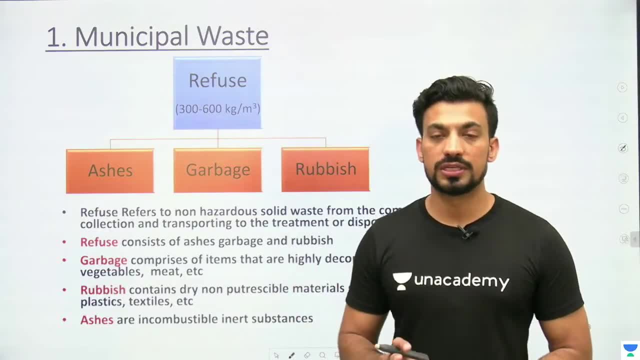 The thing that has been burnt. The thing that has been burnt, So what is that? It is ash, So you have ashes. Then comes garbage. So what things do we include in the garbage? In the garbage, whatever rotting things are there. 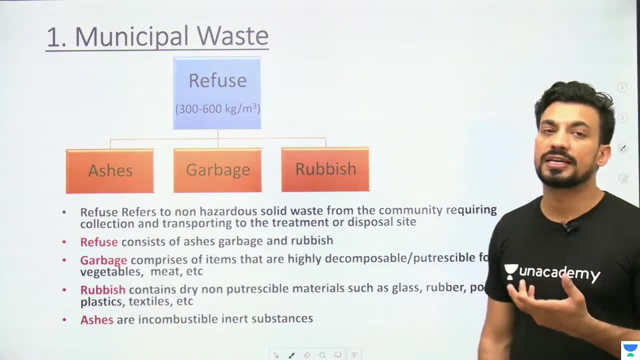 You can say, like this, here Which can be decomposed, Any food, The food that was eaten last night Or whatever has happened in the morning, So that which has gone bad, Fruits and vegetables, What is that? What is that? 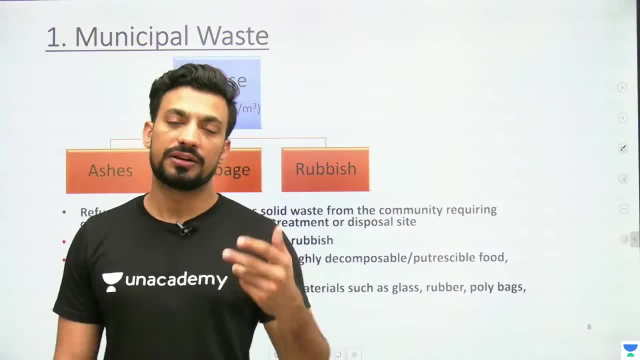 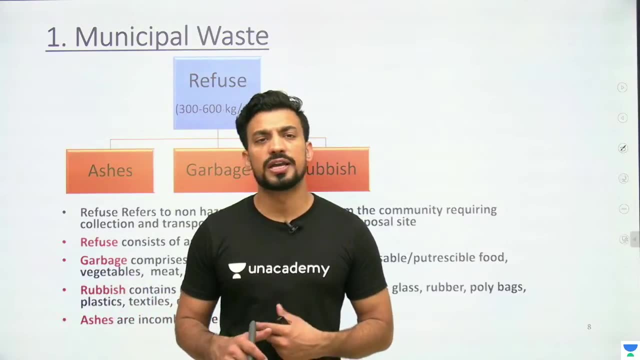 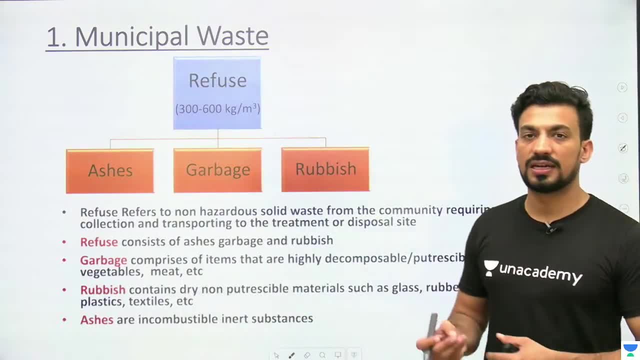 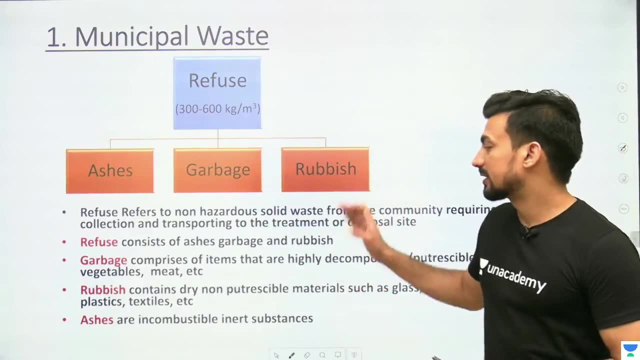 That you have Putrescable Means, that which can be rot, If there is any material that is rotting, It all comes in the garbage. And if we talk about rubbish? So what do we say in the rubbish? The dry waste is there. 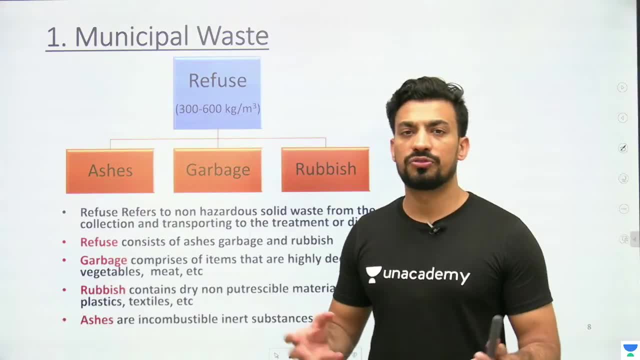 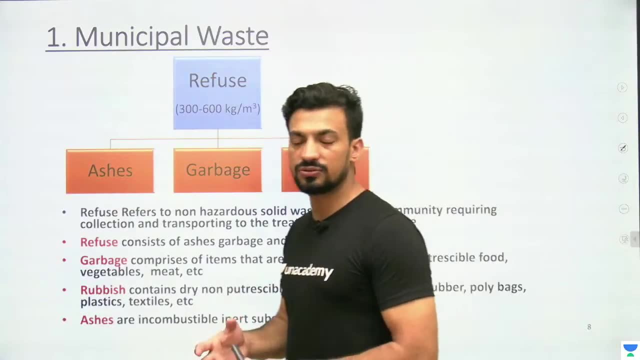 Dry waste That won't rot, Just like paper pieces have happened. You have any furniture Which is the broken furniture That happened, So such a thing that doesn't burn Generally, Sorry, and it will be dry. what will it be? It will be dry. 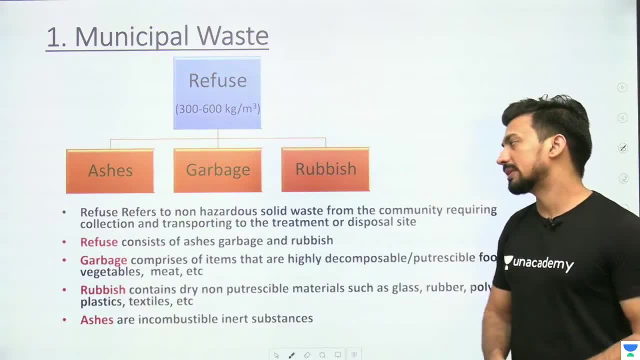 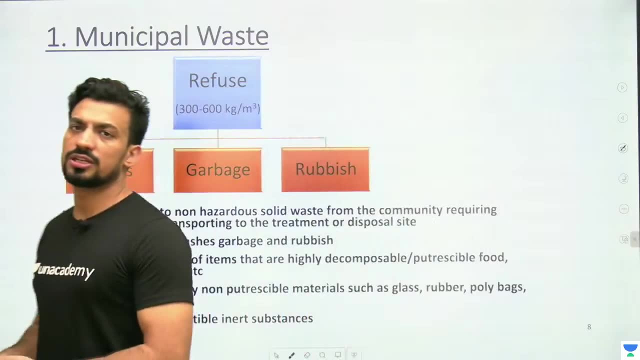 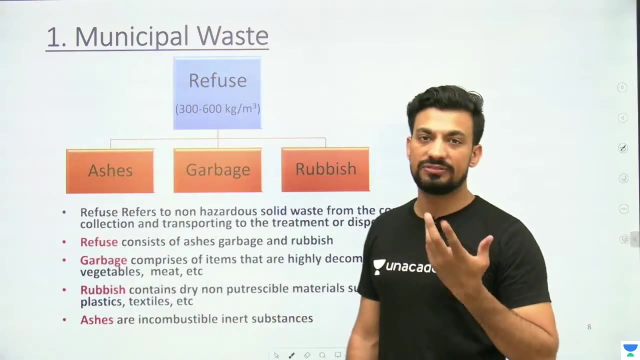 So let's talk. refuse means any such waste which is not of your use, And in refuse generally, in refuse whatever our domestic, because we are talking about municipal waste here, so in this waste you don't need to take any special precautions to collect such waste. 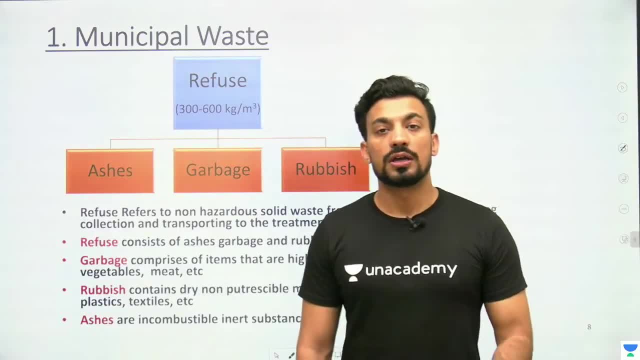 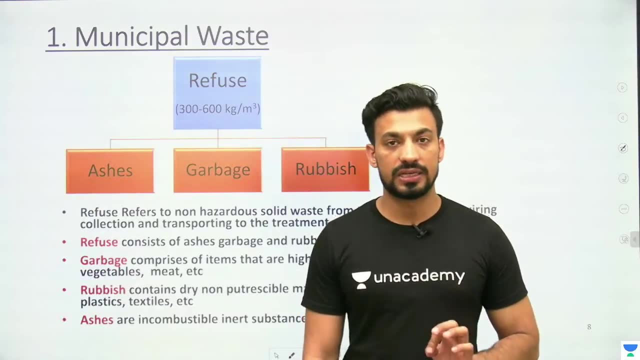 Like there is a hospital, so whatever the waste of the hospital will be, to collect the waste of that hospital and to dispose of it or to treat it, then you should take a lot of precautions in this. Why? Because it is a hazardous waste there. 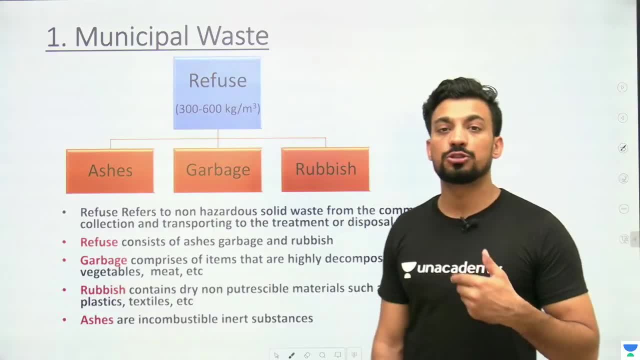 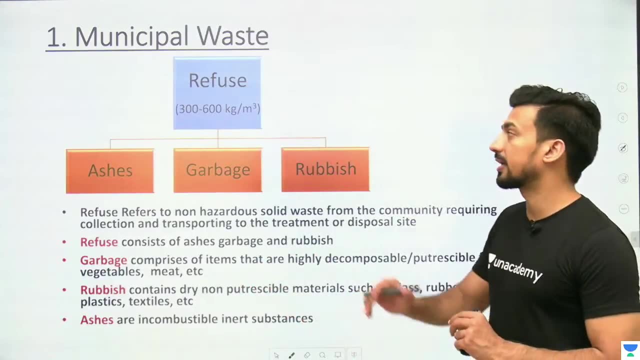 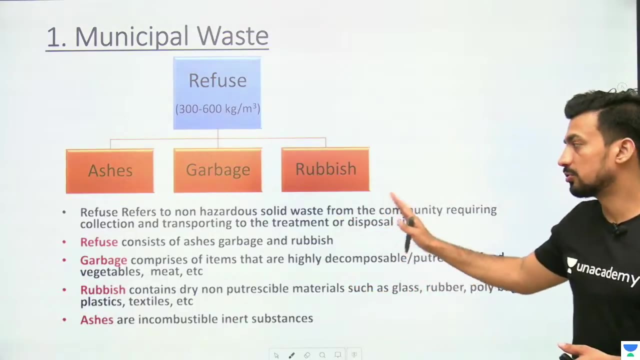 There is such a waste there In which there are bacteria which is infected, so it can be harmful to you. But here in general, if we talk about refuse, then what is our refuse? What is municipal waste or whatever is not of our use in your domestic waste? what is that? It is refuse? 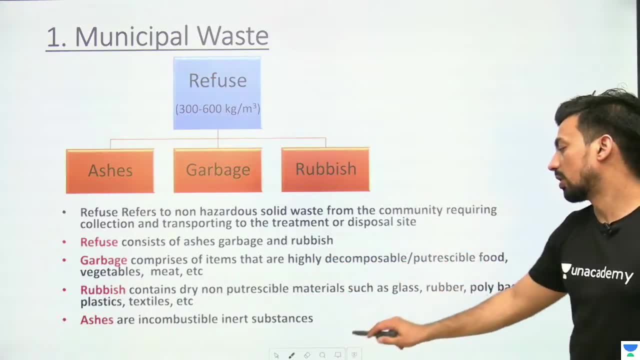 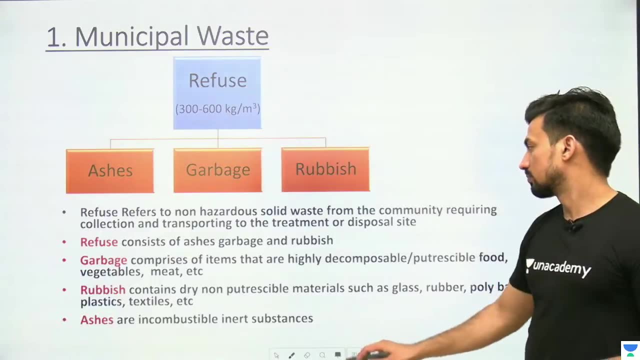 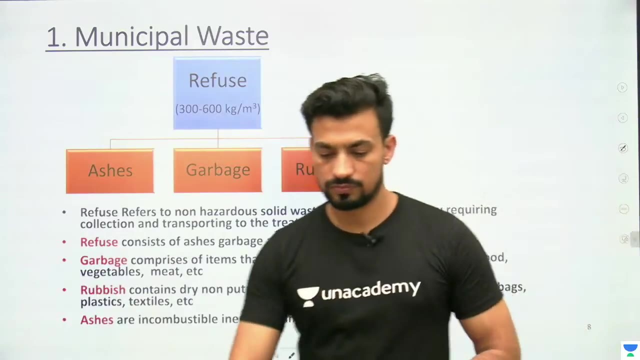 Garbage comprises of items that are highly decomposable, which is very decomposable. decompose quickly If it is not of our use, but whatever. So in some cases, for example, if you are doing a bigger project, then we are talking about miscellaneous items, or if it is about smaller items, 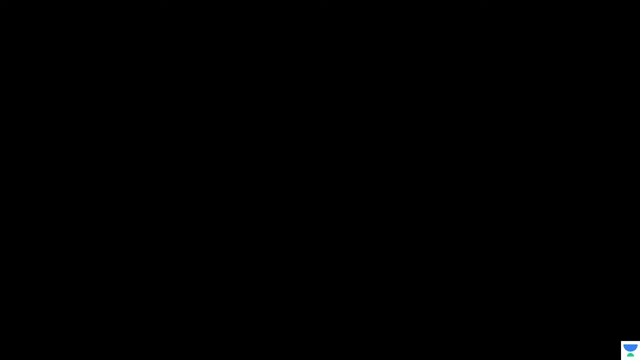 for example, you are talking about things like quantity of garbage that are stored in a plastic bag. in your house, for example, you might want to collect all of those items that are not of your use when you are doing a downsizing project. So in some cases, you might want to collect all of the things that are placed in a plastic bag. 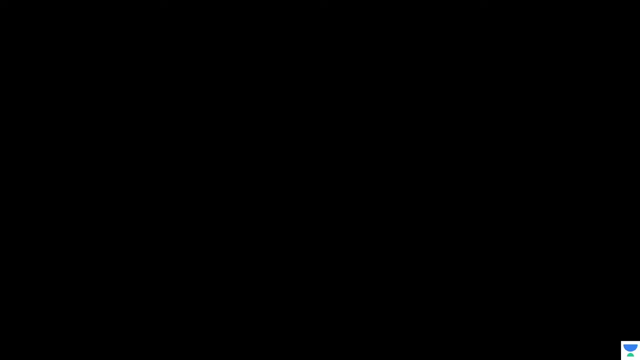 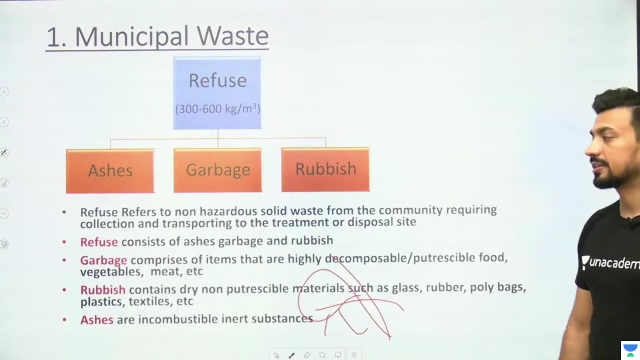 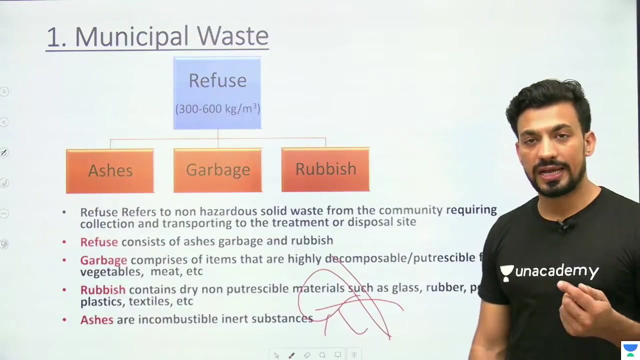 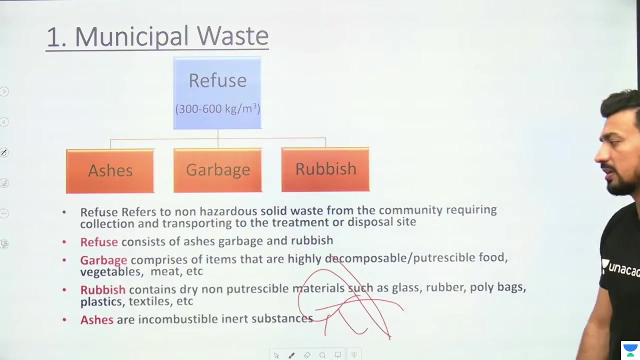 Again, they are not of our use. So now let's talk about the garbage that comes to you: Garbage that can rot, which is rubbish, which is dry waste. dry waste, such waste that does not rot, like if you have pieces of paper or some wooden furniture. these are all plastic or something like that. 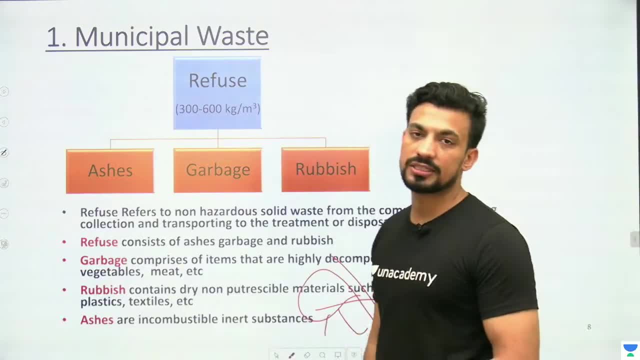 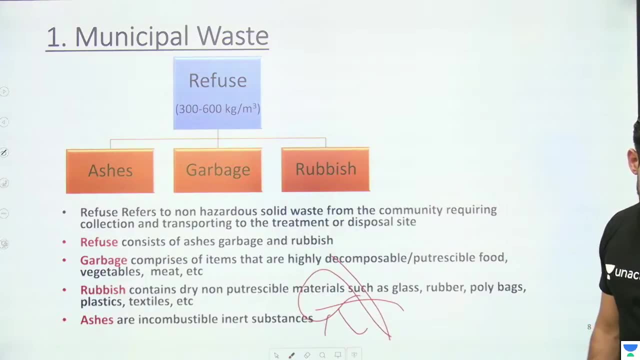 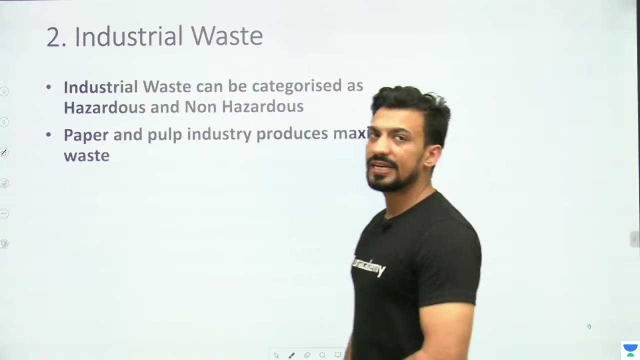 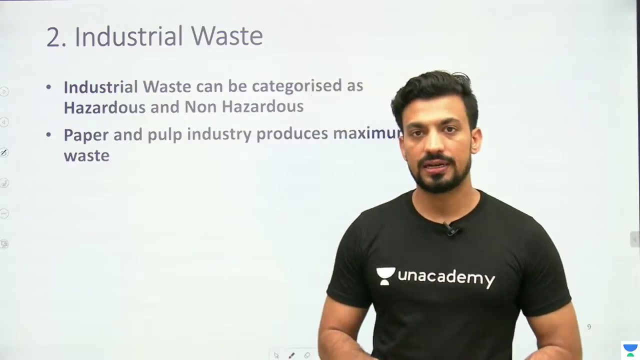 Ashes that cannot burn, which has already burned. if we talk about ash, then it will come to you here, Let's move on. Next comes the waste generated in the industry. let's talk about industrial waste. So industrial waste can be of two types, such as hazardous- now what is hazardous, let's talk about it next- or non-hazardous. 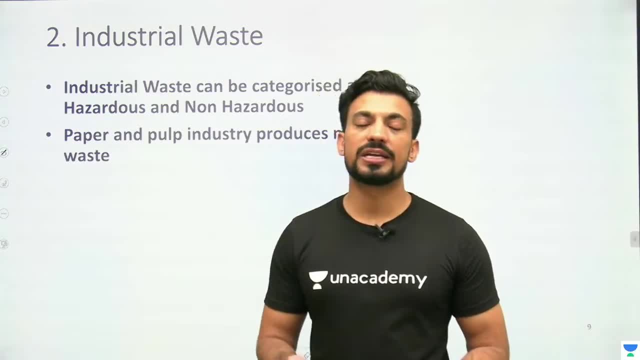 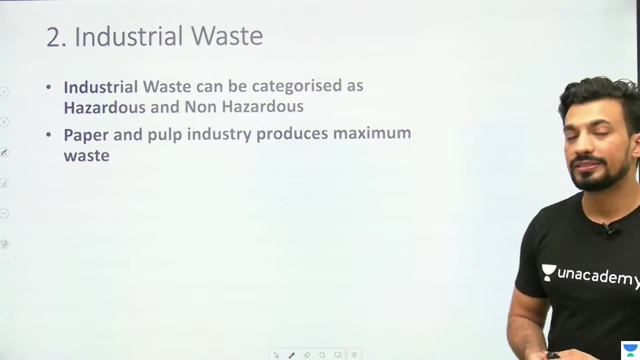 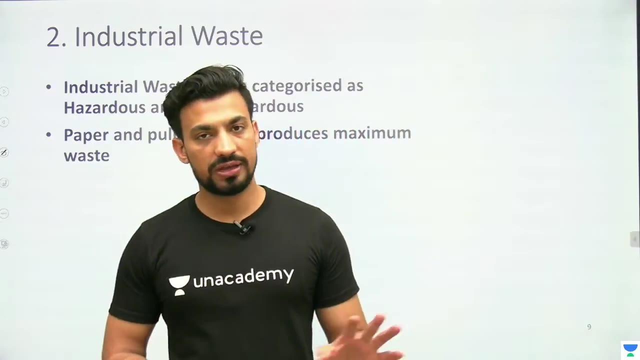 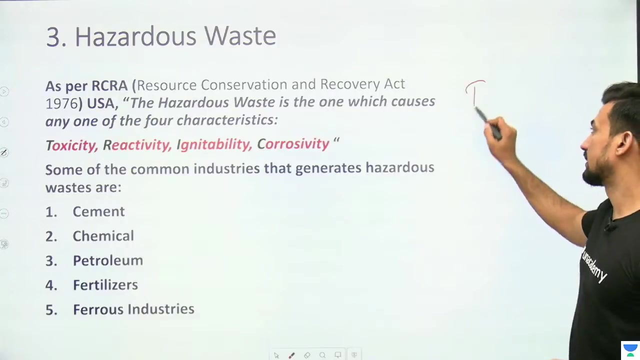 So hazardous or non-hazardous depends on what type of industry. it is the type of industry. it is the type of waste that will be generated there. according to that, we are going to see there, as you all know, the paper and pulp industry generates the most waste, just an example. that industry to industry it is going to vary. and now if we talk about hazardous waste, then there is a trick for hazardous waste. what is hazardous waste? what is there to remember it? there is a trick. what is the trick? 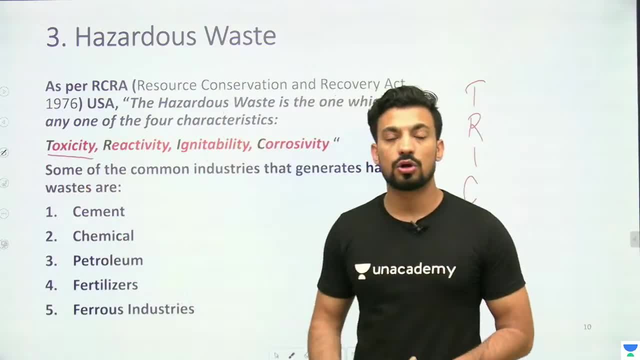 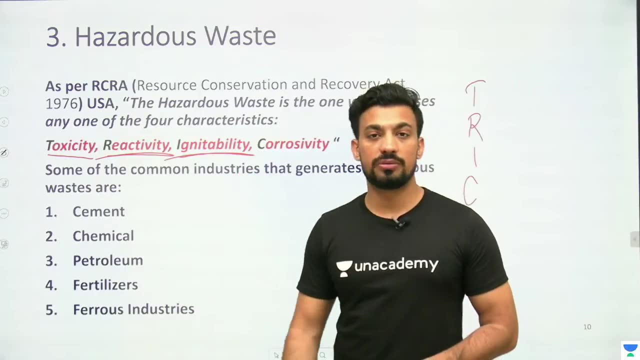 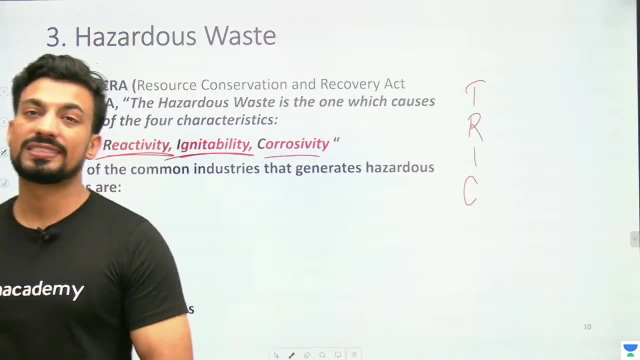 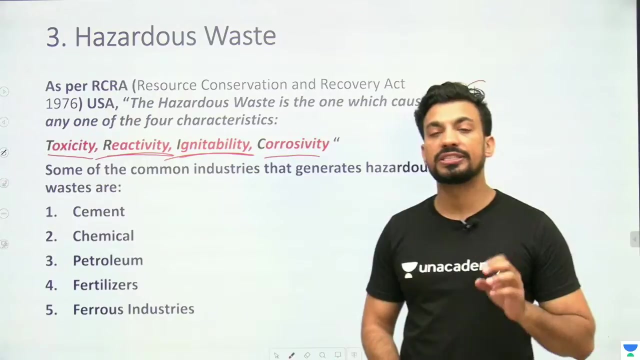 Anything that is toxic, which is toxic, poisonous, it can react, there is reactivity in it, it can burn, it can be ignitable and it can damage anyone in contact. it can create corrosion. it is corrosive. So for this we say that it is hazardous. Anything that is toxic, is reactive, is ignitable, is corrosive. what we call it, we call it hazardous. 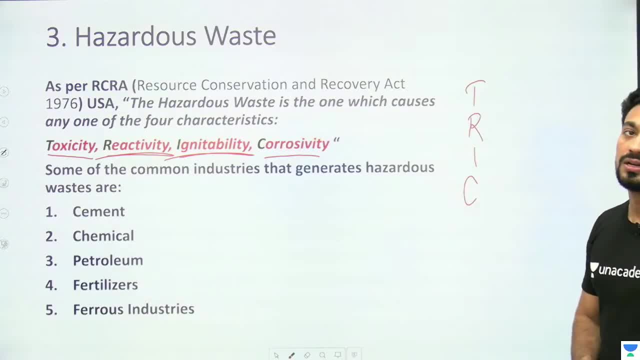 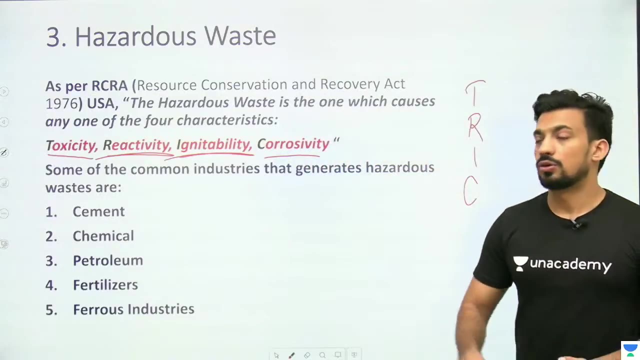 Conservation and Recovery Act 1976 of USA, the hazardous waste is the one which causes any one of the four characteristics. if any one of these four is present, then we say that it is hazardous waste, be it toxic, be it reactive, be it ignitiable, be it corrosive. 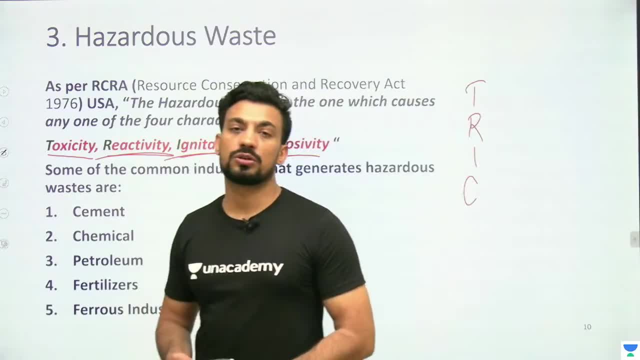 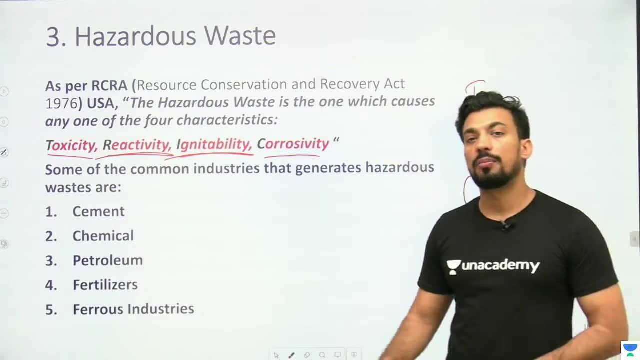 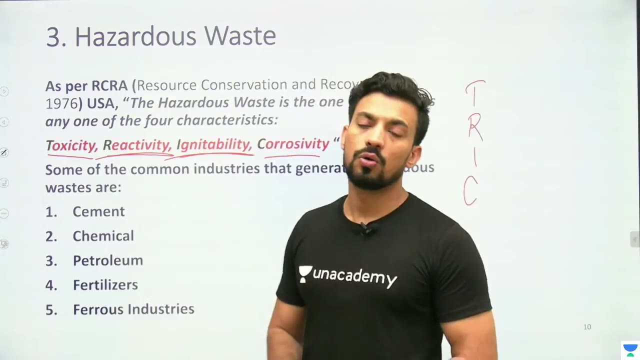 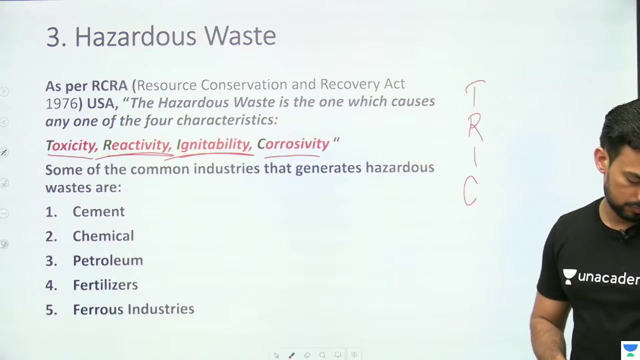 What are the industries? if we see some of the industries then we need to say: in cement or in the chemicals? this chemical industry, petroleum industry, fertilizers, or the one where your ferrous or the iron is used. obviously there will be corrosive eating. 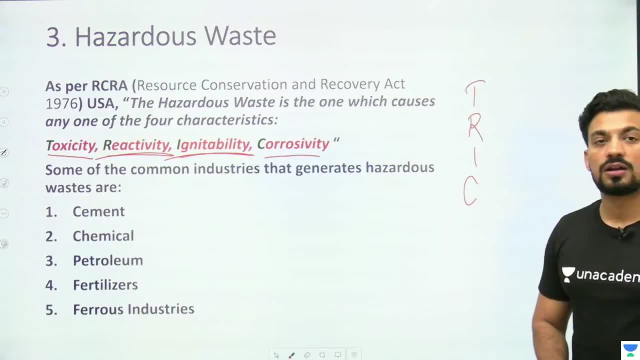 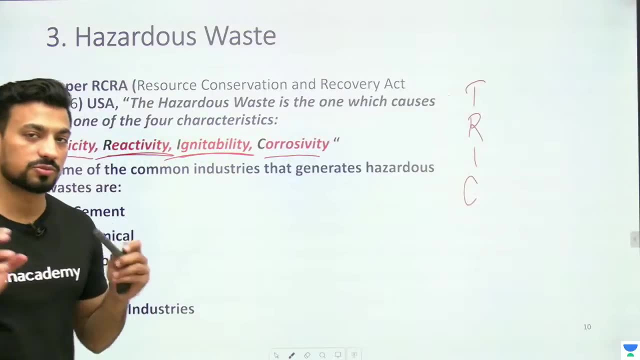 What is garbage? decomposing Garbage? you close the dustbin for two days and see, do not open the dustbin for a few days, put it in the peel of vegetables, fruits, vegetables, and close the dustbin after that. you see. 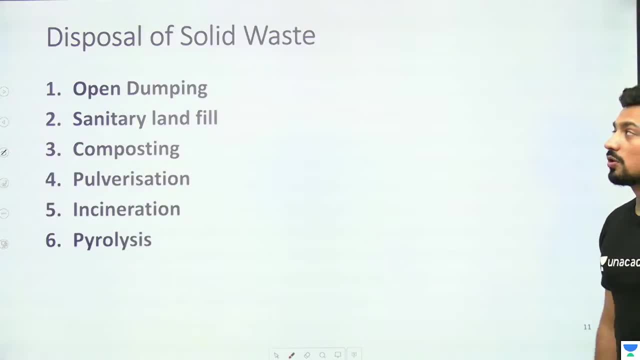 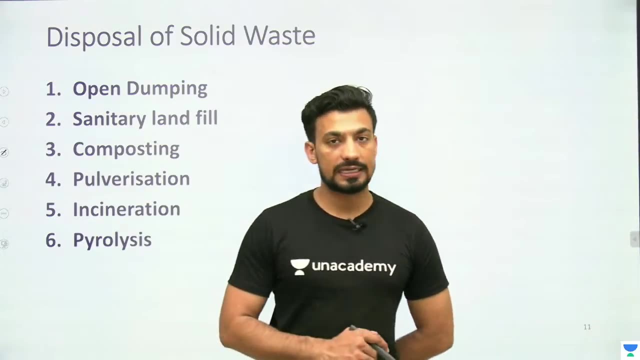 Next, disposal of solid waste. how to dispose of solid waste, how to dispose of it that it should not be harmful to the environment. The first way, the simple way, is that throw it anywhere you can see it, such as in the. 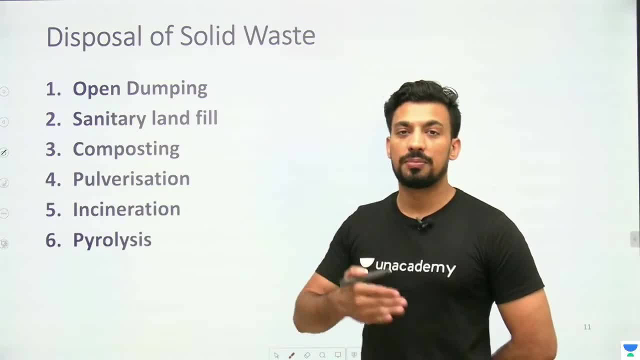 garbage dump, as people often do, where your house is. there is a house on the side. there is a house on the side. there is no house behind. there is an empty plot. it went to the roof, but you should not do this. 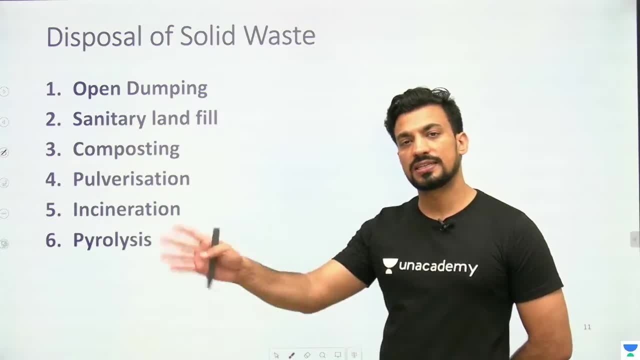 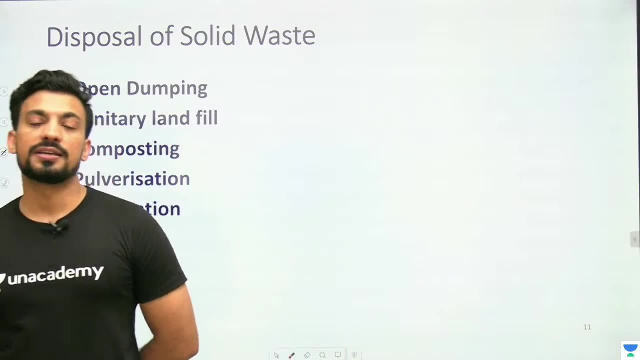 Open dumping. you must have seen somewhere nearby. some areas are definitely like this, where there is such a place around the entire locality where everyone comes and throws garbage. It is okay to say that there is a public dustbin or they are there, but those things 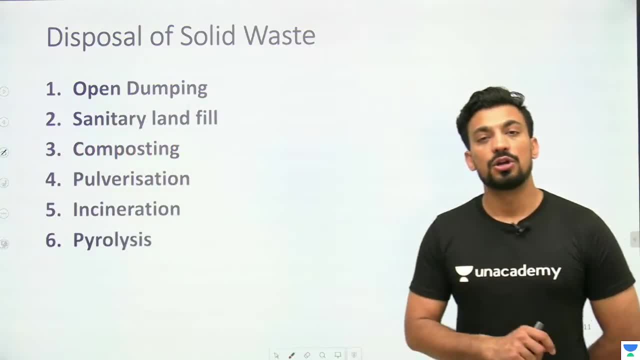 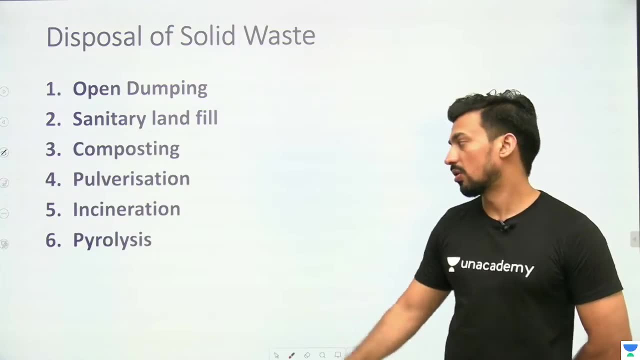 are lying around it. So open dumping is not allowed. it should not be done. You have sanitary landfill: composting, pulverization, insulation and pyrolysis. Open dumping method is simple. there is no need to put much engineering in it. take out. 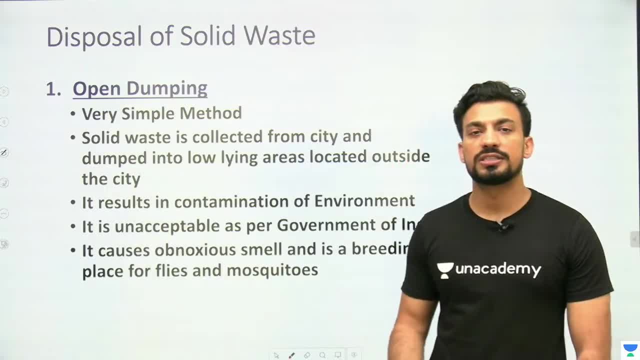 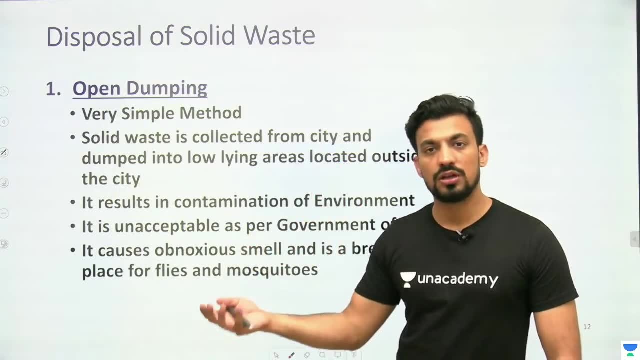 the garbage from the entire city. wherever there is garbage from the city and you go to such a place, that is, go a little far from the city, go to that locality and dump that garbage openly. dump it openly there and throw it. 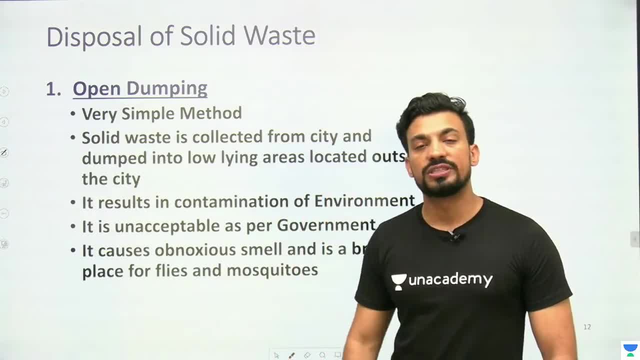 So this is not right. it will be in the open area in the open area. it will be in the open area. If the environment is exposed, then what will happen there? it will spread diseases. if the waste is reacting, then it will react if the decomposition of that waste is happening. 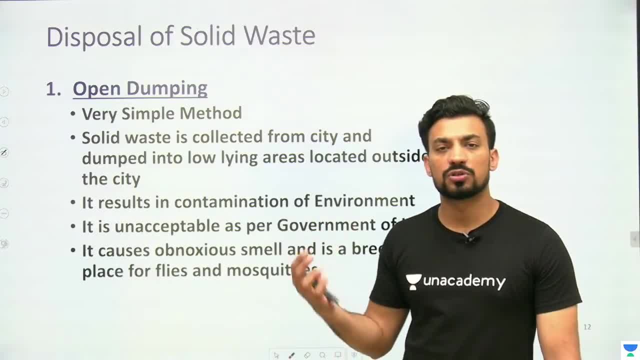 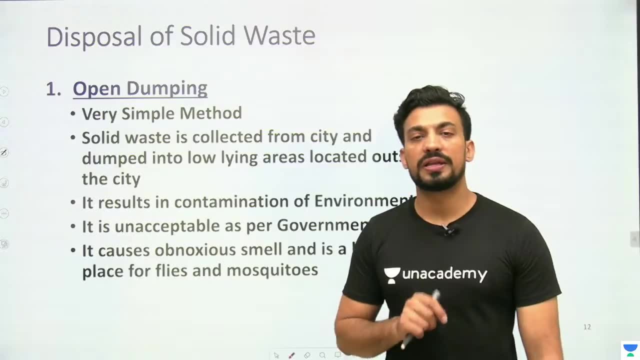 then the decomposition will happen. gases are being released, flies are coming, mosquitoes are coming, whatever, all things are there, the whole environment of spreading diseases becomes there. So that's why it is not adopted. that's why it is not favored. it harms the environment. 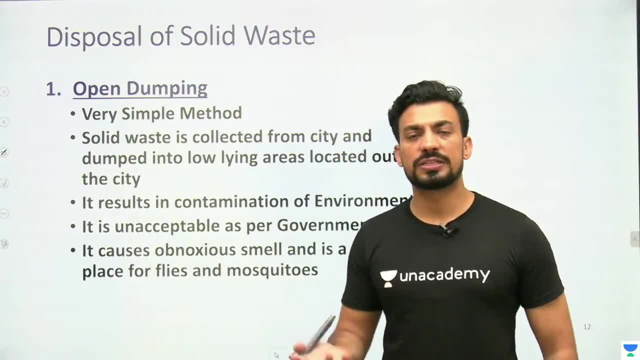 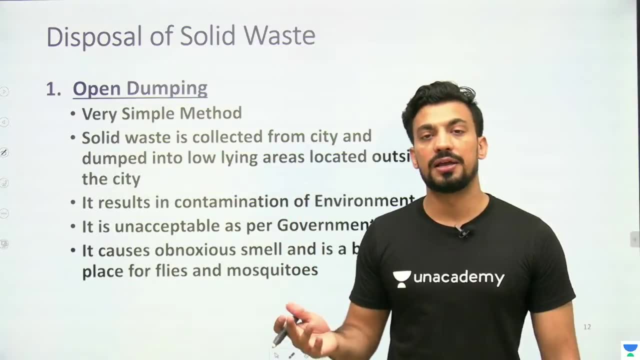 that's why we don't do it. There is a very bad smell. You also know, If you have ever been to a place where there is a lot of solid waste or your liquid waste is openly dumped, then it spoils the entire environment there. 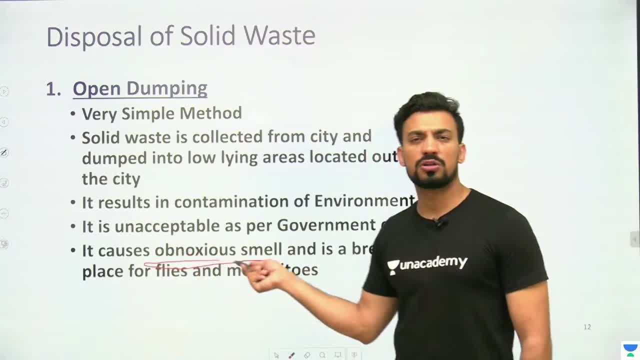 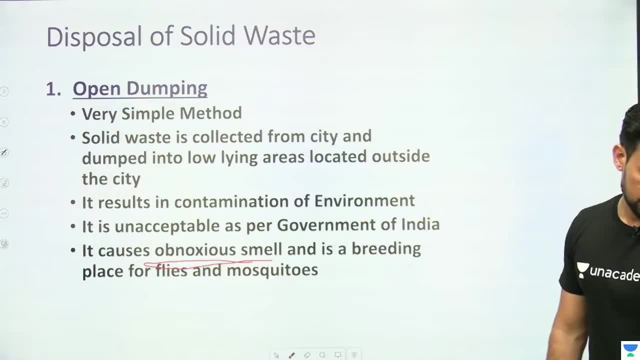 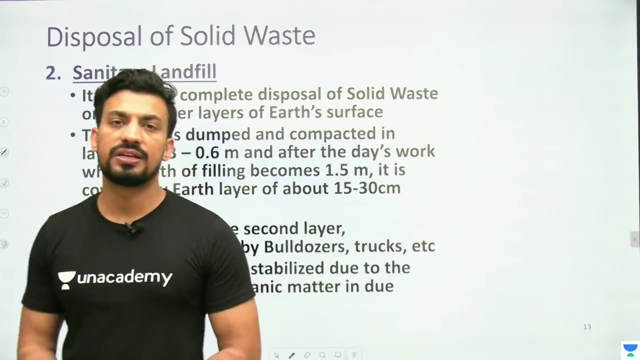 What happens to it? Obnoxious smell. Obnoxious means a very dirty smell that comes and is a breeding place for flies and mosquitoes. Flies and mosquitoes start growing there. After that, friends, comes sanitary landfilling. Sanitary landfilling means that you are there. 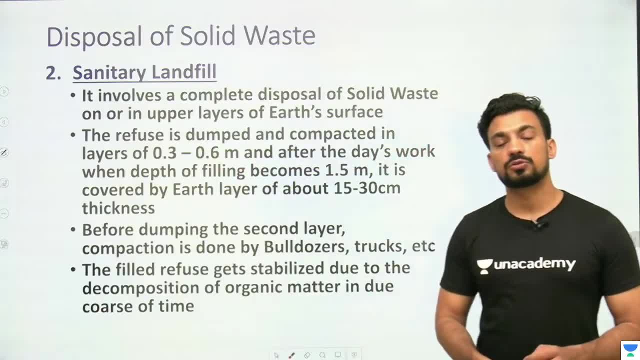 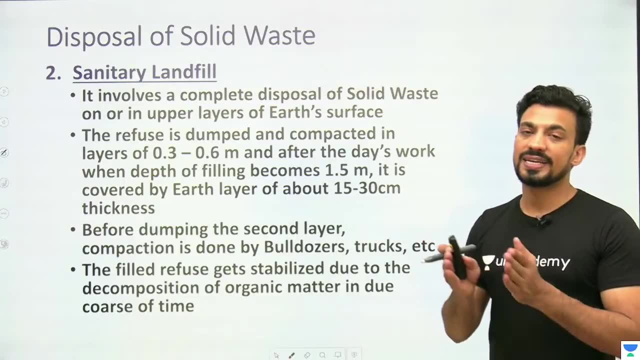 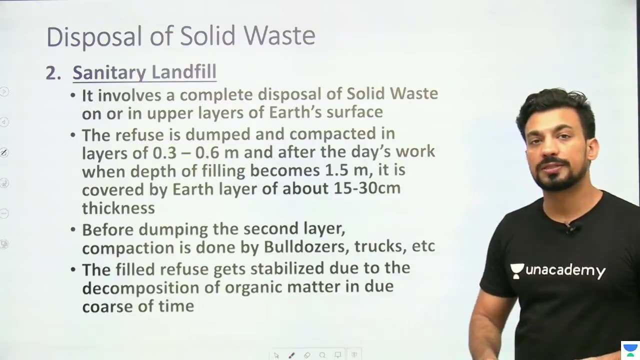 Then you cover it in soil. How do you cover it in the ground That you do whatever waste you have in compact? compact it in layers of 30 to 60 centimeters. compact it in layers of 30 to 60 centimeters and after that, when the depth of filling becomes, 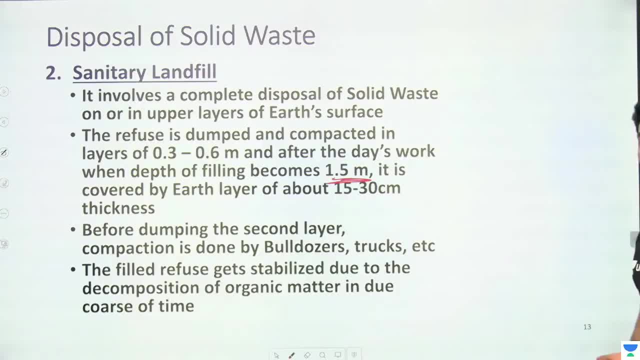 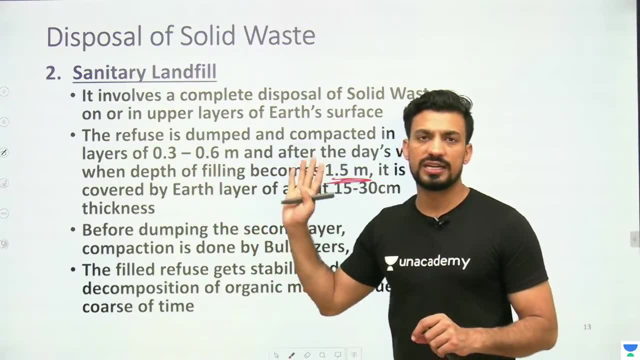 one point five meters. when the depth of filling becomes one point five meters, then apply the earth layer. Now what happened is that you are there, you can also apply the earth layer from the land. what happened is that you take 30 to 60 cm, 3 to 60 cm layers, keep making, compact it and one layer is made. then 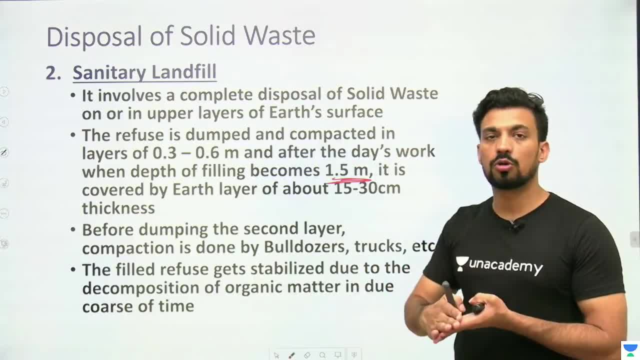 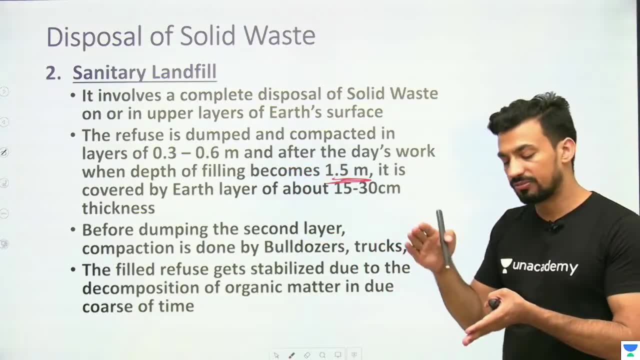 after that you put more waste. take another layer of 30 to 60 cm compact. it make it so compact here and when the thickness of 1.5 m overall, when the depth of filling is 1.5, then what do you do? cover it with soil. 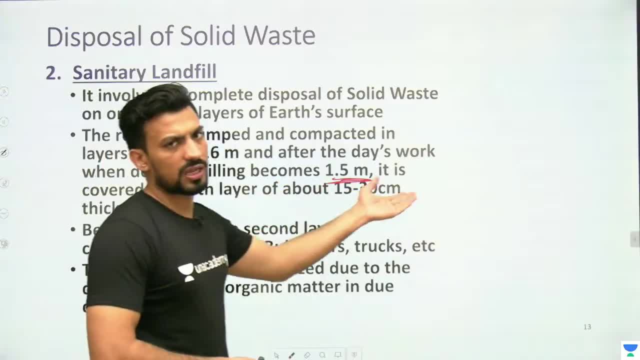 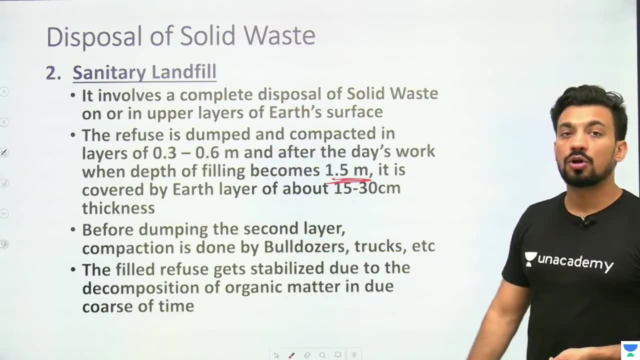 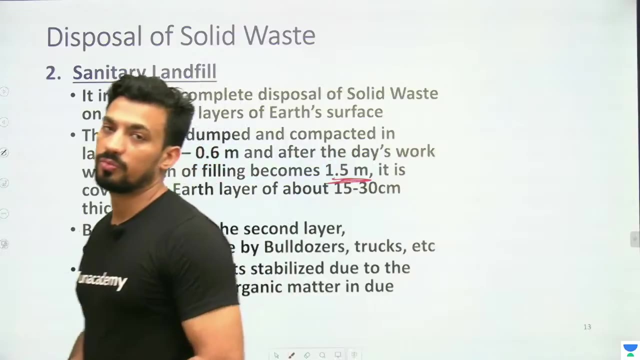 put a layer of 15 to 30 cm of soil and after that you keep repeating the process like this. before dumping the second layer, compaction is done by bulldozers, trucks, etc. After that, before putting the second layer, you compact the first one. 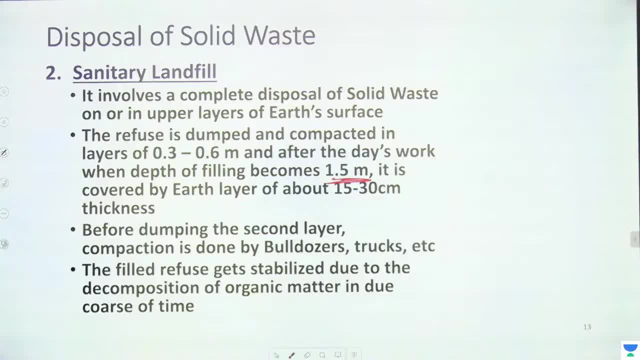 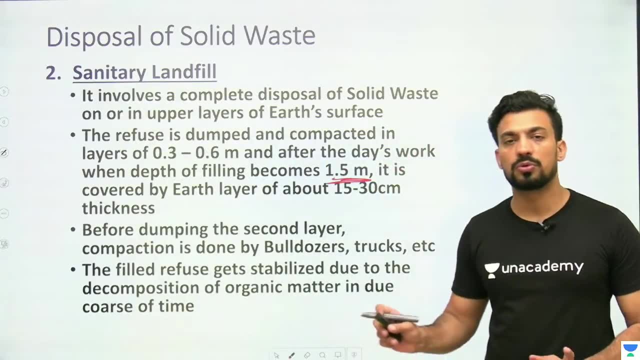 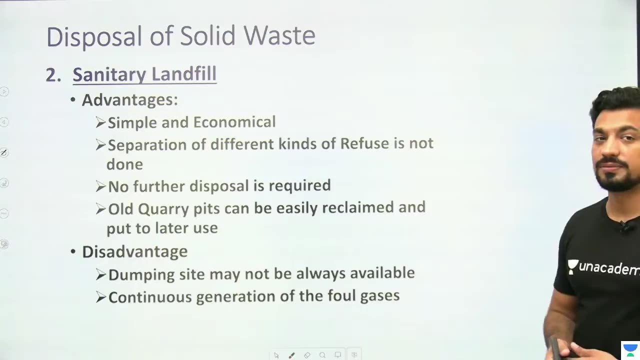 the field refuse gets stabilized due to decomposition of organic matter in due course of time. with respect to time, slowly, the waste will come to its end. You will decompose and settle there. Next, let's talk about the advantage. of advantage: no special treatment is done here. it is simple, it is economical and 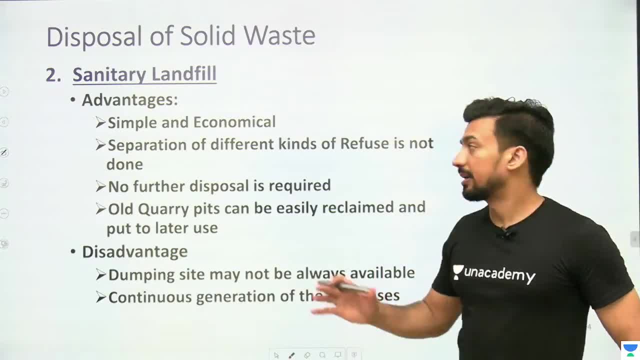 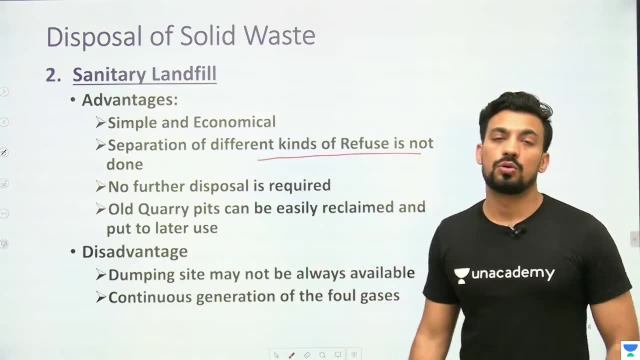 in this you do not have to separate the waste separately. separation of different kinds of refuse is not done. whatever, all the garbage is together, whatever it is, everything went inside it. so you put everything together now. after that you do not have to do any other disposal. after that it ends. 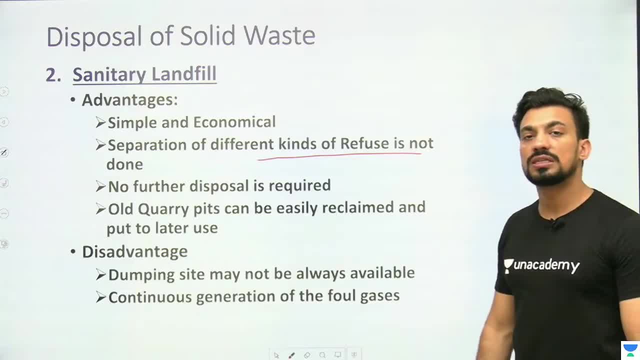 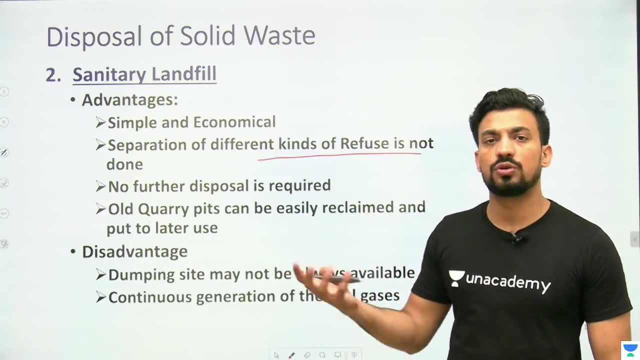 there is no problem. work is done there. old quarry pits from where you have taken out the stones. you have already taken out the stones from there, so that quarry has become a treasure. there are empty pits. there are big pits. fill them up, go there and put it. 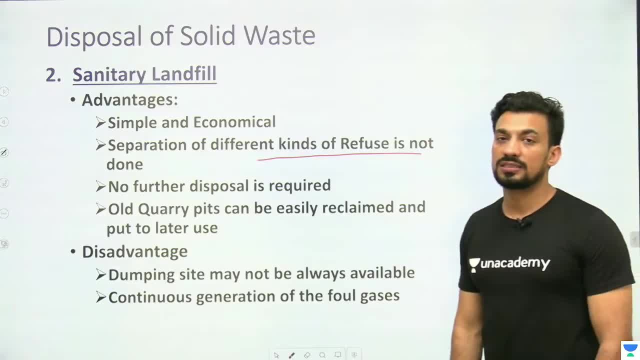 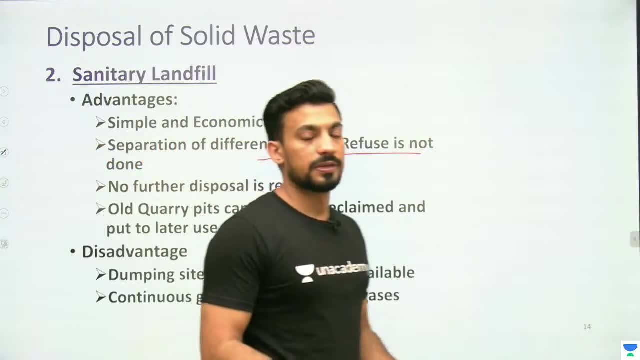 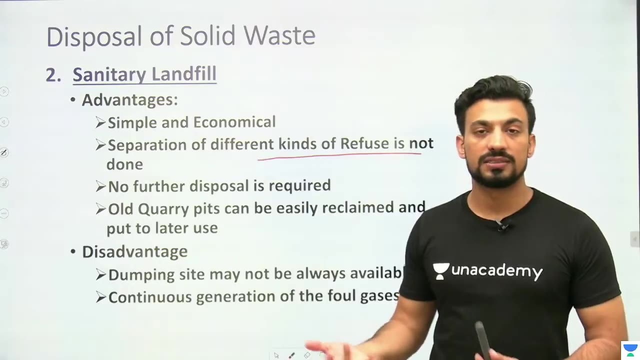 What is the disadvantage Dumping site? you know in today's time, if there is such a place, the most garbage will be generated in the cities. you also know this thing. if so much waste is being generated in the cities, if you have to decompose that waste or if you have to dump it, then you need space, and you know how much space is available. 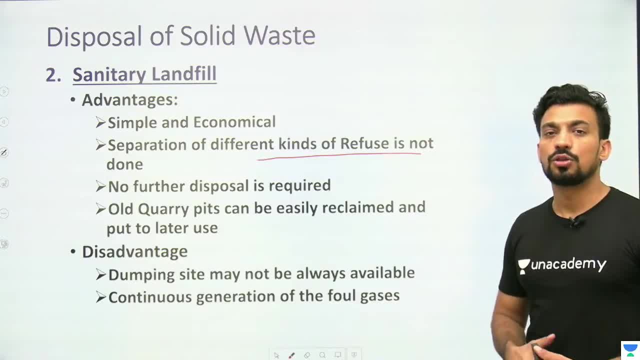 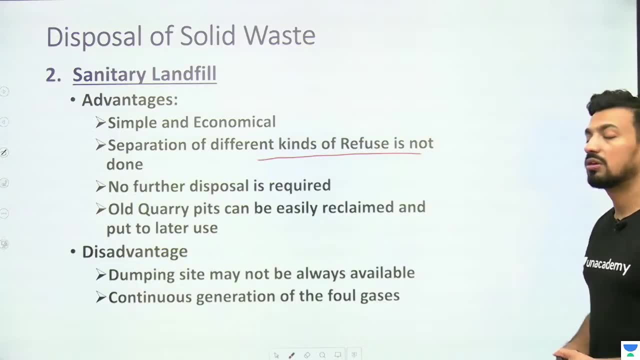 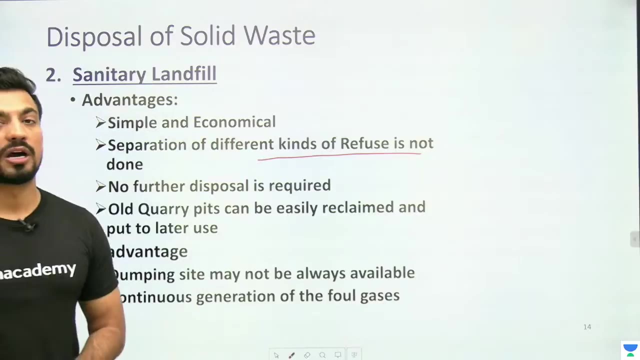 how much space is expensive. if we talk about cities, then it is not possible to find such sites specially for dumping- Continuous generation of foul gases. now, wherever we dump, some foul gases will come out of the pores of the soil and they can spoil the environment. 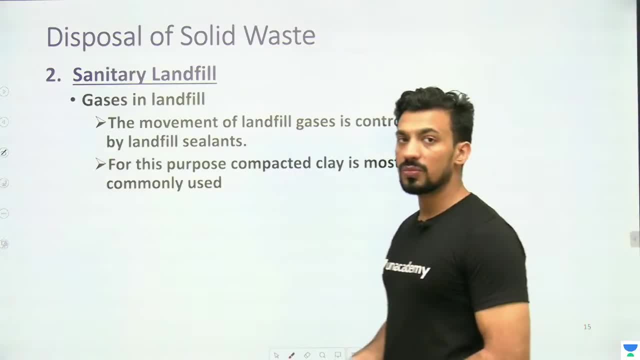 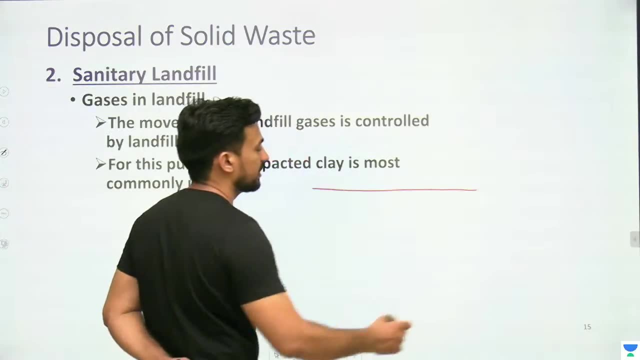 And what else can happen in it if it rains? if it rains, then water will go into the soil. water will go into the soil. this was the top layer. suppose here was soil. then down here you have put these different layers of waste. there are different layers of waste. 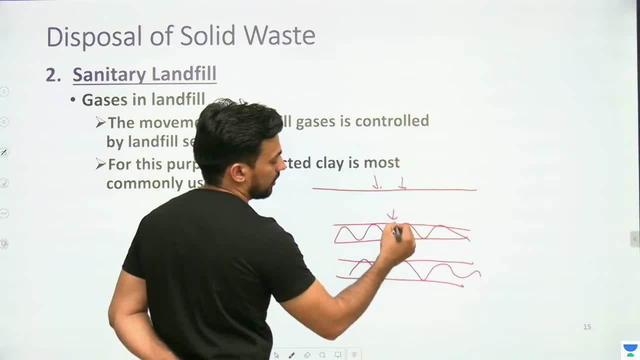 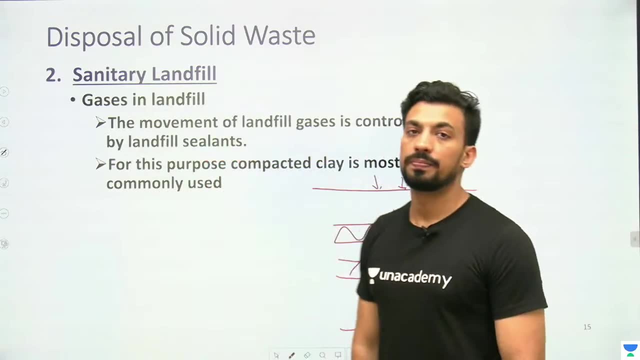 now when the water comes, the water will go down from here. then it will go down again. it will go down again. it will go to the ground water table. then it can spoil it there if the situation is such that if the ground water table is a little high, 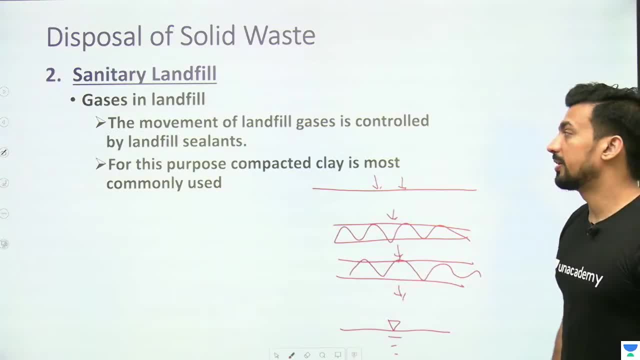 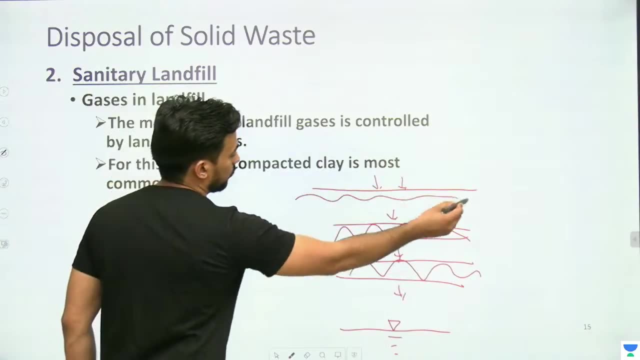 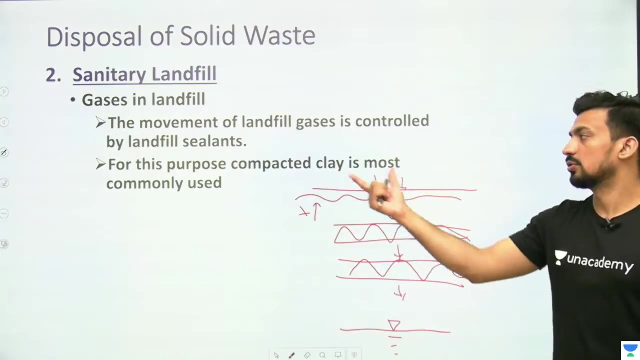 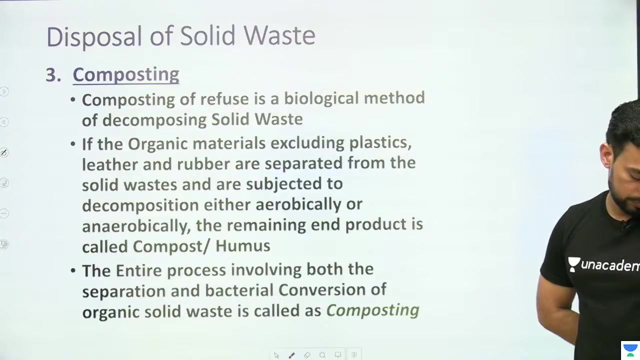 So how can you control the movement of gases? For the gas not to move upwards, add sealants so that the gases do not move, And you can use clay. Compacted clay is commonly used. Next, let's talk about composting. 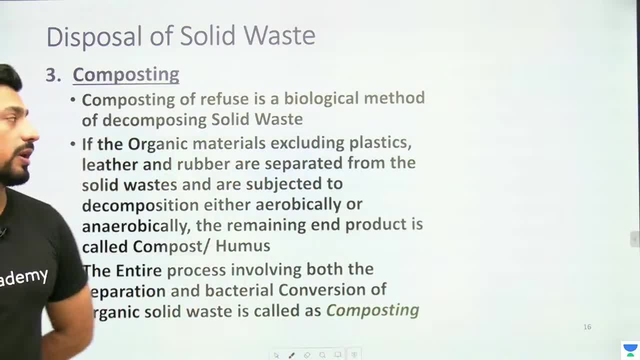 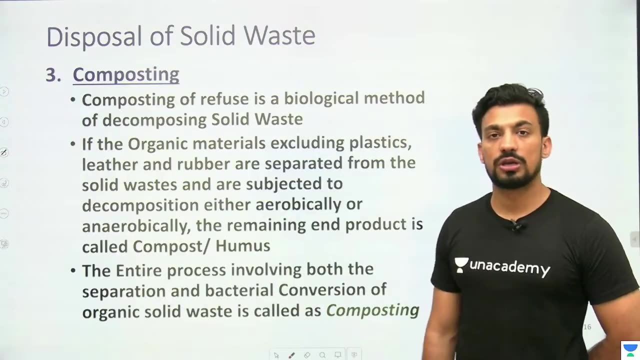 What is composting? Composting of refuse is a biological method of decomposing solid waste. What is composting of refuse? It is a biological method. Biological method means again we will talk about microorganisms which will come into the role If the organic materials, excluding plastic, leather and rubber, 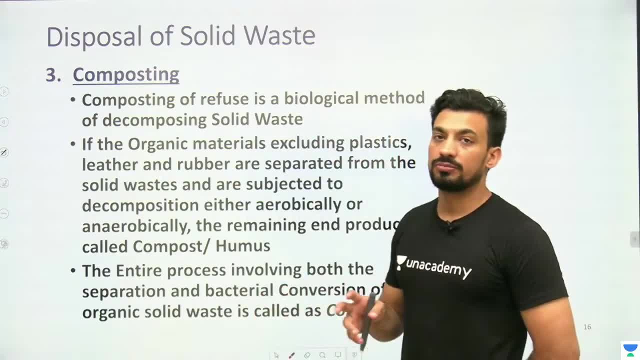 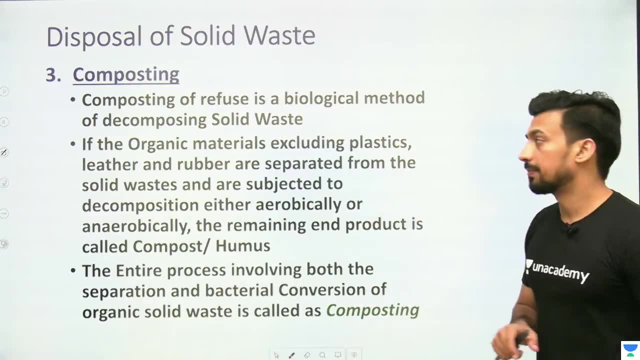 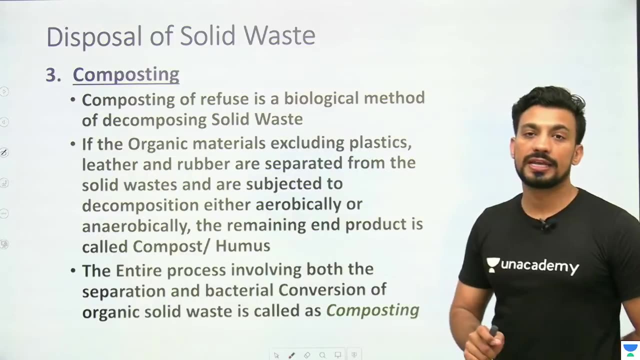 are separated from solid waste. From solid waste, you have to remove plastic, leather, rubber and these, And then the organic waste which is left. remove plastic, leather and rubber from all the organic materials. After removing these, what will you do? 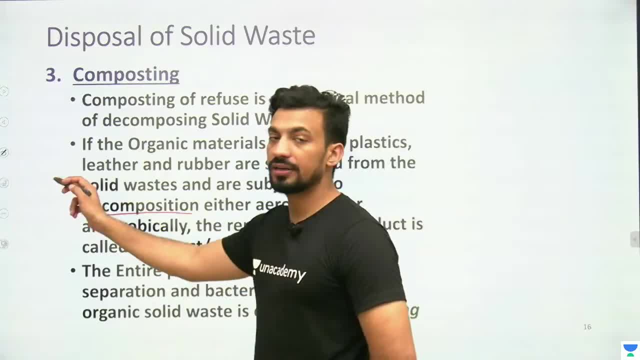 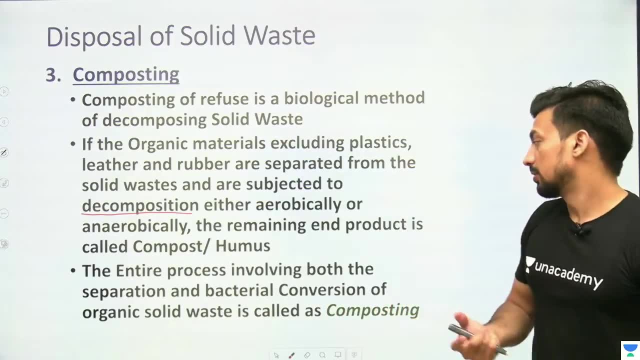 You will decompose the solid waste. You will decompose it Whether in the presence of oxygen or in the absence of oxygen. what will we do? We will decompose it And what you call the product that is made here, whether you call it compost or humus. 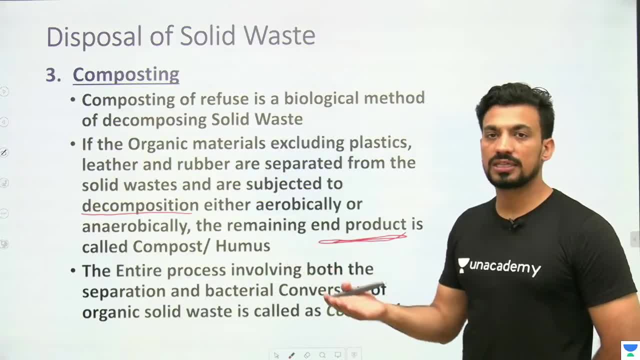 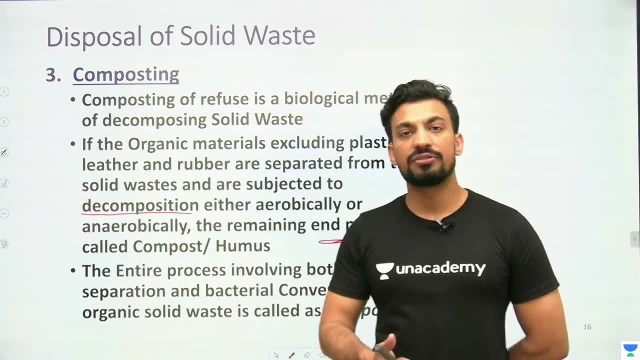 whatever you use, we talk about composting, it is used in agriculture. So what is that? Decomposed organic waste is there. Decomposed organic waste is there. Whether we talk about the waste of animals or cow dung, we make it using that. 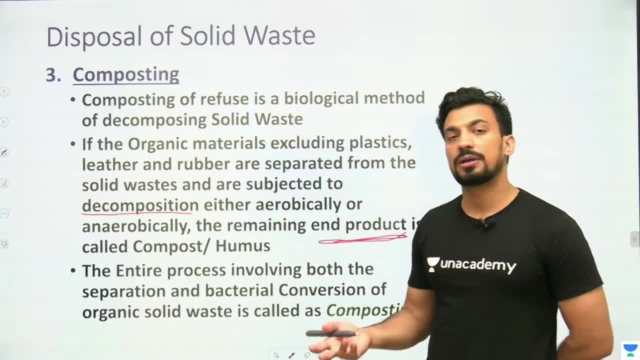 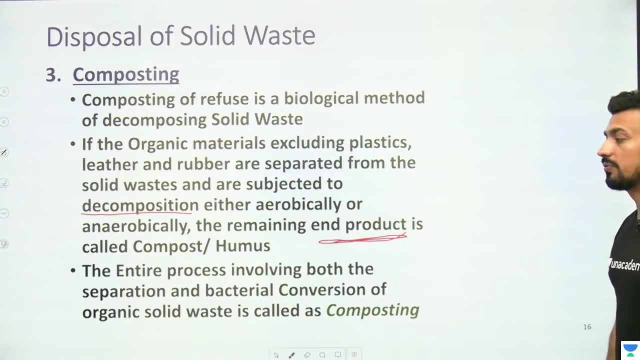 So what are you doing? We are decomposing the waste, And what are you making from that? You are making compost or humus. The entire process, involving both separation and bacterial conversion of organic solid waste, is known as composting. You have to remember one simple thing. 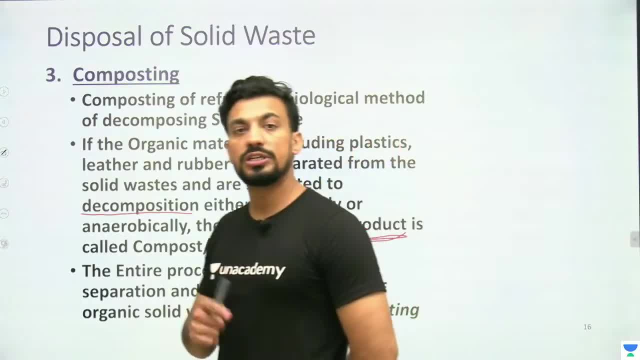 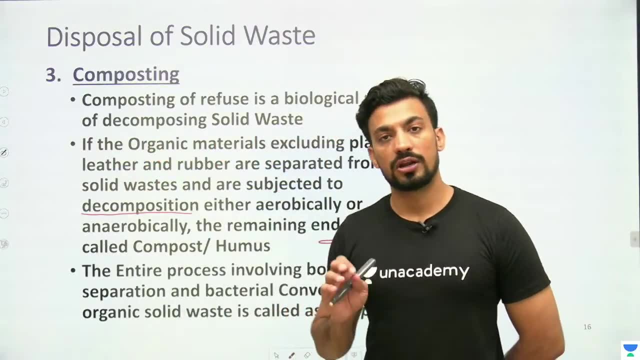 What is compost? Compost is decomposing organic waste. Organic waste means the dead and decayed matter of plants and animals, Any material organic waste. If we decompose organic waste, then we are getting compost here Now, in composting, 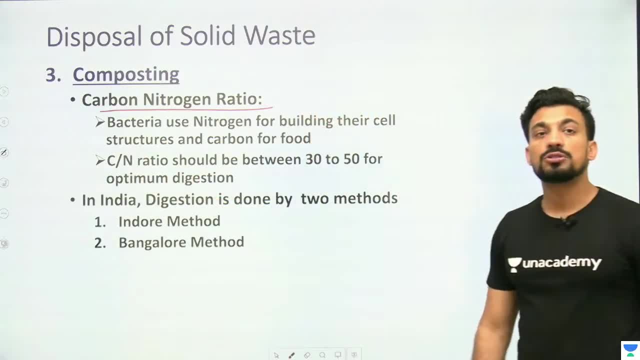 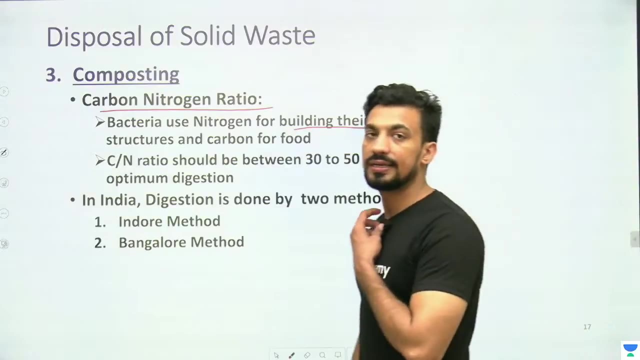 what is the use of carbon-nitrogen ratio? Bacteria that decomposes it. does bacteria need nitrogen there? For whom do we need? nitrogen For building their cell structure and carbon for food. Nitrogen for making the cell. carbon for food. 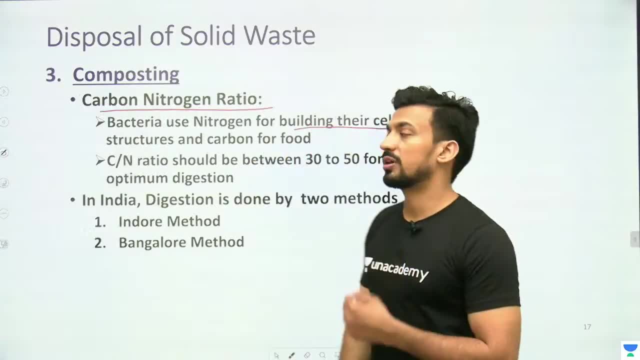 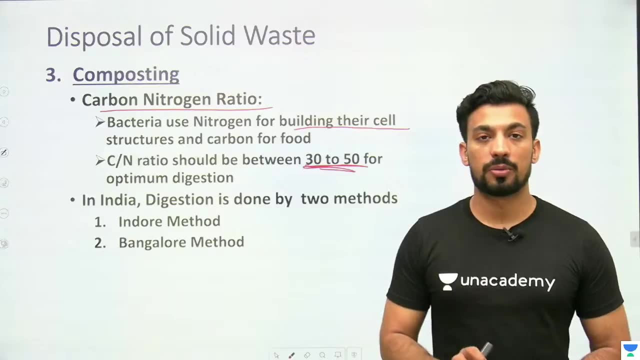 And this ratio of carbon-nitrogen. it should be between 30 to 50. It should be between 30 to 50. So that it can decompose that organic waste properly. Now it has two methods: In the presence of oxygen. 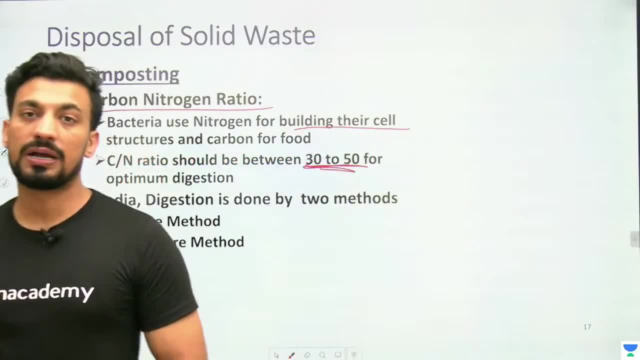 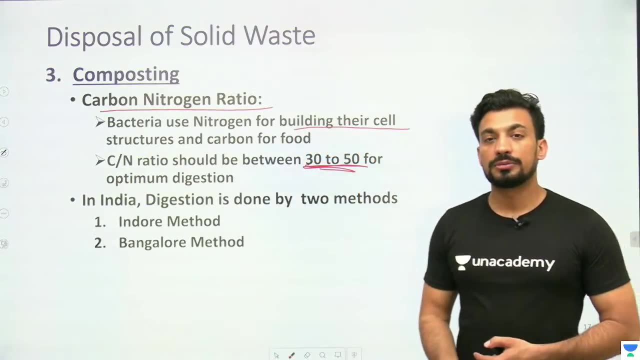 and in the absence of oxygen. There are two methods: in the presence of oxygen, that you are decomposing. in the absence of oxygen, One comes from Indore and the other comes from Bangalore. About Indore, it is said that Indore is a very clean city. 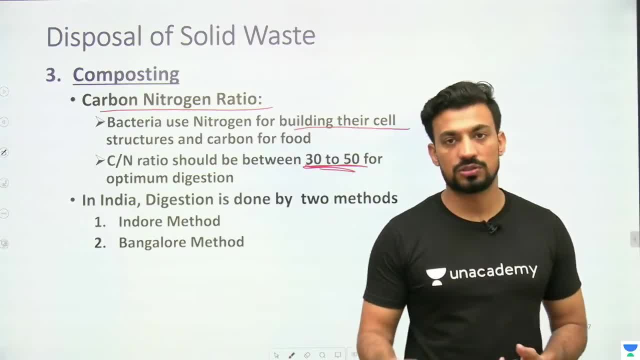 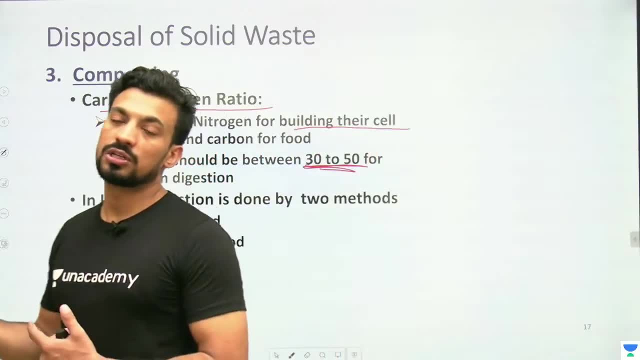 It is good. It is a clean city. It is a clean city. There will be good oxygen there, So oxygen came here. If we talk about Bangalore, then in Bangalore, Google Maps also tells you to get off the car, go on foot. 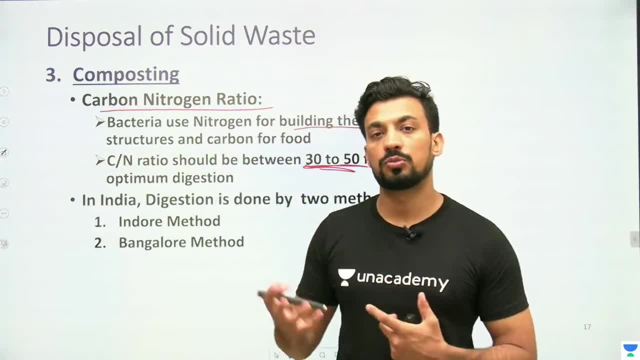 you will reach soon. So what is there? There is a lot of traffic. If there is traffic, then there is pollution. If there is pollution, then there will be very little oxygen there. So that's why, in the absence of oxygen, 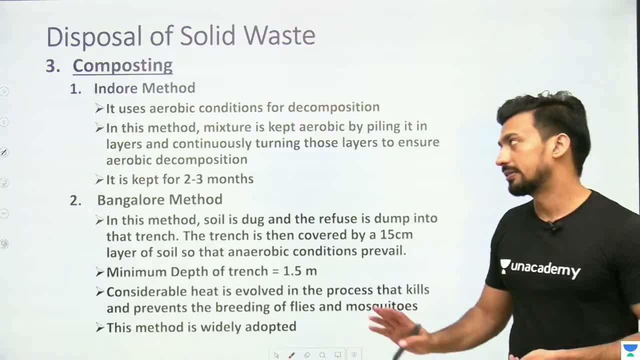 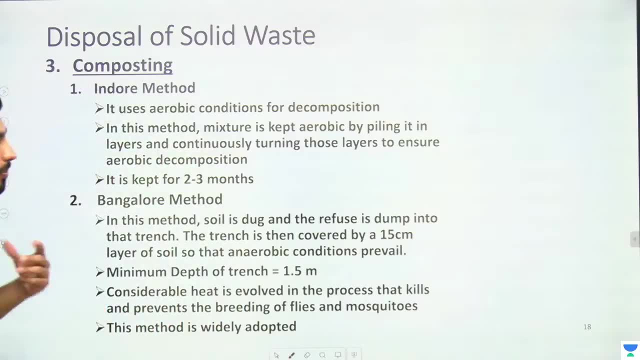 in the presence of oxygen. you get these two methods here. This is what it asks you in objective questions. What does it ask you in objective? It asks in objective that what is the method of composting? Or it will ask like this: 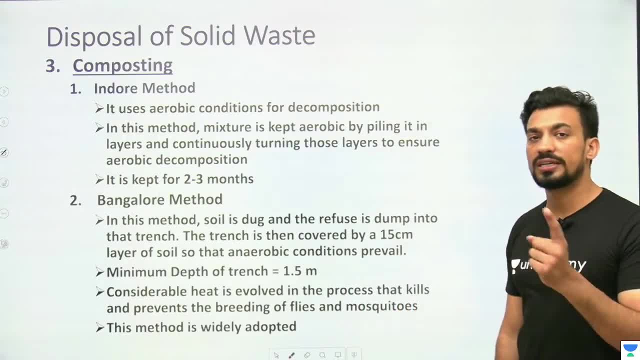 What is in the Indore method? Is it aerobic decomposition or is it anaerobic? So in the Indore method we get it decomposed in the presence of oxygen. There are aerobic conditions of decomposition And here, whatever your waste is, 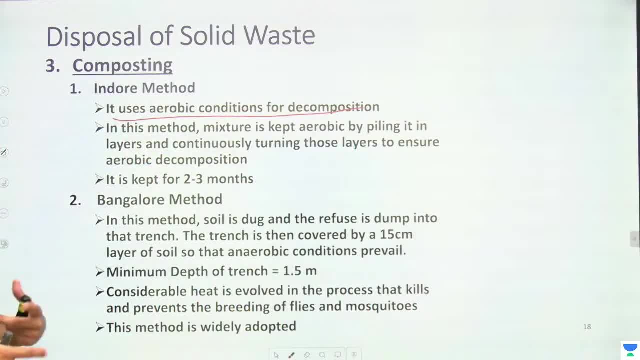 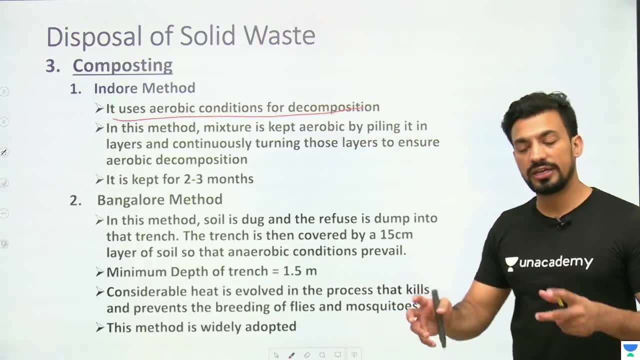 what do we do to that waste? We will do aerobic. We will keep rotating those layers. Whatever your waste is which is being decomposed, we will continuously turn those layers in it. We will keep rotating them so that we keep getting oxygen. 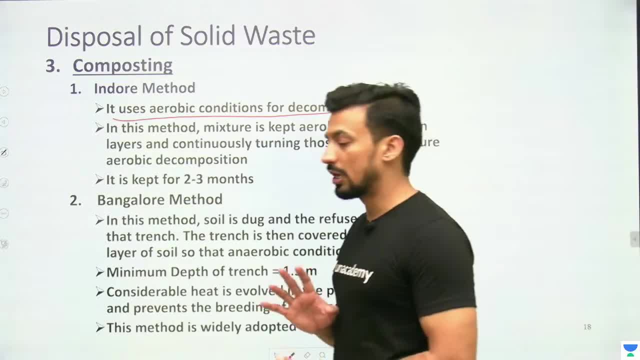 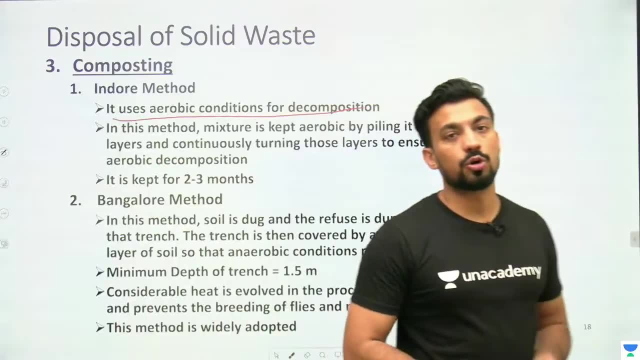 And whatever waste is being decomposed, it is in aerobic condition here And it takes about 2 to 3 months to decompose that waste. What do we do in the Bangalore method? We will dig a pit, We will put that waste in it. 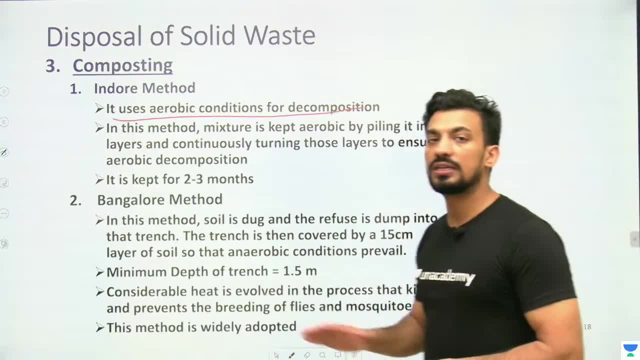 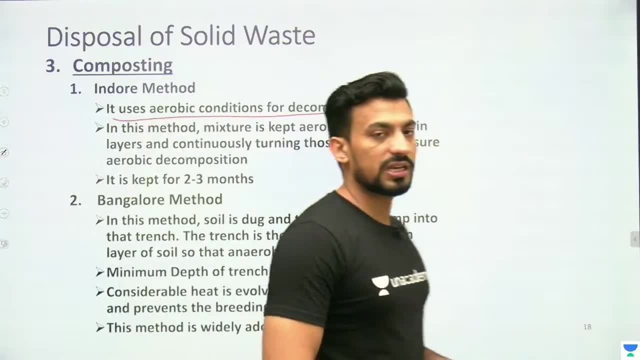 We will put it in that trench And we will cover it with a layer of soil, And in this way we will cover it so that it does not get oxygen there. When there is no oxygen, then in the absence of oxygen, that waste will decompose here. 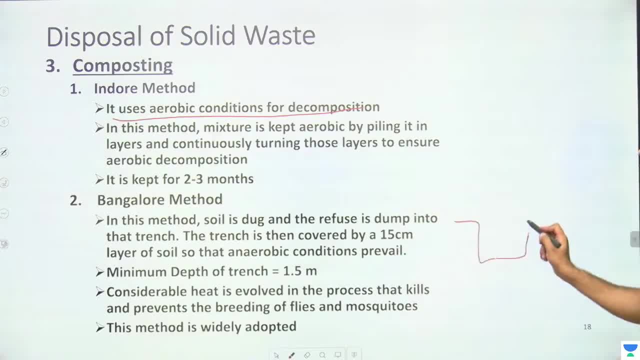 So in this method, soil is dug and refuse is dumped into the trench. Whatever the refuse or waste is, it is dumped. On top of that, a layer of soil is put back of 15 centimeters so that there are no aerobic conditions. 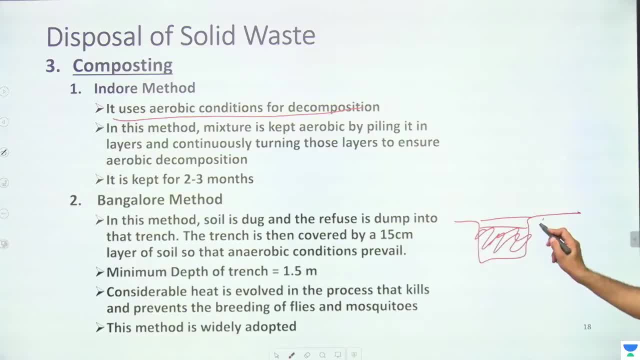 and oxygen does not go here. Minimum depth of trench: the minimum depth should be 1.5 meters. minimum Considerable heat is evolved in the process That kills and prevents the breeding of flies and mosquitoes. This method is widely adopted. Yes, thank you. 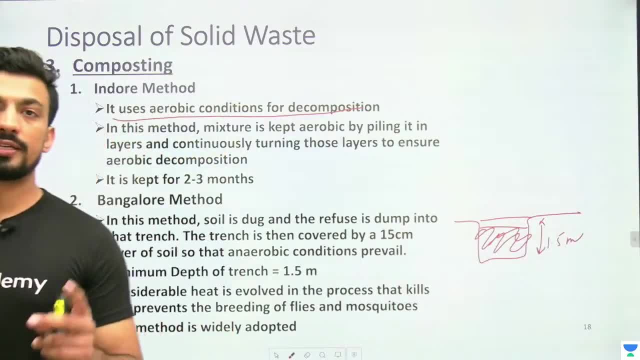 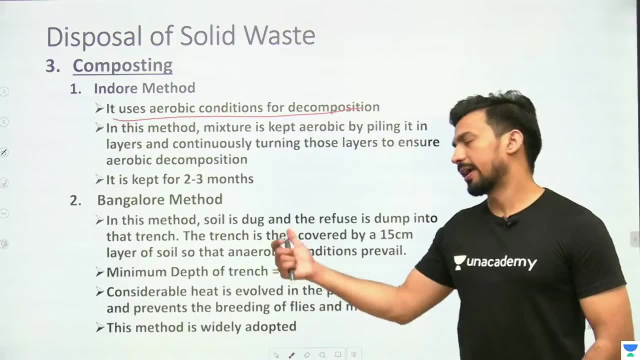 So you just have to remember this much: Two methods of composting in the presence of oxygen: In the presence of oxygen, aerobic is the Indore method. In the absence, anaerobic is our Bangalore method. After that, friends, what does pulverization mean? 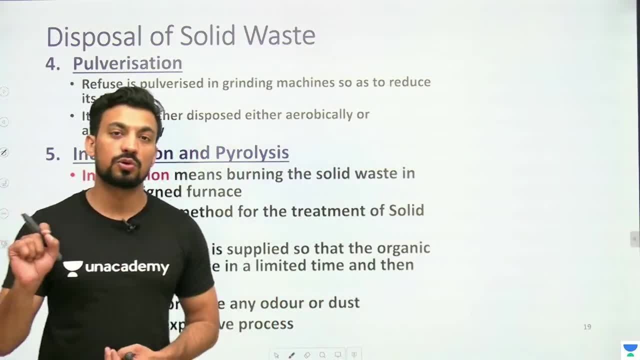 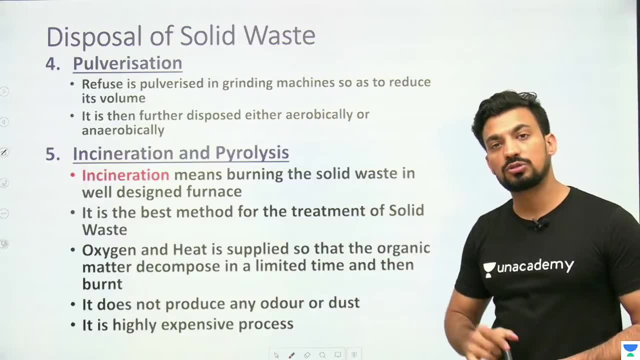 What does pulverization mean? What to do? To crush, to grind, to do it in very small pieces. So what does pulverize mean? What is its refuse in the grinding machine? What will we do in small pieces? We will divide it into small pieces. 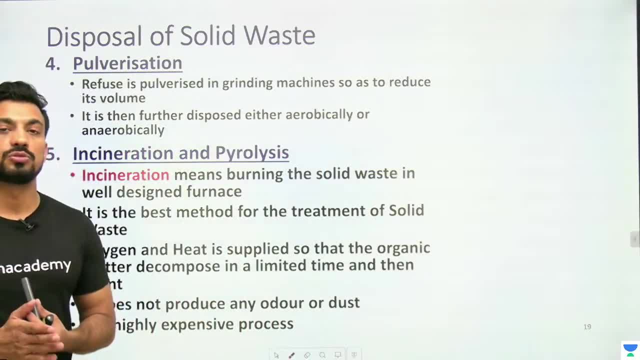 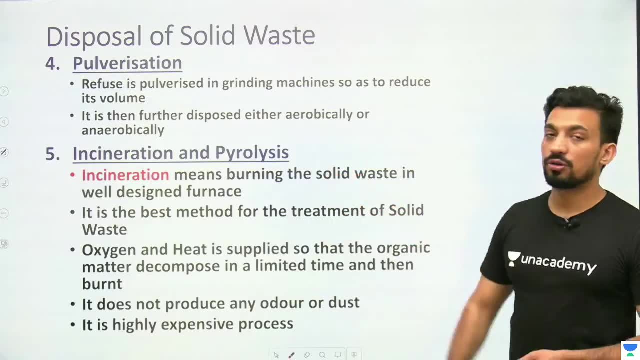 Why will we do it? So that its overall volume is reduced. Then, after that, we will decompose it, whether in the presence of oxygen or in the absence of oxygen. What is incineration and pyrolysis? What does incineration mean? 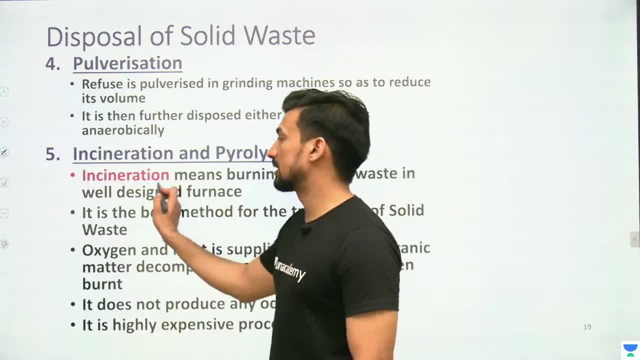 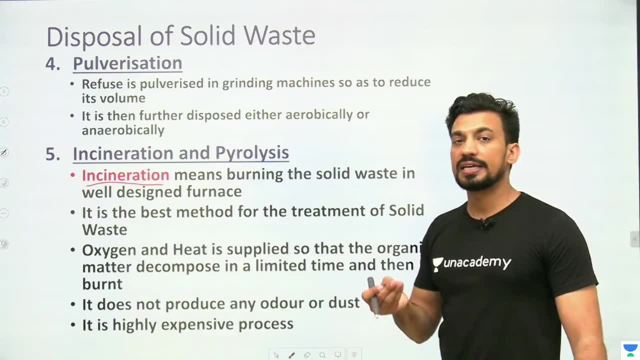 Incineration means that you are incinerating it. Incineration means that you are burning it. What are you doing? You are burning the waste. Now you have two ways to burn it. What will happen is you have something, just you, directly. 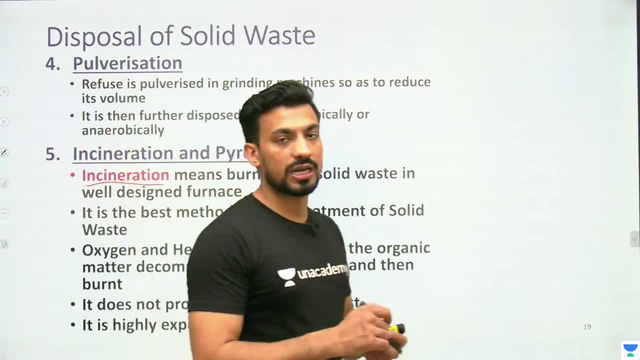 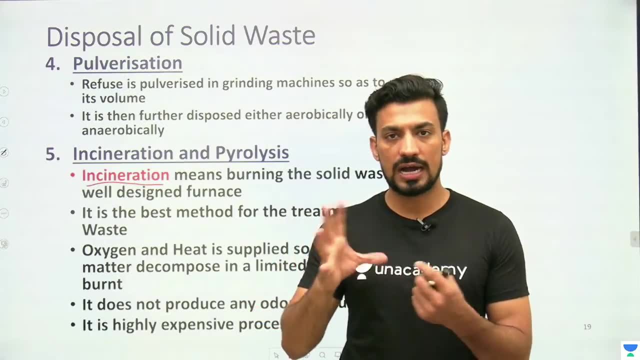 set it on fire, Like paper. What will you do with paper If you set it on fire or you do it with a matchstick light? it burn it. When you burn it, it will produce heat. The fire will burn. 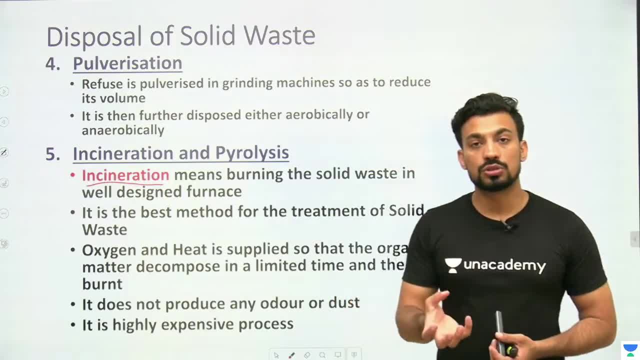 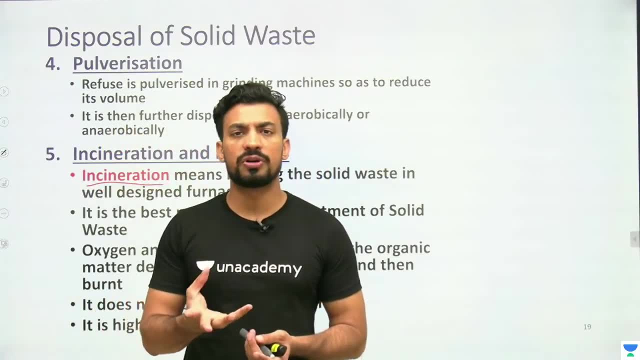 Heat will be produced from there. This is one thing. Secondly, what happened? As we talk about wood or we talk about making tar, then what do we do? Keep providing it with heat. Provide so much heat. Don't give it fire directly. 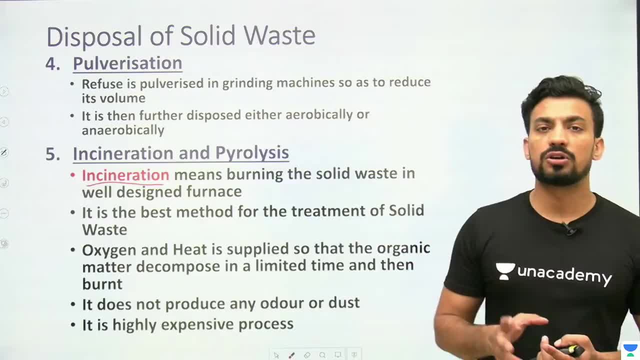 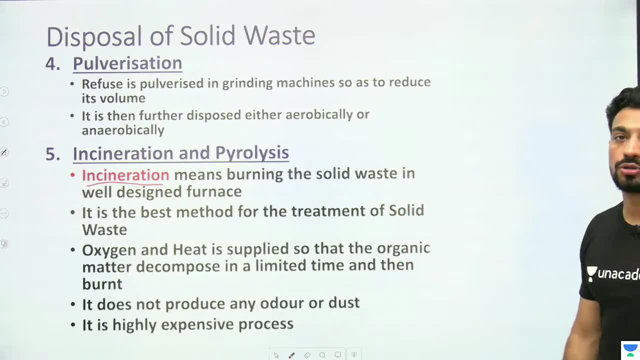 Don't give it fire. We are providing it with heat so that it can be converted into tar later. So, in the same way, here is incineration and pyrolysis. So what do we do in this? We are burning solid waste. 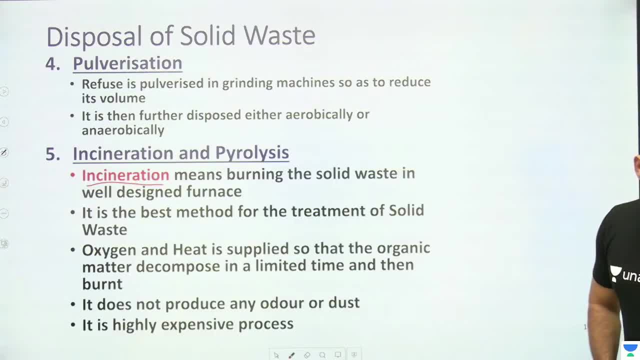 What are we doing in incineration? We are burning it. It is the best method for treatment of solid waste. Oxygen and heat is supplied so that the organic matter decomposes in a limited time and then burnt Now, because you have organic waste here. 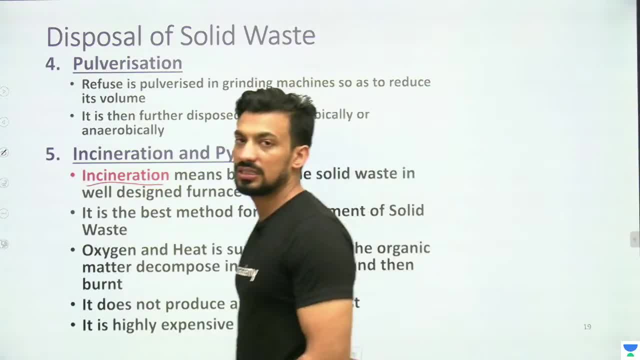 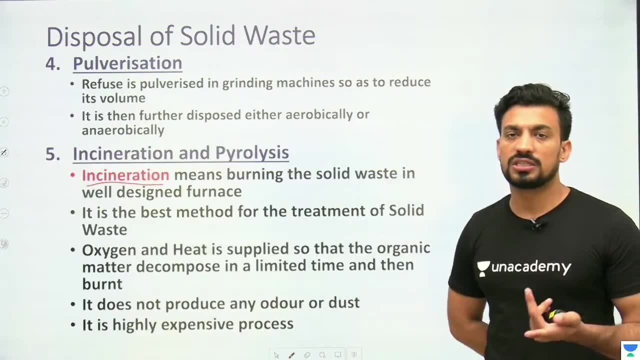 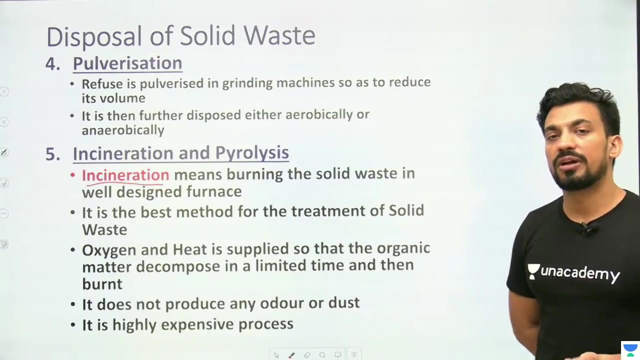 Now, organic waste is not like inorganic materials. If organic waste is not burnt so fast, the rest of your fuels are burnt as soon as possible. So organic waste is burnt as fast and it will not burn. What will we provide for that? 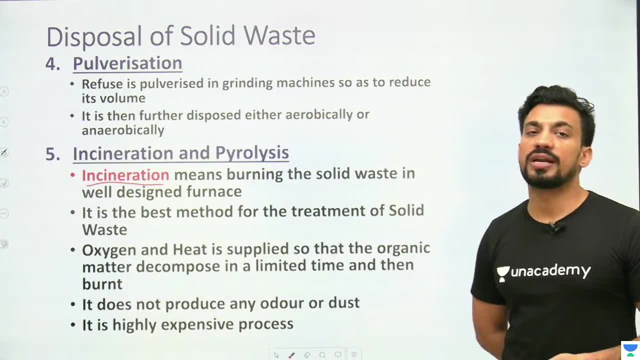 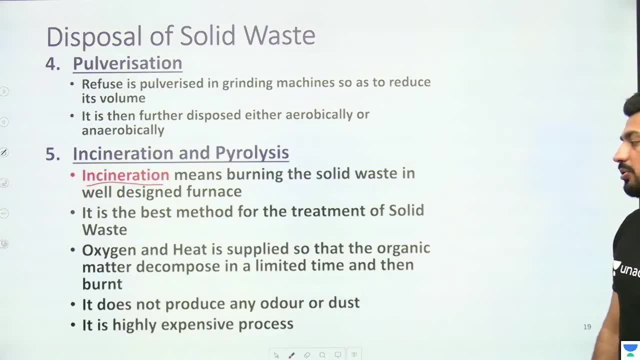 We will provide oxygen and we are providing heat ourselves. We are providing it here, So it does not produce any odor or dust. It will not smell by burning it Or no dust will be produced. But it is an expensive process. You are burning it yourself. 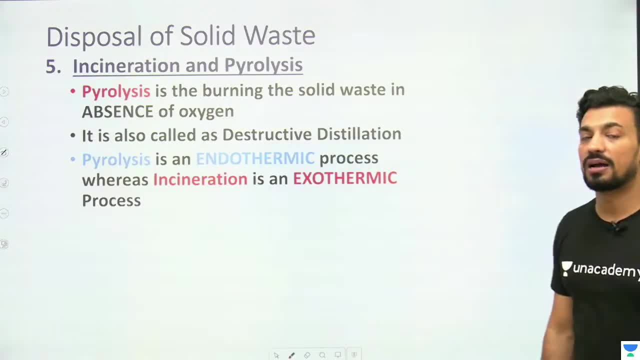 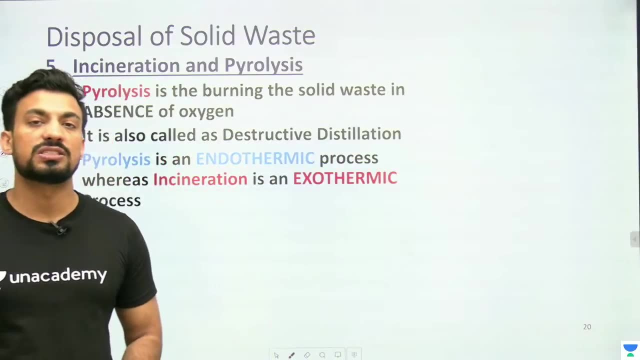 in incineration, You are providing oxygen and heat yourself. If you talk about pyrolysis, then what are you doing? in pyrolysis, You are burning it in the absence of oxygen Or, as we do, distillation, destructive distillation. 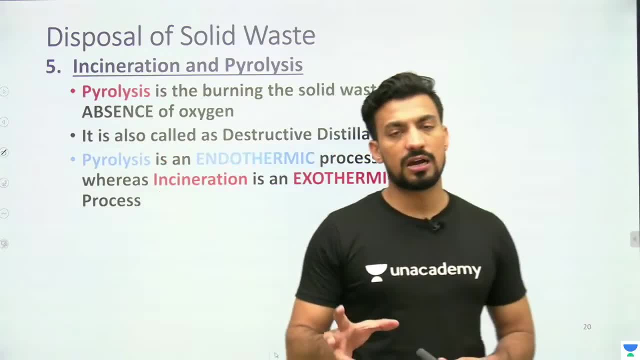 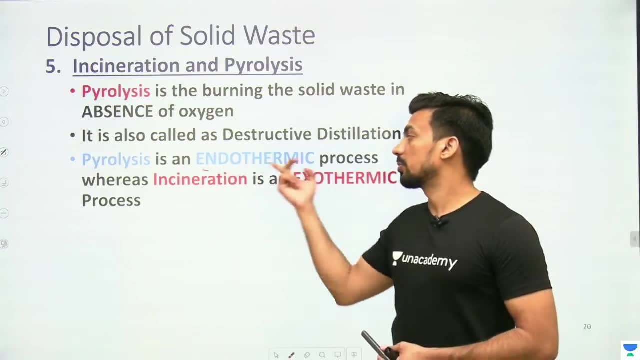 of wood. We have studied in childhood. So we are doing the same thing here. We are heating it in the absence of oxygen, We are giving it temperature. So what are we doing? in pyrolysis, It is an endothermic process. 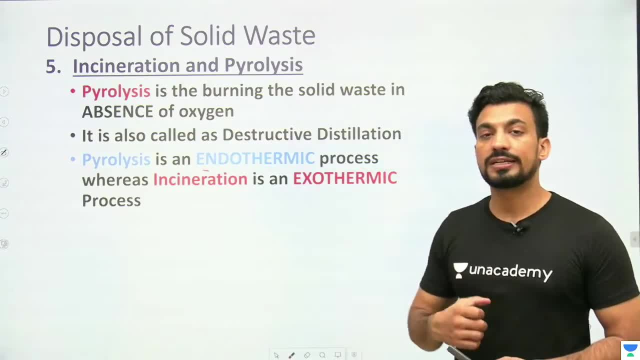 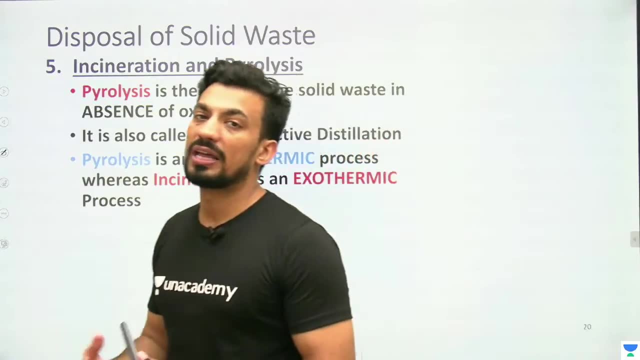 What are we doing in pyrolysis? It is endothermic, That is, it is absorbing energy, You are providing it- Whereas incineration is exothermic. If anything will burn in incineration, then it will release energy later here. 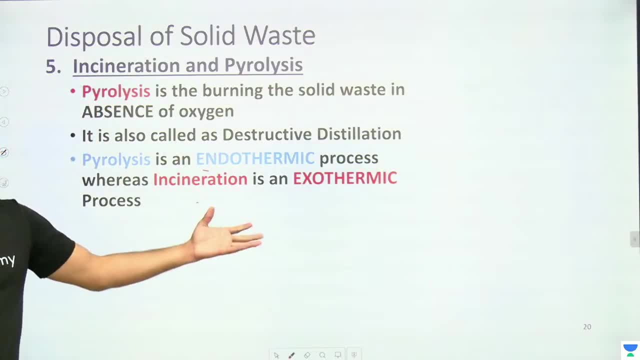 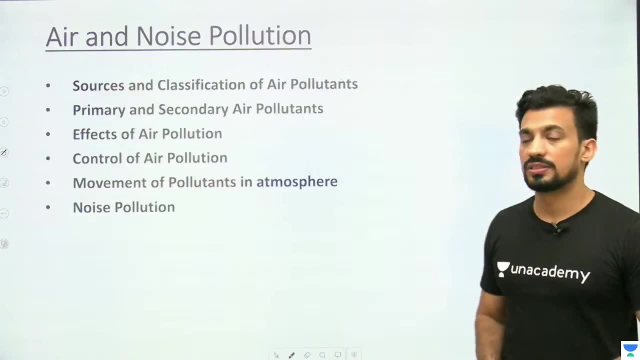 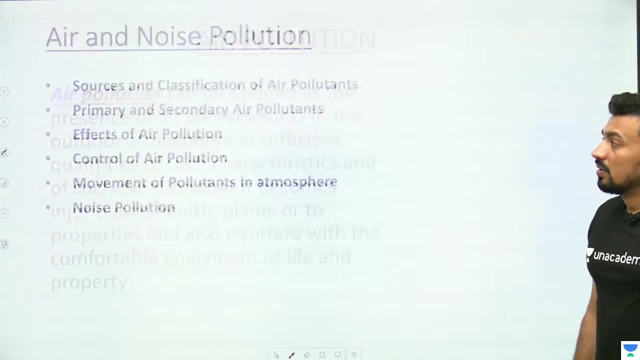 So your incineration is exothermic because it will provide energy by burning, And pyrolysis is endothermic. This is the basic difference between them. Let's talk about air and noise pollution. Let's come to air pollution. 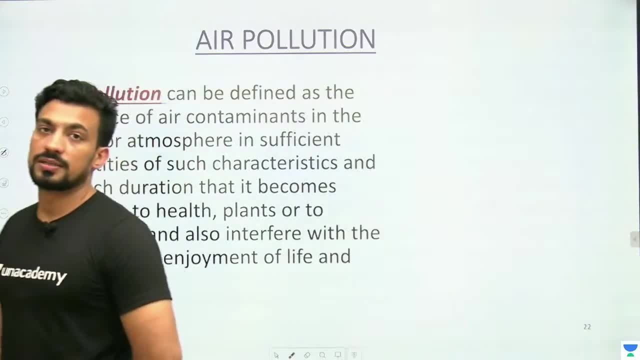 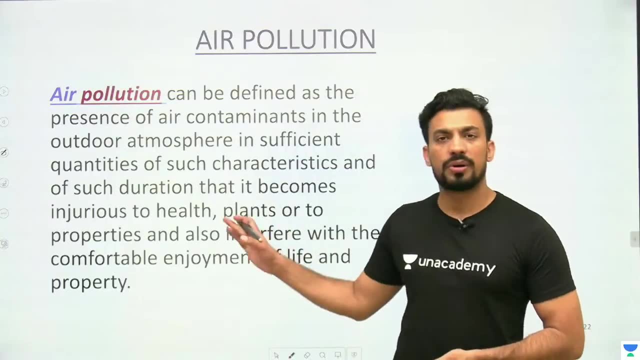 Let's finish the environment. Let's talk about air pollution. What is air pollution? Any unwanted substance in the air is air pollution. There is no special meaning to read all the other stories. You know what happens with air pollution. There will be a problem. in breathing with air pollution. We need the oxygen in the air, But we will not get that much oxygen. All the other gases will also go, Due to which the lungs will be damaged. The lungs will be damaged. Oxygen will not go properly. 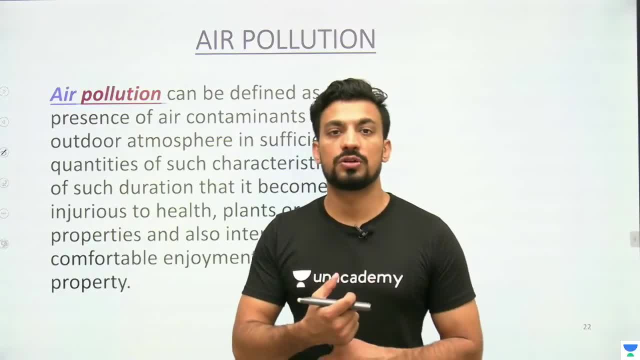 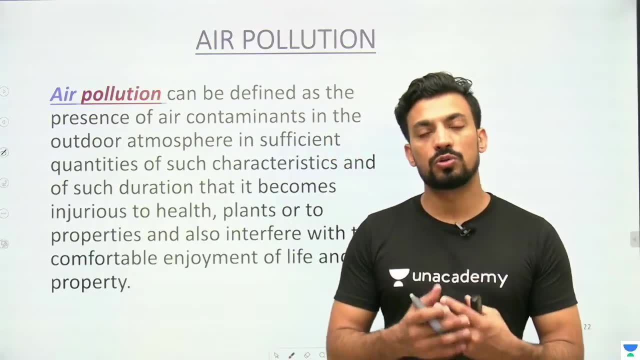 in the body, Lungs will not work properly, The body will not get oxygen properly, Oxygen will not get. So all the work is slowly, our digestion system, our body's overall growth, the cell that has to be made Because in our body it is not like that a cell is made, once New cells are made, The old ones keep getting dead, So this process keeps going on overall. That's why our body changes so much. From every year to next year, we are seeing so many changes. 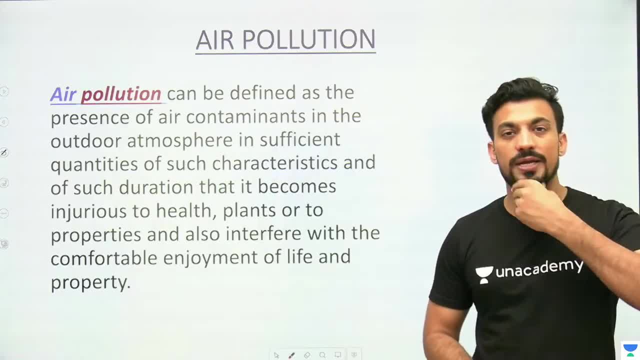 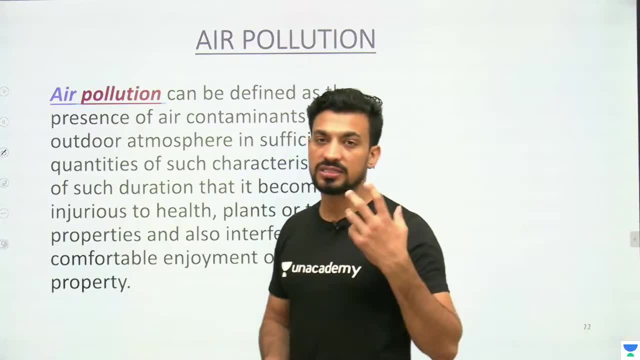 Why are they coming Because of all these reasons So slowly? the whole overall will impact our body. If you are looking, there will be no clarity in the air, It will not look good, The eyes will start burning, Irritation will start in the skin. 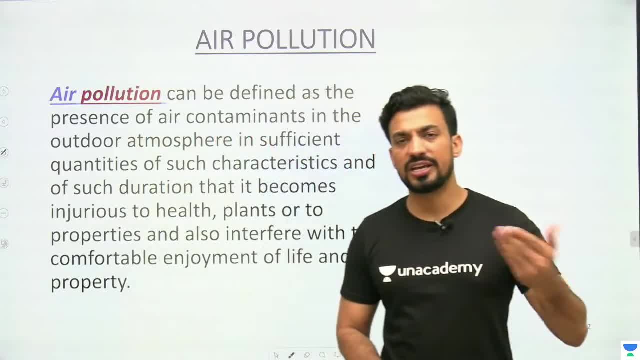 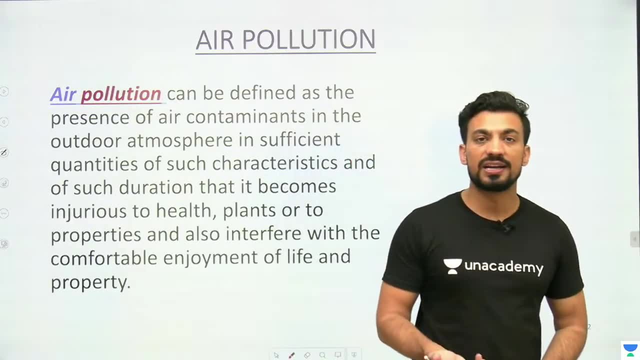 It will start, If you assume, as soon as the contact of air is coming with you. it will start harming you in all ways. If there is a lot of gases present in the air, they will create acid rain there, So all these issues will happen. 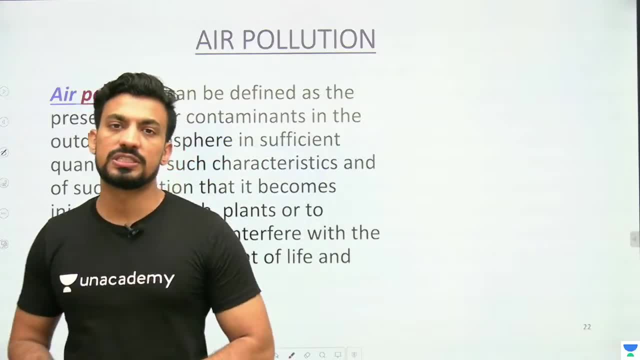 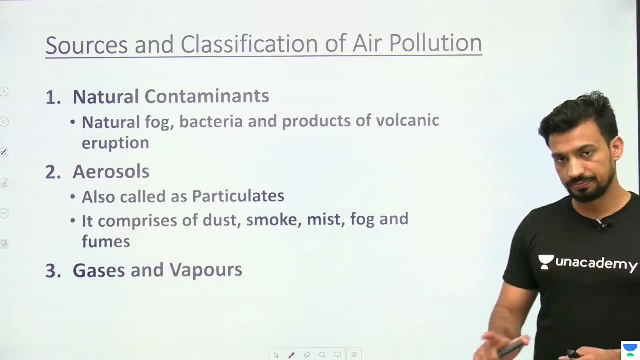 Now, either humans, animals, plants, vegetation will start harming everyone. Now, what can be the sources of air pollution? What is the source, What is classification? If we talk about the source, then in the sources, it can be natural, It can be natural. 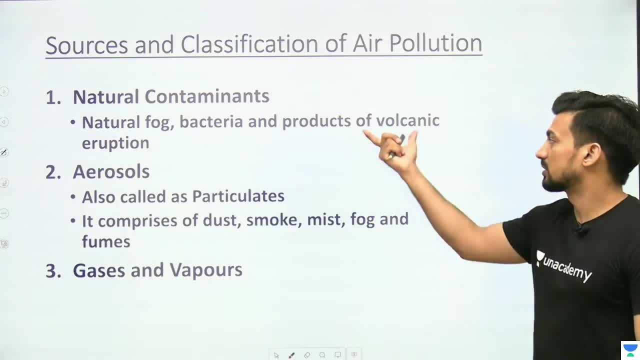 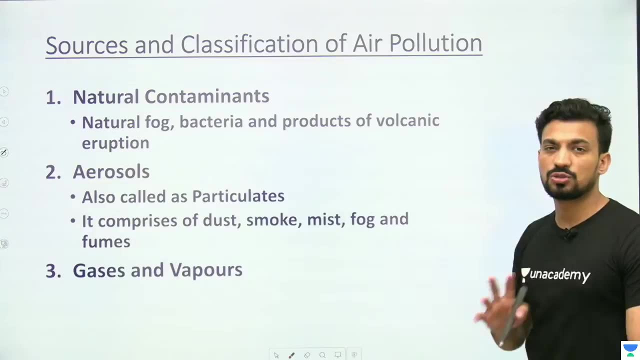 contaminants. What will come inside? It can be fog, It can be bacteria. Volcanic eruption: If the volcano erupts somewhere, then due to that, the dust there or the particles or gases there, due to them, the environment will be polluted. 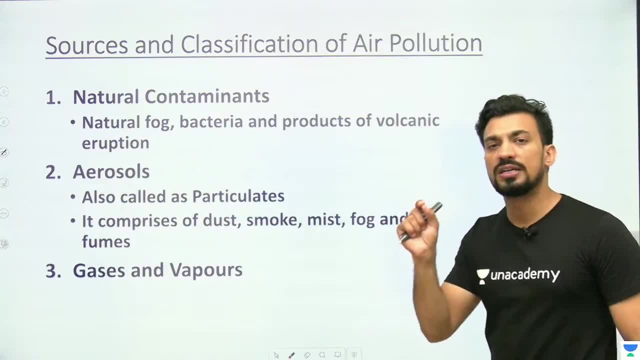 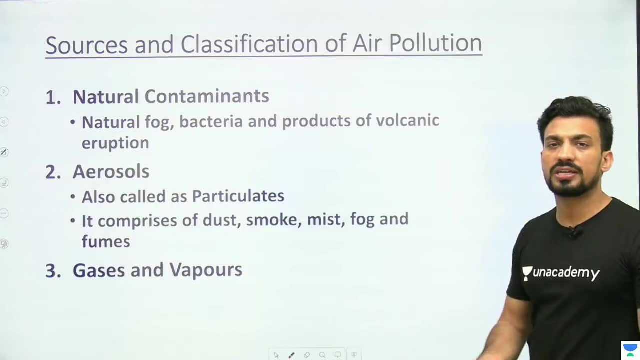 Aerosols means very small particles, Very small particles like dust, if you see, you have cleaned your room very well After a while. if you see above your table, above your books, above your laptop, above your phone, you will see very small particles. What will that be? 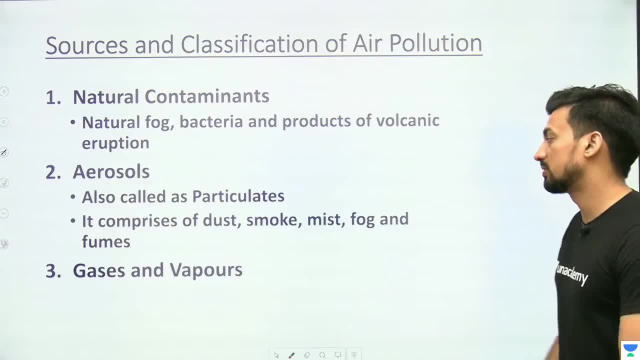 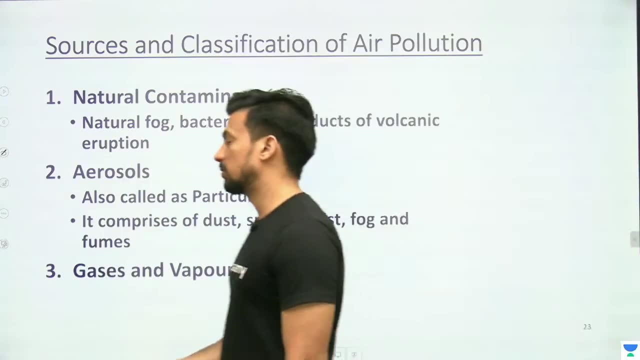 It will be dust or that particulate matter will be present. Apart from this, dust, smoke, mist, fog or fumes that come your voice, Fumes are very fine particles that you will see in the liquid If we talk about gases. 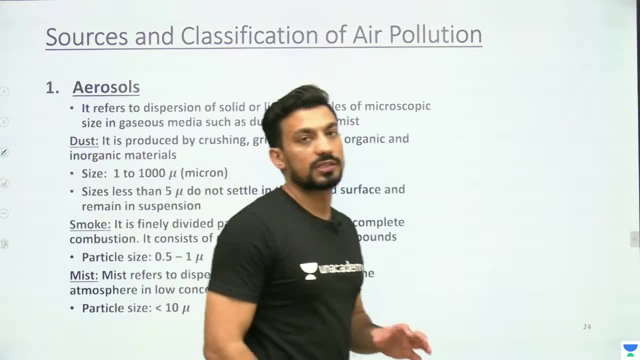 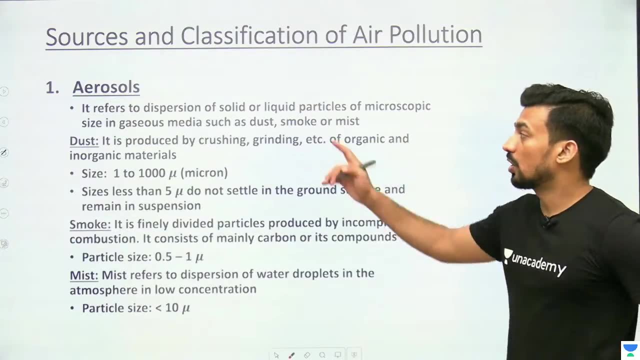 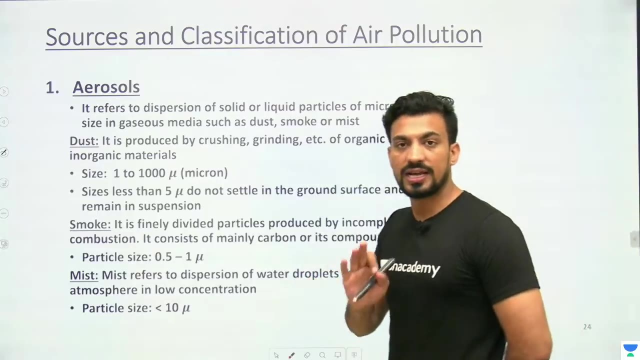 then gases and vapors due to them. it can happen. If we classify aerosols further and further in detail, then what happens in aerosols? So aerosol means particles of solid or liquid which are very small in size. Aerosol means like dust, so dust is solid. 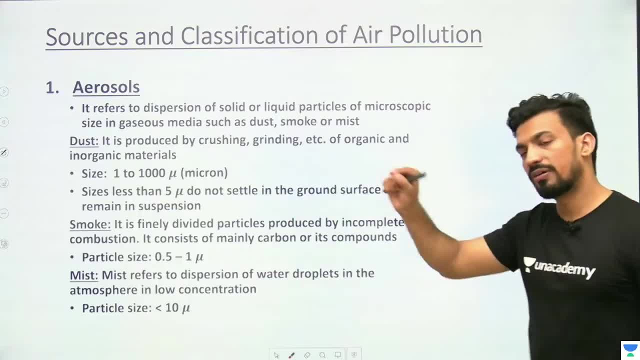 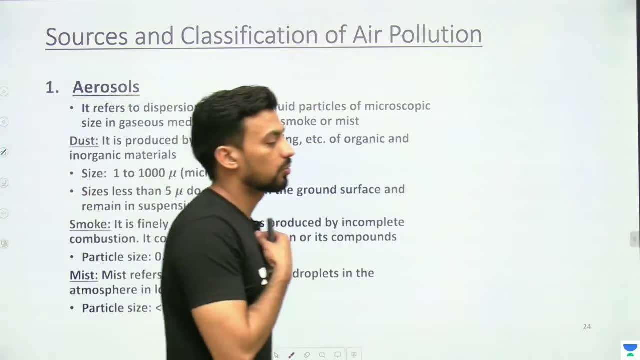 but particles are very small, so small that it is rotating in the air. it is rotating here. So, whether it is particles of solid or particles of liquid, then what do we call it? It is called aerosol. Like, suppose, if you use deodorant. 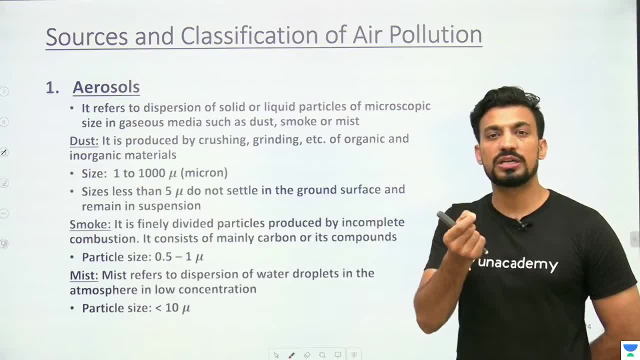 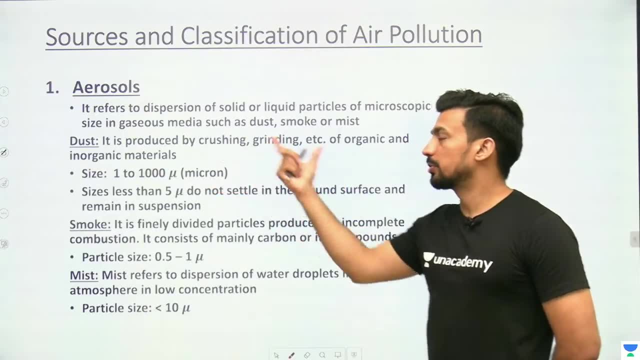 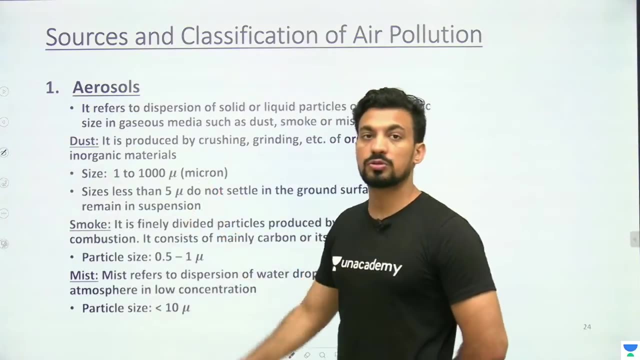 then what is the particle coming out of it? There are small particles of liquid. and what are the particles of liquid? It is aerosol, in a way. So dust is produced by crushing and grinding of organic and inorganic material. Its size is between: 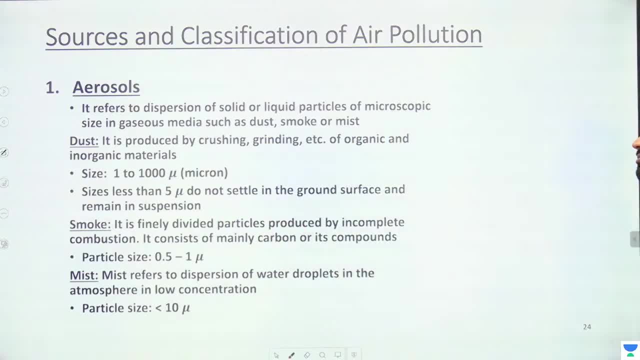 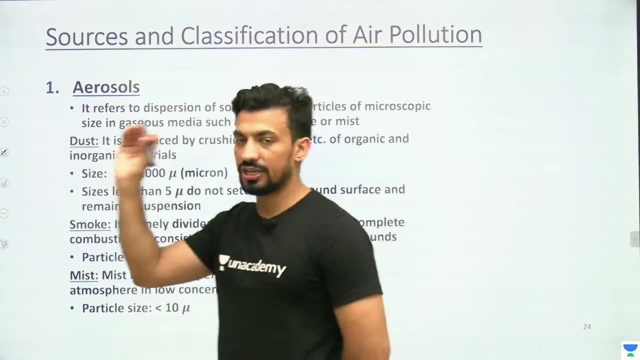 1 to 1000 microns. 5 microns, which is size less than 5 microns, do not settle in the ground surface and remain in suspension. So whenever you are sitting in a room and you see particles of liquid in the air, 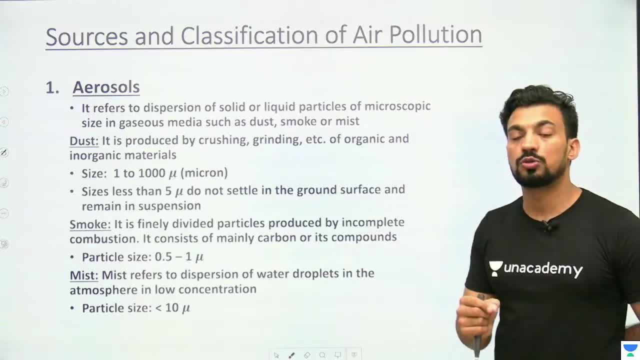 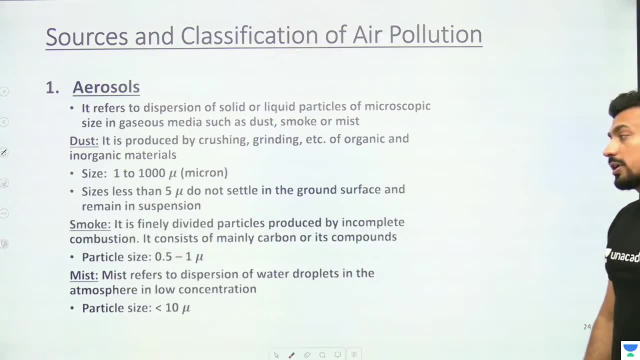 then what are those particles? They are aerosols. It is dust which is smaller than 5 microns. That is why those particles are not settling on the ground. Very small particles. If we talk about smoke, then what will happen to smoke? 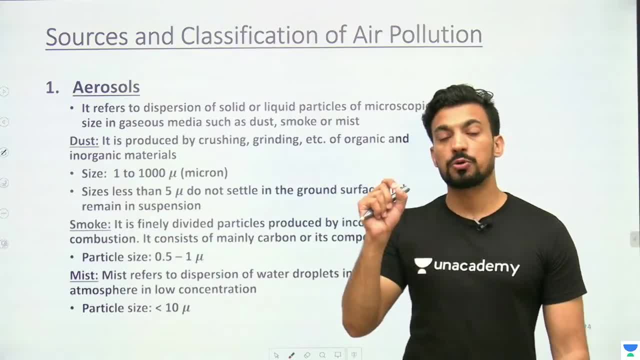 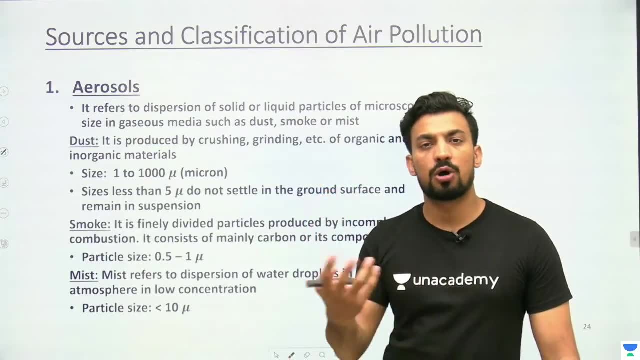 Whatever smoke is burning, the smoke coming out from it. now, what do you see in the smoke? The particles that are not burnt properly. you are doing a bonfire, so the smoke that comes out from that smoke, that wood particle or coal that you used, that which was not 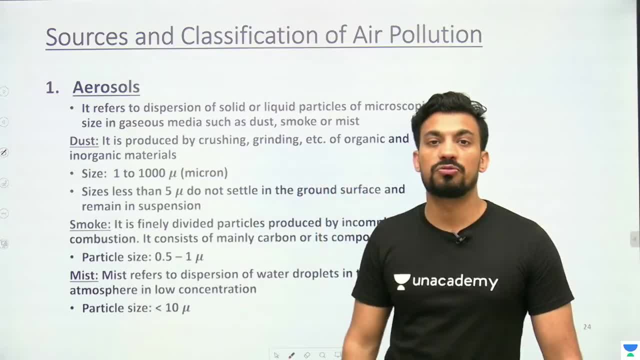 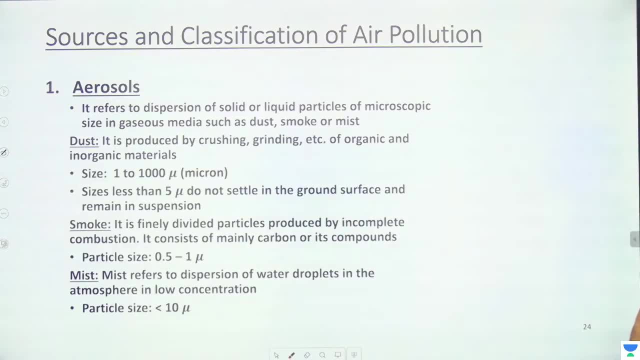 burnt completely. that which was not burnt completely is taking the form of smoke there. So what will happen in the smoke? It is finely divided particle produced by incomplete combustion. Incomplete combustion- it is not burnt properly. that is why it is called carbon and its 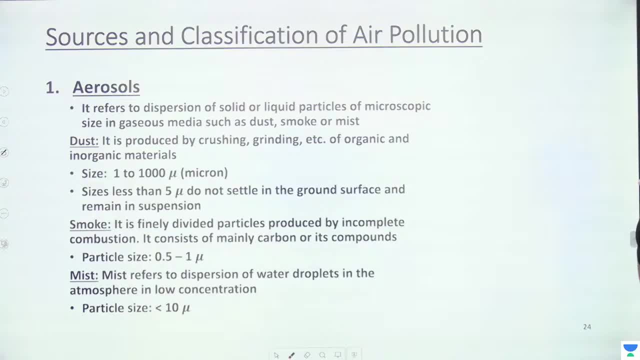 compound. The size of the particle will be between 0.5 to 1 micron. Then comes mist. What does mist mean? The droplets of water, very small particles- 10 microns, small particles of water are called mist. Then comes fog. 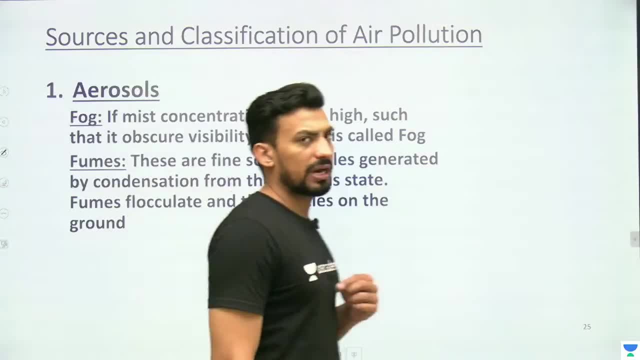 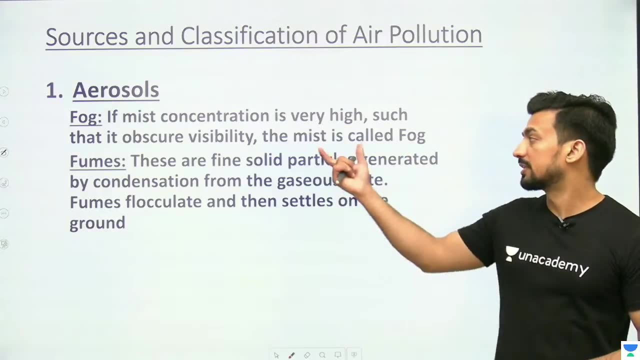 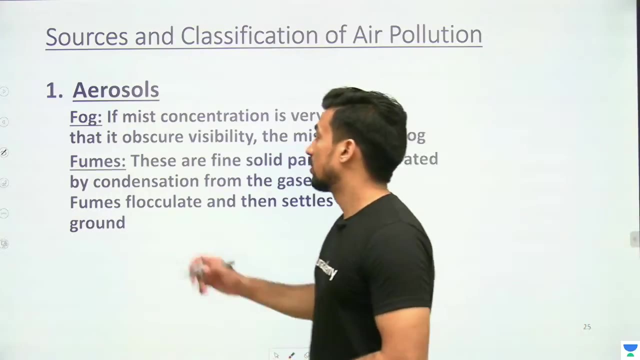 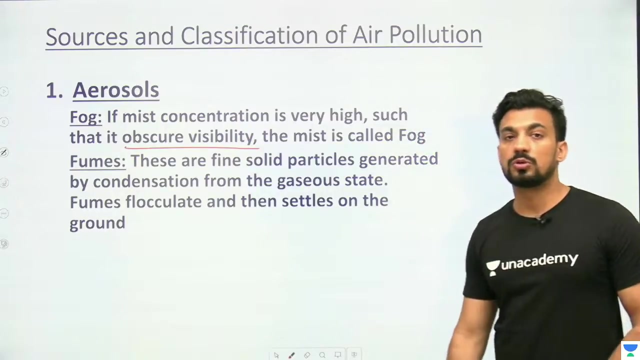 If the concentration of mist is high, the particles of water, which are very small particles which you see in winter. what do we call it? We call it fog, When the mist concentration is very high, due to which the visibility of obscures becomes a hindrance. 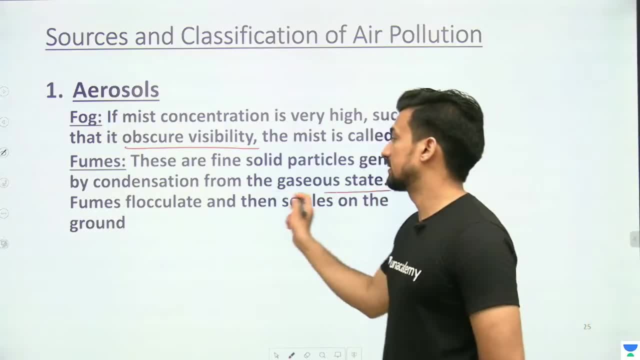 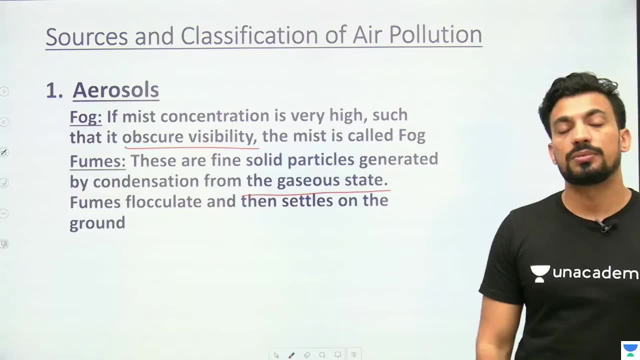 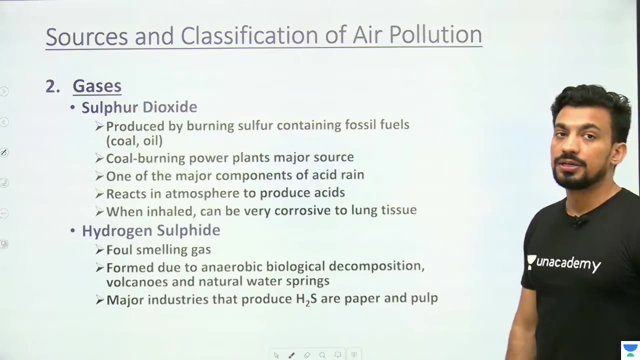 visibility is not visible there. The gaseous state is solidified here, and then those small particles are called fumes. We call them fumes. Now, what gases are there? Let's talk about them: Sulphur dioxide, Hydrogen, sulfide. 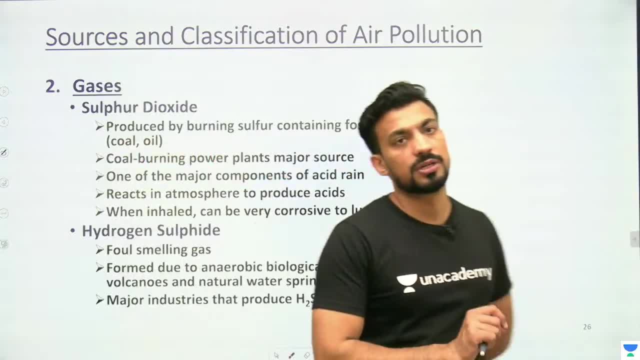 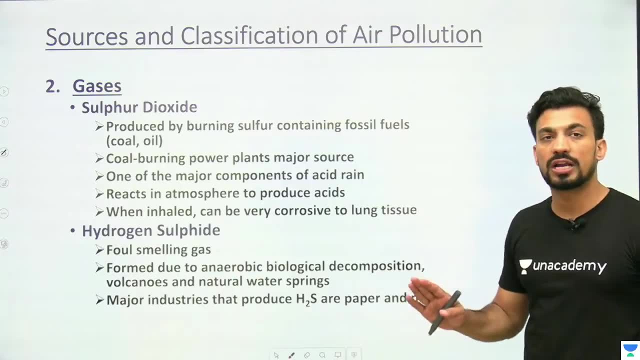 Now there are basic things about them which we have read till now. you are just looking at the same thing here. so what you will get from them? Sulphur dioxide is released here. coal burning power plants are the main source of coal burning power plants- Sulphur dioxide. 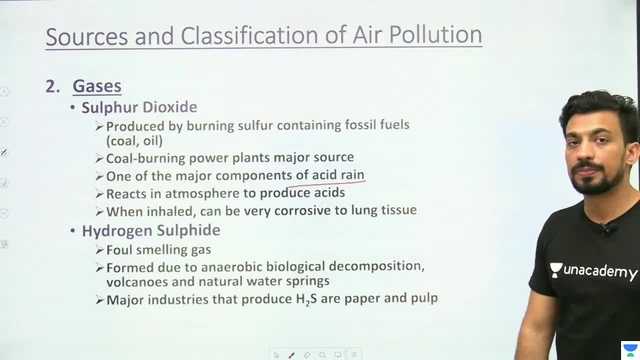 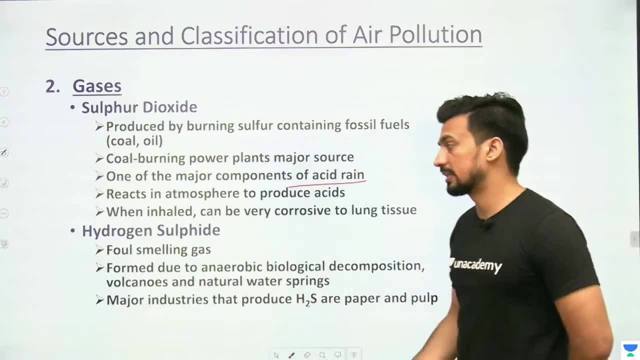 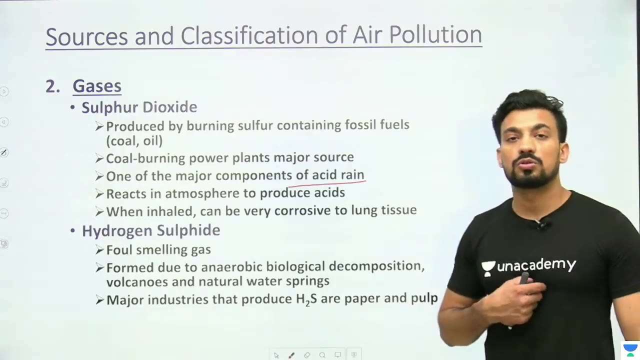 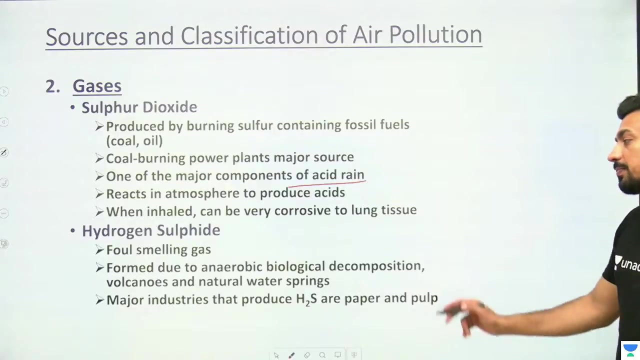 is released from them. one of the major components of acid rain is obvious. we also know this reacts in atmosphere to produce acids, and acid is produced in the western hemisphere, in the western hemisphere and in the western hemisphere. 英文, the word acid is called as an alcohol. 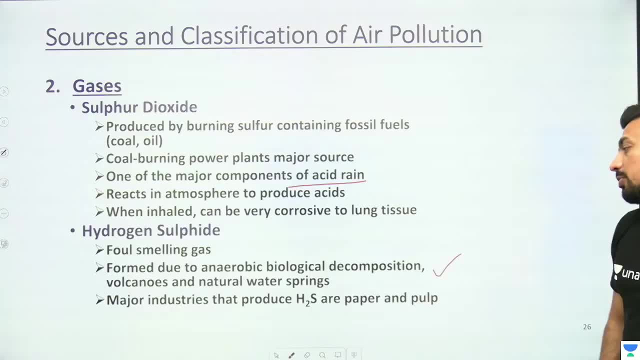 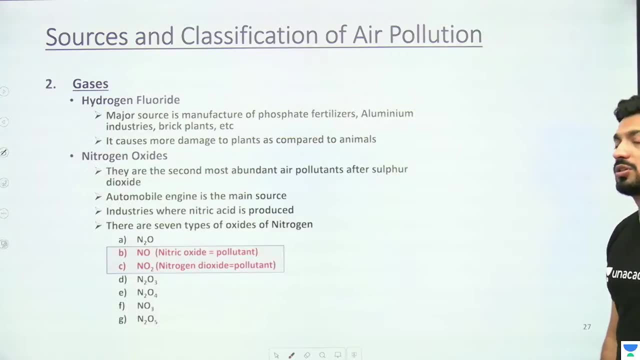 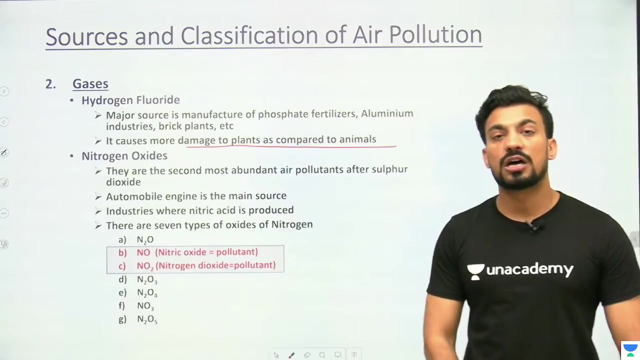 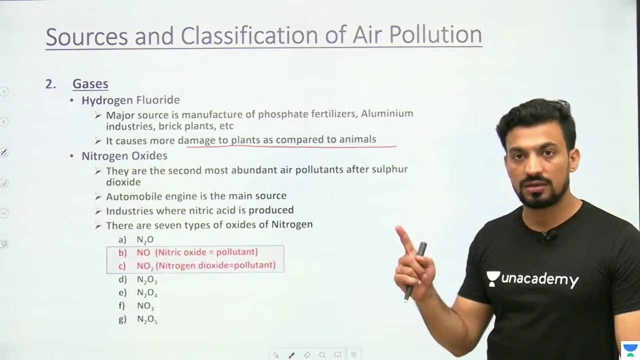 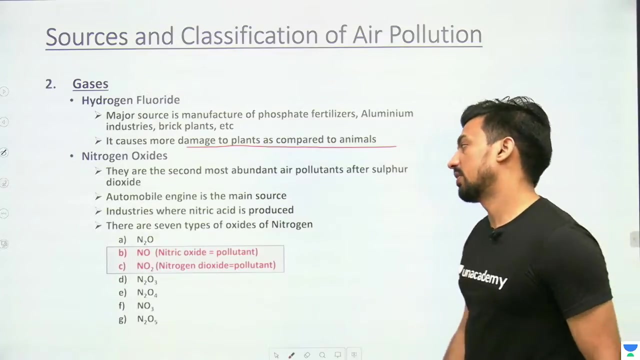 acid and there found oxygen in the sea. Hydrogen Fluoride is generated from Phosphate, Fertilizer, Aluminium Industries, Brick Plants, etc. Hydrogen Fluoride damages plants more than animals. Nitrogen Oxides are harmful or not. Nitrogen Oxides are harmful or not. 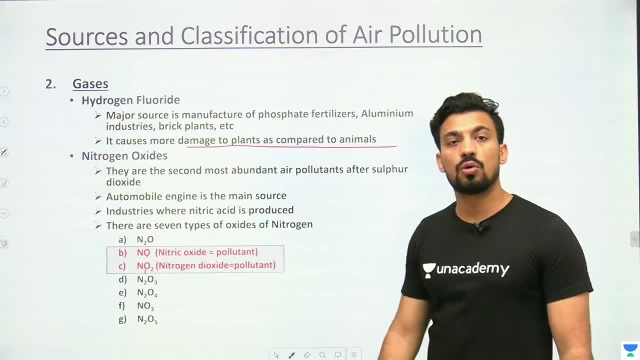 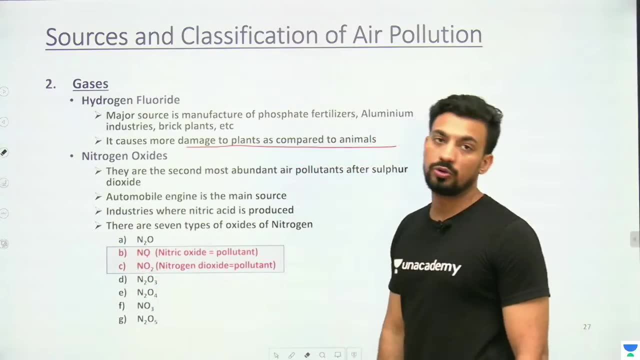 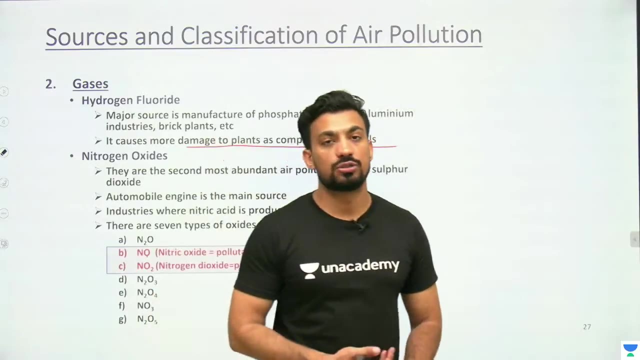 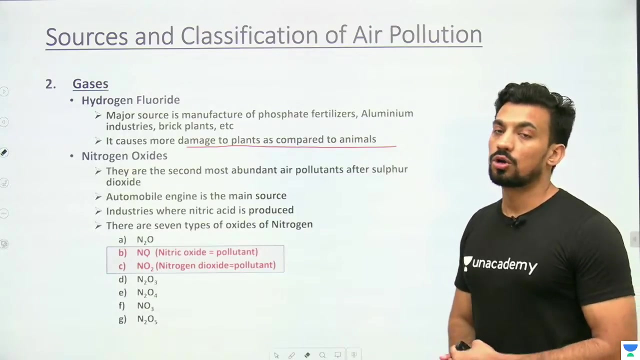 Nitrogen Oxides are pollutants or not. Nitric Oxide and Nitrogen Dioxide- Nitric Oxide and Nitrogen Dioxide are pollutants or not. Nitric Oxide and Nitrogen Dioxide are pollutants or not. Automobile Industry or Automobile Engine is the main source of Nitrogen Oxides. 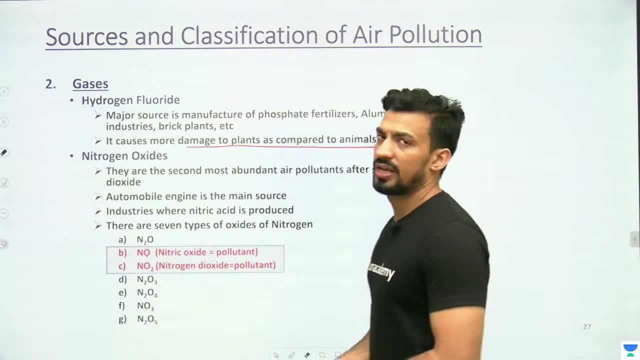 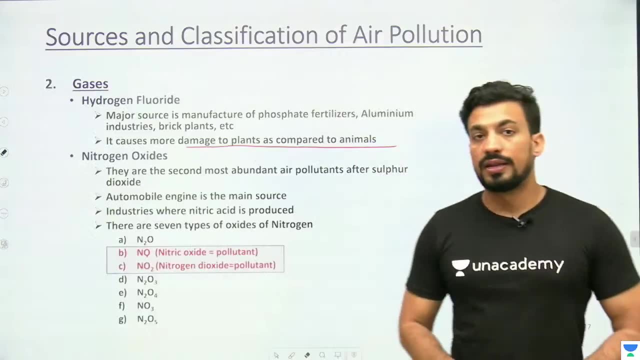 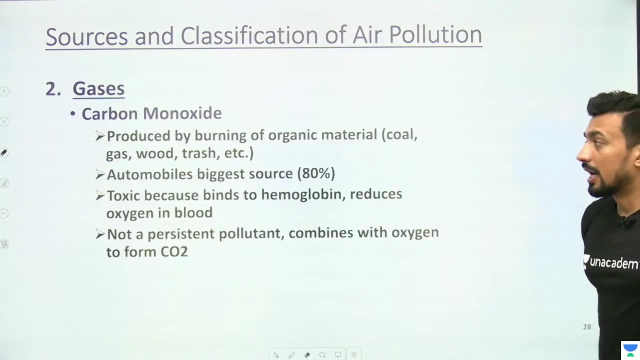 They are the second most abundant air pollutant after Sulphur Dioxide. After Sulphur Dioxide there are Nitrogen Oxides. After Sulphur Dioxide there is Nitrogen Oxides. Next Industries where it is produced. Next Industries where it is produced. 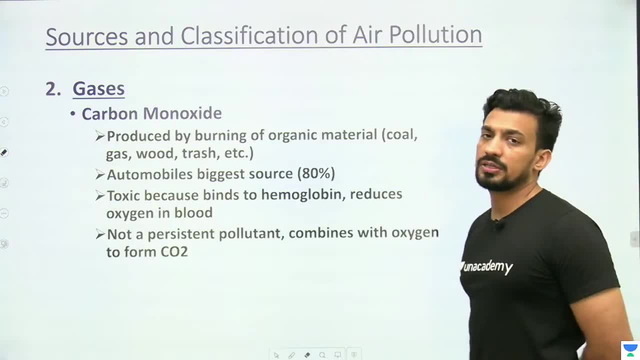 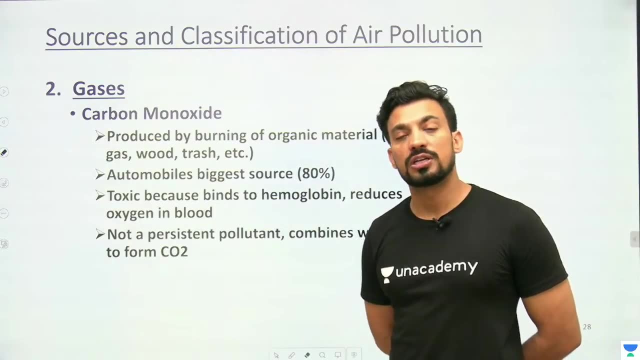 Carbon Monoxide. It is burning. You must have read in news that some people took a sleeping pill in the night. The room was closed in one room. Why they died? Because there was incomplete combustion. Carbon Monoxide became carbon monoxide. It is attached to the body. the body could not get oxygen, due to which it died here. 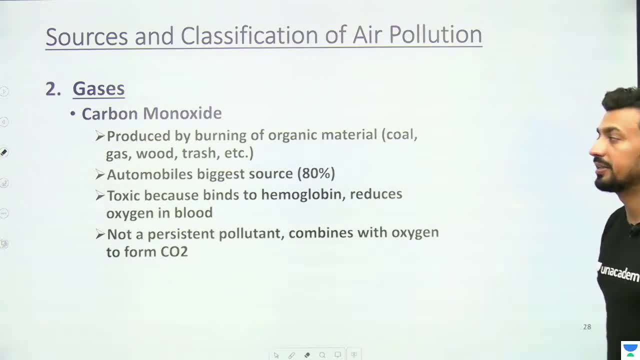 So carbon monoxide is produced by burning of organic material, coal, wood, trash, whatever garbage you have burnt. Automobiles are the biggest source. It is toxic because it binds with hemoglobin and will not allow oxygen to enter the blood, Not a persistent pollutant. along with oxygen, it makes carbon dioxide. 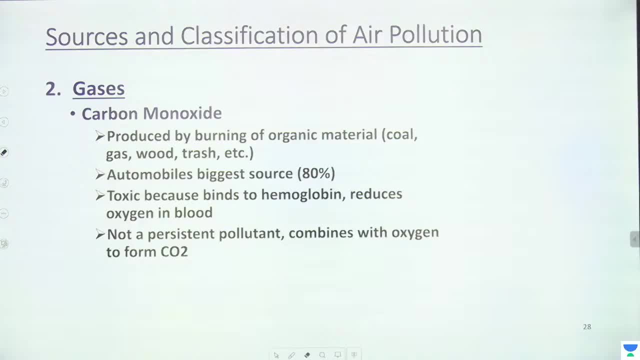 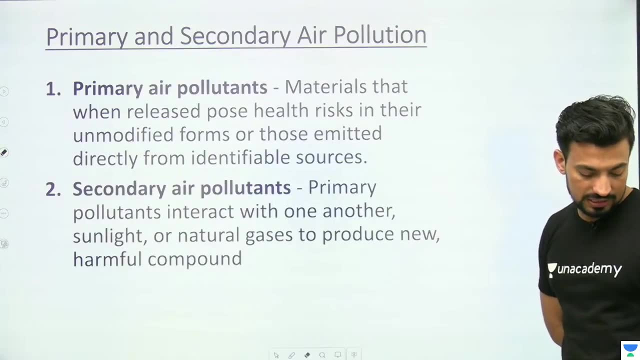 But it does not mean that this carbon monoxide always remains in the form of CO. Friends, after that comes the primary and secondary. Now wake up here. I know that the stories are going on for a long time. Wake up a little. the questions come from here. 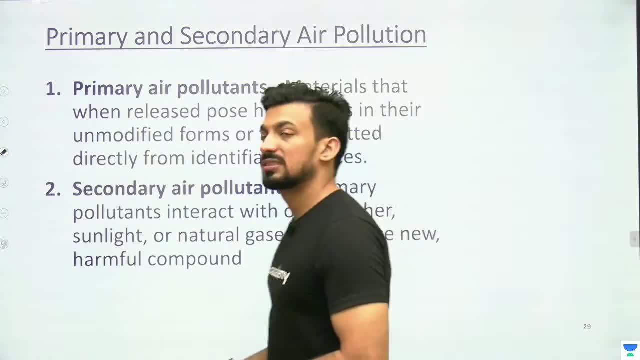 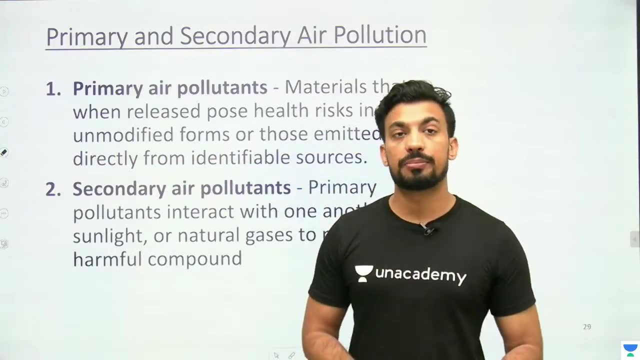 Look, the questions have come. Which is the primary and which is the secondary air pollutant? These questions have been asked. It will not ask you so much details, but it asks you so much in the objective: Which is the primary and which is the secondary? 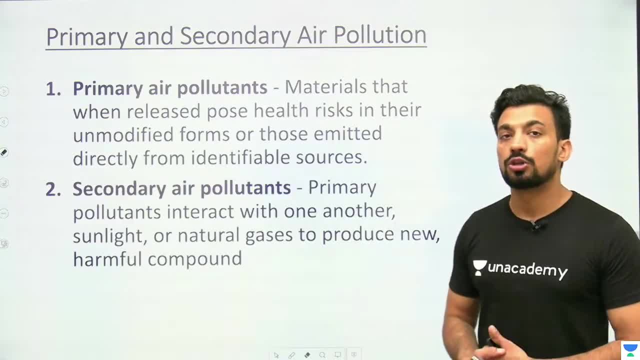 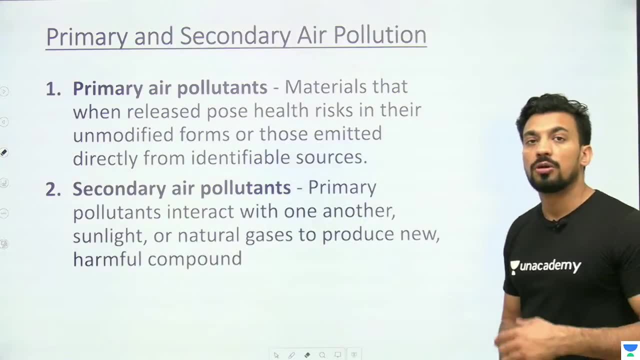 So you know these things And you will write in these short notes here. So what comes in the primary air pollutant Materials that, when released, pose health risks in their unmodified form? They have not been modified. they have not been found with any other compound. 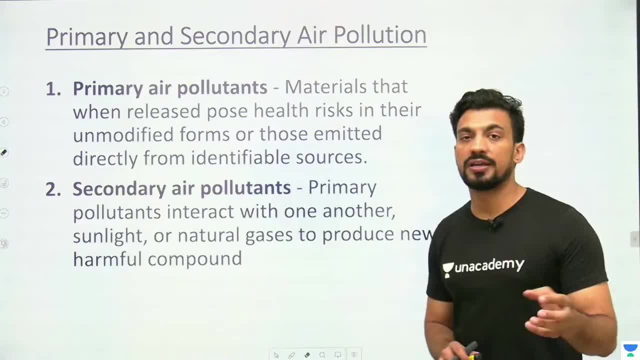 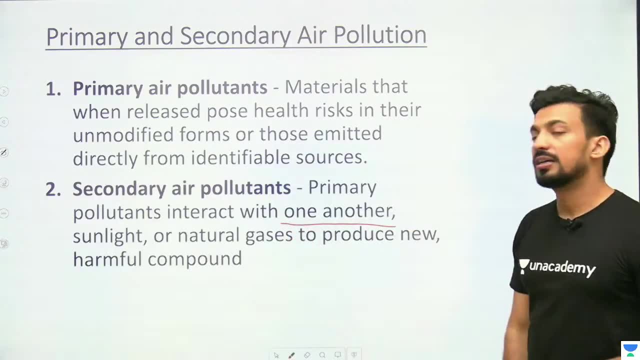 They are present in their original form, so they will be called primary. What will come in the secondary? They will interact with someone else. After interacting with someone else, or after interacting with sunlight, After interacting with natural gases, they make another harmful compound. 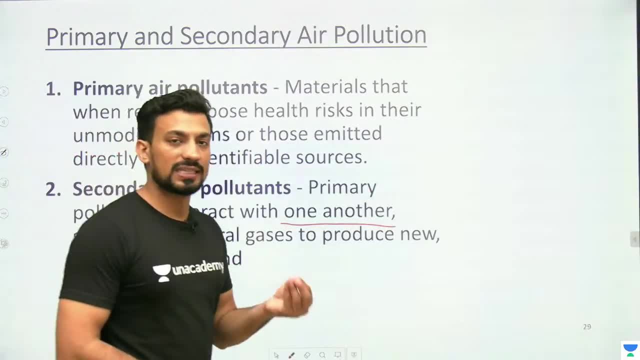 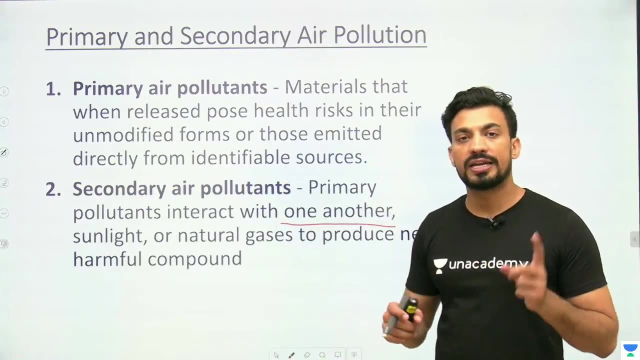 So what do we call this Secondary? Primary: is such a substance or such a pollutant which is a pollutant in itself? Secondary: two different pollutants have been found, or one pollutant has been found with something else, Like sunlight is not harmful for us. 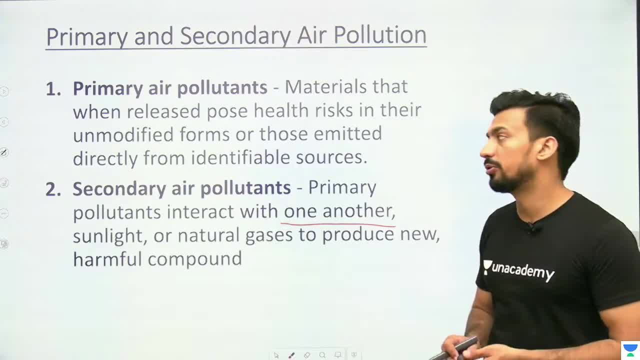 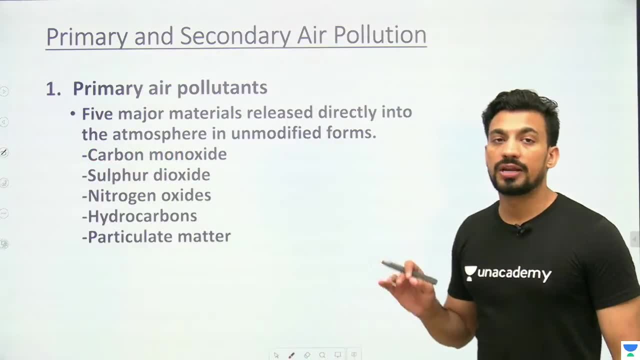 But in its presence, what happens? further Secondary air pollutant is made here. So in the primary you have five major air pollutants. Remember carbon dioxide, sulfur dioxide, carbon monoxide, sulfur dioxide, Carbon monoxide, sulfur dioxide, nitrogen oxide, hydrocarbon and particulate matter. 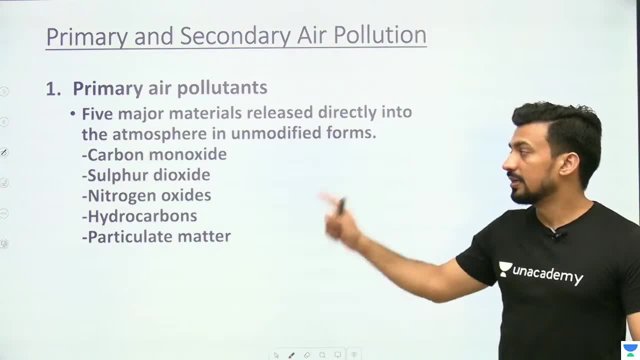 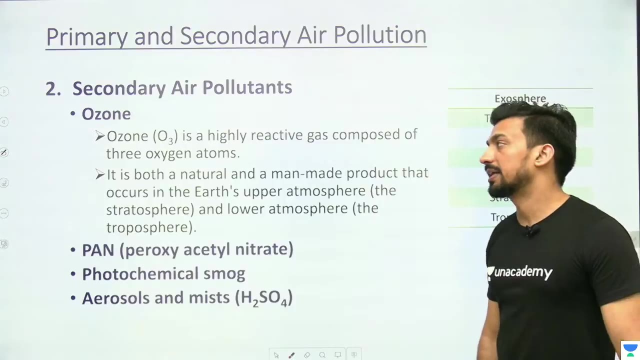 This is the primary air pollutant: Carbon monoxide, sulfur dioxide, hydrocarbons, particulate matter, Carbon monoxide, sulfur dioxide, nitrogen oxide, hydrocarbons and particulate matter. If we talk about the secondary, then you have ozone in it. 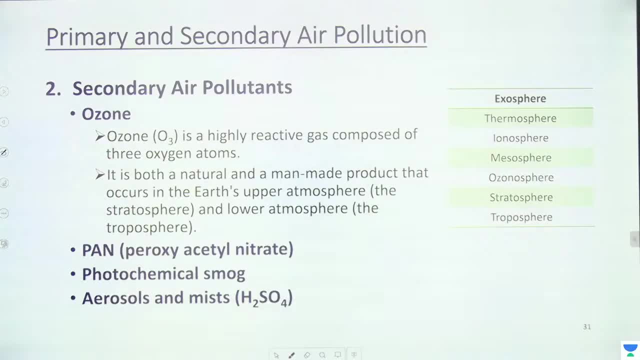 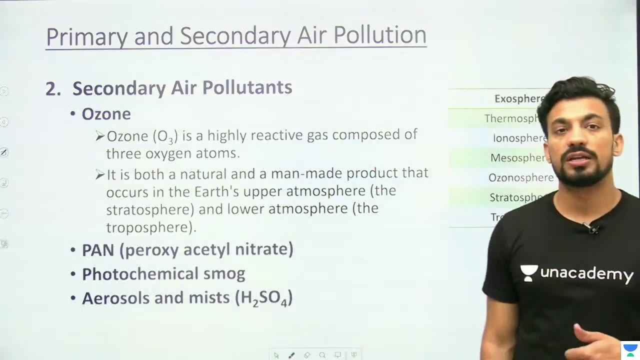 It is highly reactive, Composed of three oxygen atoms. It is natural and man-made product which exists in the upper atmosphere of the earth. It is air pollutant. It does save us from harmful rays of the sun, But it is also an air pollutant. 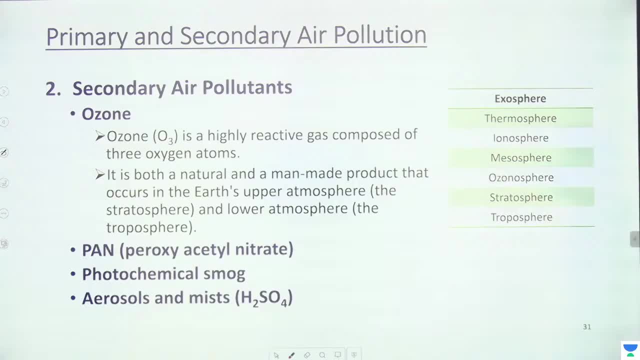 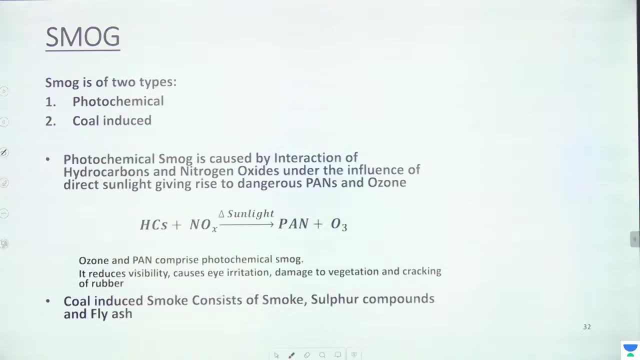 Ozone is highly reactive gas composed of three oxygen atoms, both natural and man-made. Then comes peroxyacetyl nitrate, photochemical smog, aerosols and mists. What is smog? What is smog? Smog is of two types. 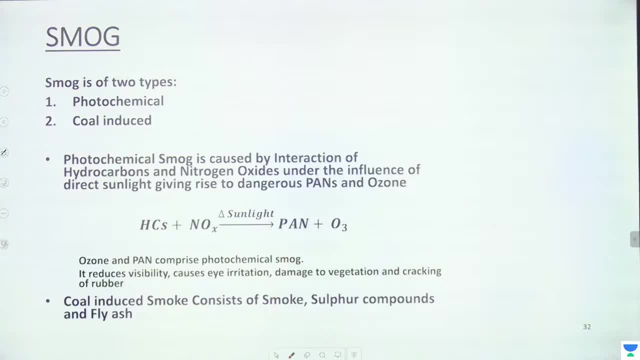 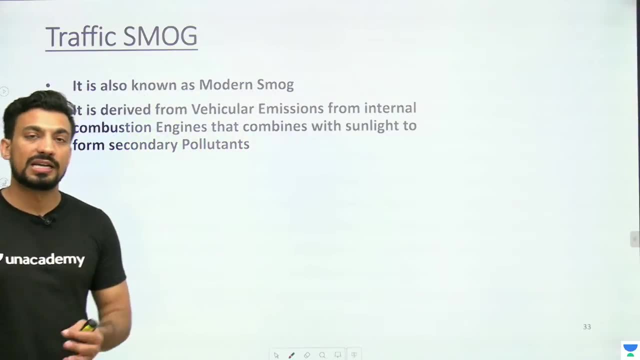 One is photochemical and the other is coal-induced. If we are reading from our childhood which we used to call as modern smog or traffic smog, What did we read in our childhood? We used to read this modern smog or traffic smog. 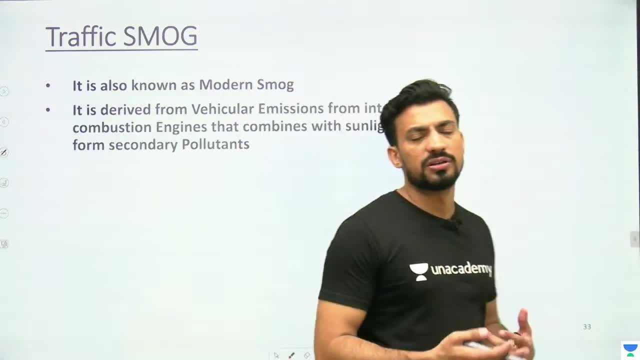 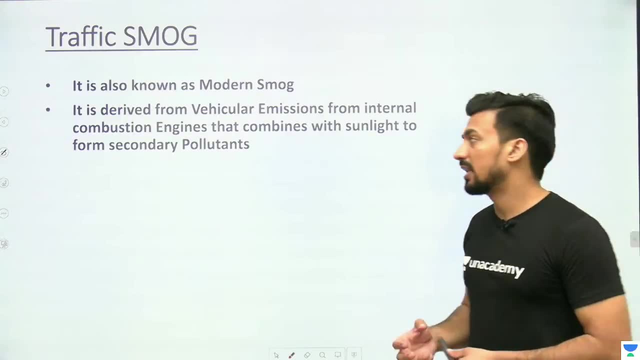 What happens in this? Whatever is the vehicle, whatever is your traffic, whatever waste is being generated from the traffic, the gases that are coming out there, those gases are in the presence of sunlight. in the presence of sunlight, what do they make? 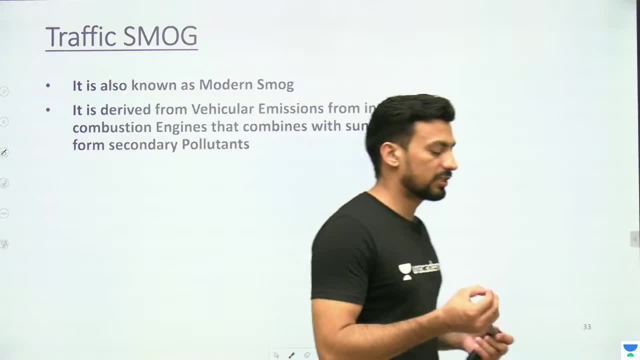 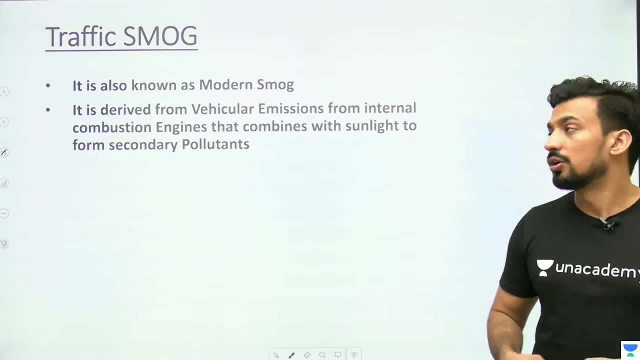 They make smog, Or in the environment, the particulate matter or the droplets of water, the fog. that has happened. what will it do with them? It makes smog here. So this is modern smog, or traffic smog. 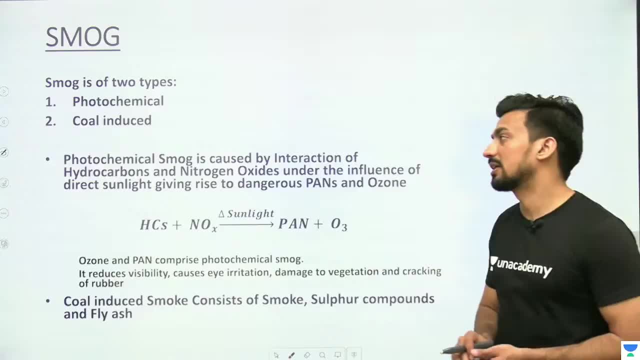 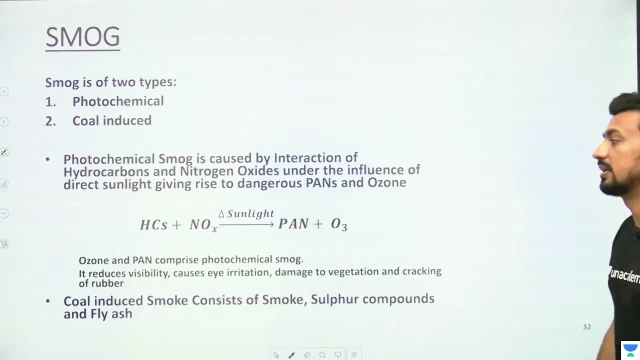 And now what we are reading. which one are we talking about Now? we are talking about which smog? Photochemical smog. So what is happening in photochemical smog, Whatever hydrocarbons are there, with nitrogen oxides and in the presence of sunlight? 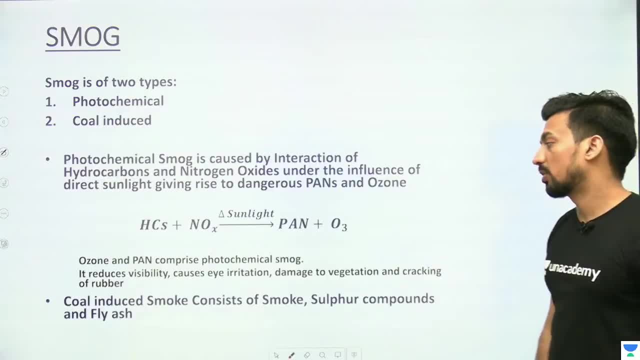 what do they make? They make a pan. What was the pan? Peroxyacetyl nitrate. They make peroxyacetyl nitrate here And along with that ozone is released here. Ozone and pan- they make photochemical smog together. 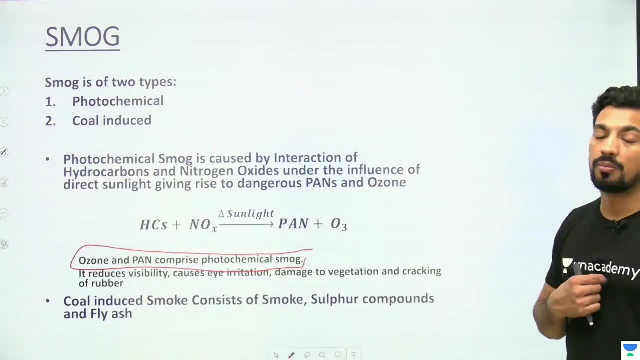 Which is what happens for us. There is an air pollutant here. What will happen because of this Visibility? there will be a problem in seeing, there will be irritation in the eyes here. there will be damage to vegetation, cracking of rubber, etc. 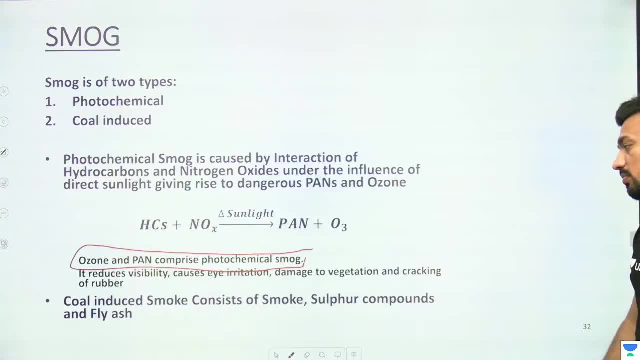 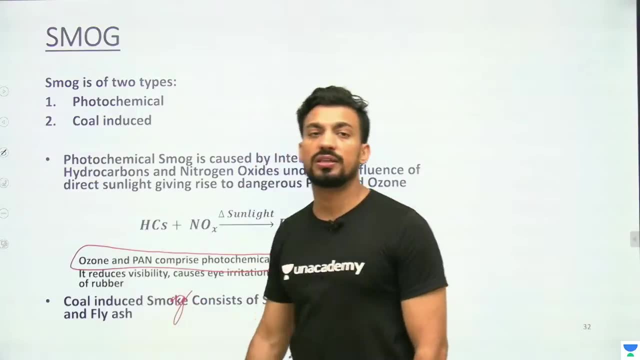 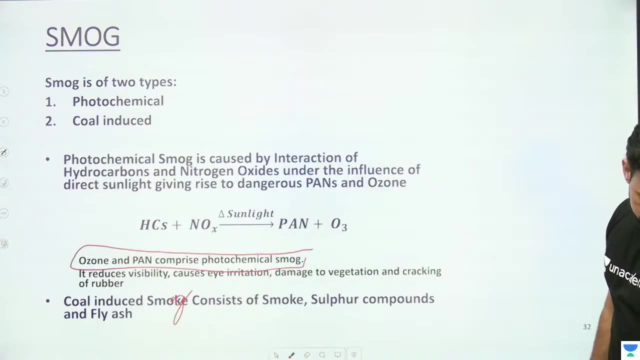 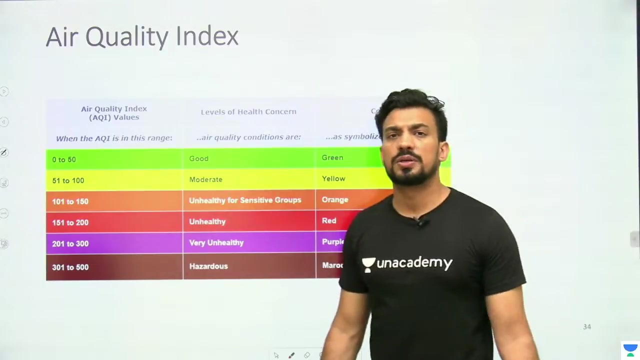 Coal induced smog consists of smoke, sulphur compounds, etc. So the smog made from coal, the coal induced smog, will have fly ash, sulphur or other compounds. Next, air quality index. You all know air quality index. 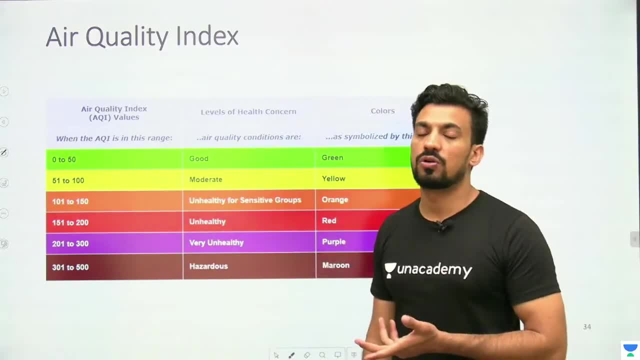 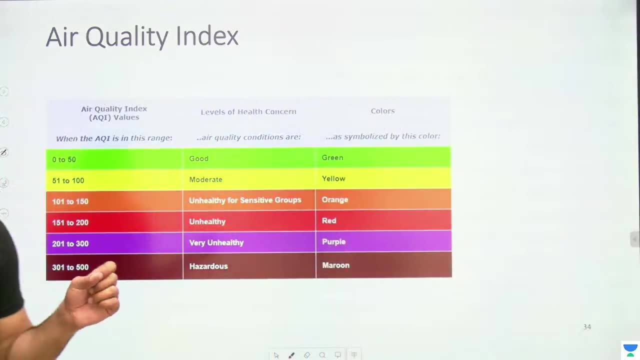 If you google your area today, now you search what is the air quality index of Delhi, Jaipur, Bangalore, Indore, wherever you search Kolgata, then you will get the air quality index. In many cities there are screens. 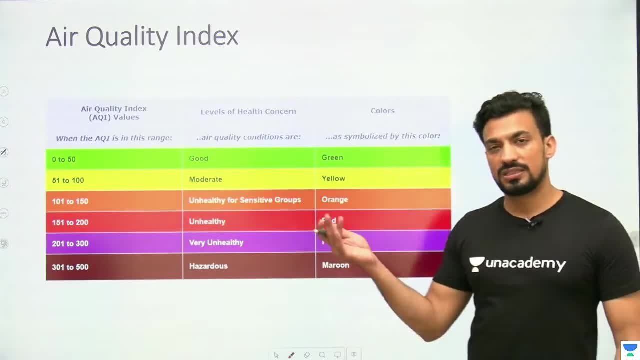 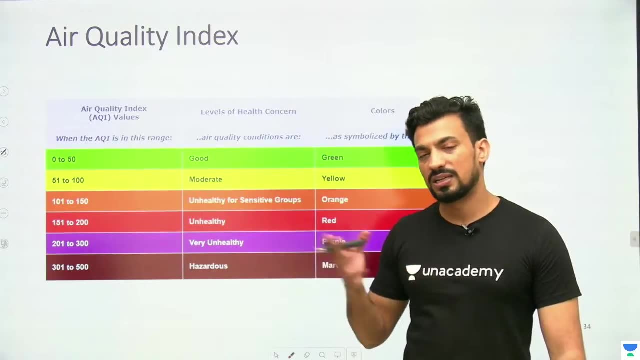 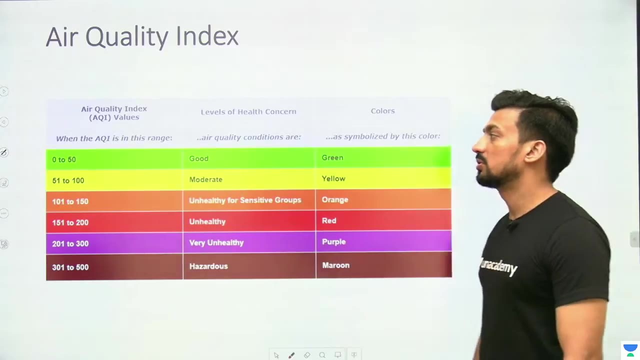 that the air quality index is visible there. There are also titles below that. it's time to do yoga. you can do yoga in fresh air. So by doing this, they keep telling the air quality index. How is the air quality here? Between 0 to 50,. 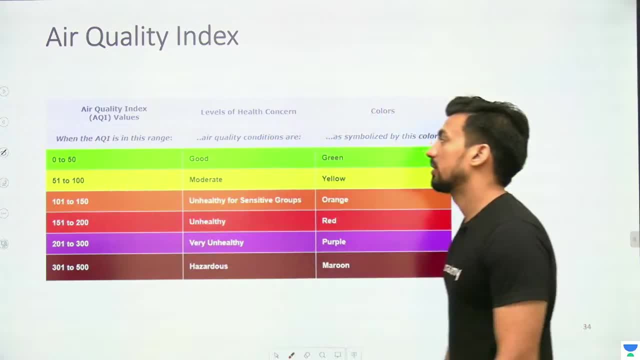 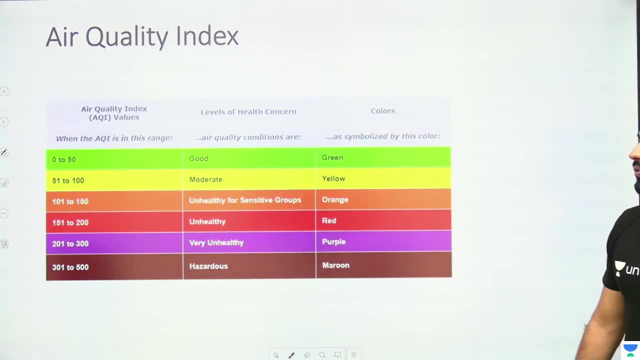 there is the value of AQI, that is, the air quality index. So you say that the air quality is good. What do you symbolize with green color? 51 to 100 is moderate. from yellow 101 to 150 is unhealthy. 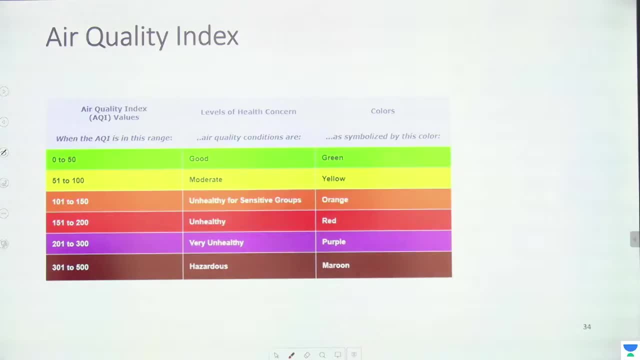 for sensitive groups, who are aged people or who are sick or children. it is unhealthy for them. We will denote with orange: 200 to 200 is unhealthy. We will denote with red: 201 to 300 is very unhealthy from purple. 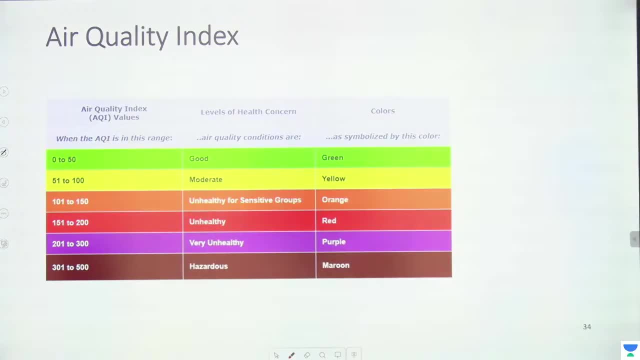 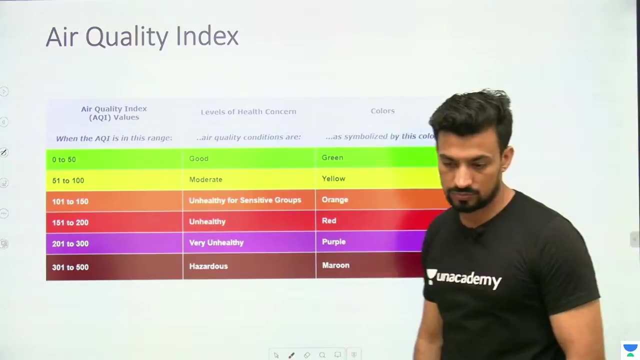 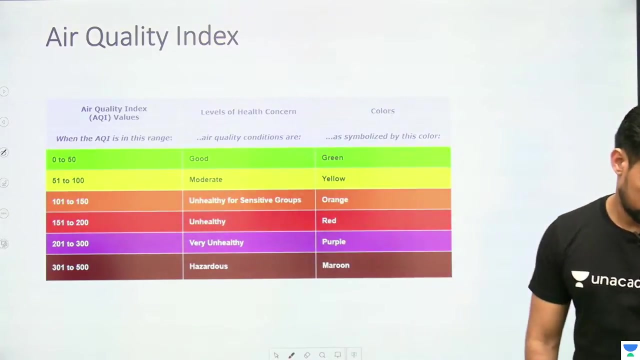 301 to 500 is hazardous. It is very dangerous. Maroon color will be visible. It will be visible in blue. If I talk about this here, it is showing 164.. PM 2.5 is the main air pollutant as of now. 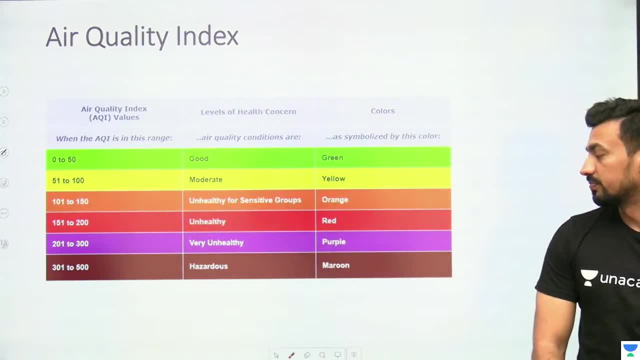 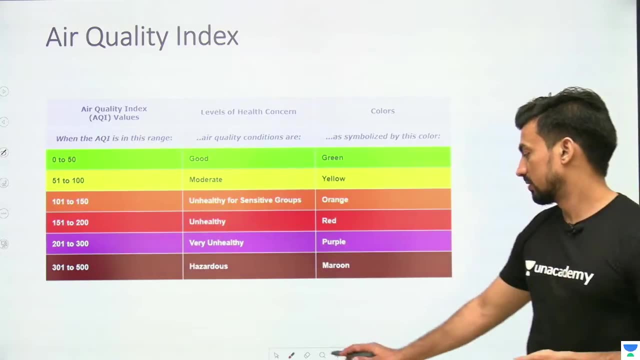 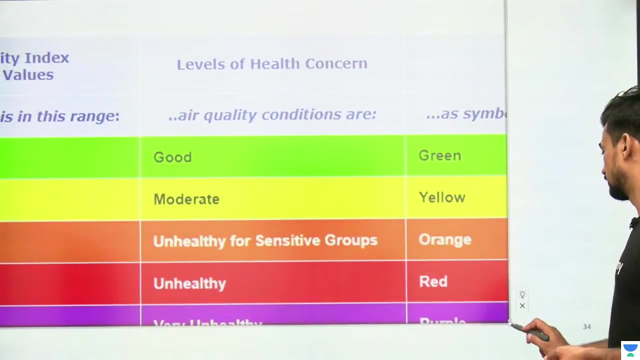 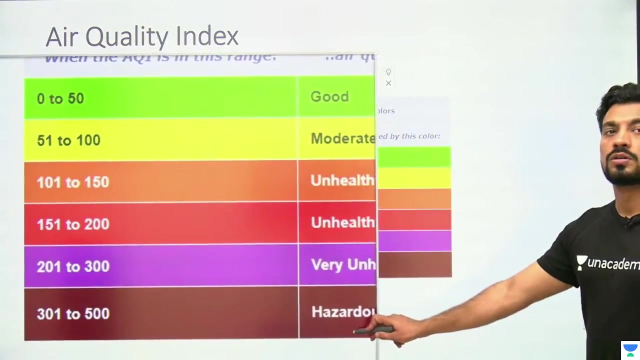 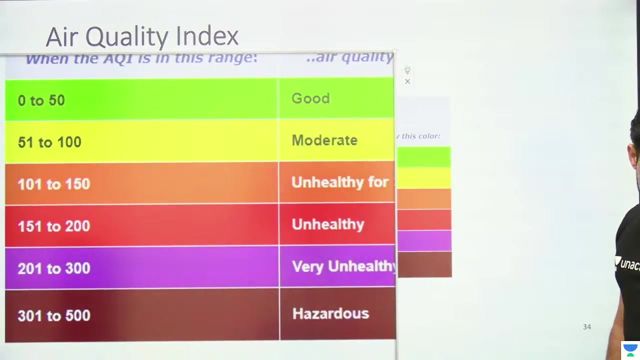 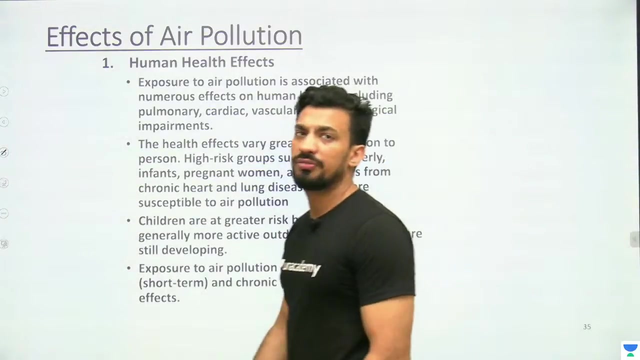 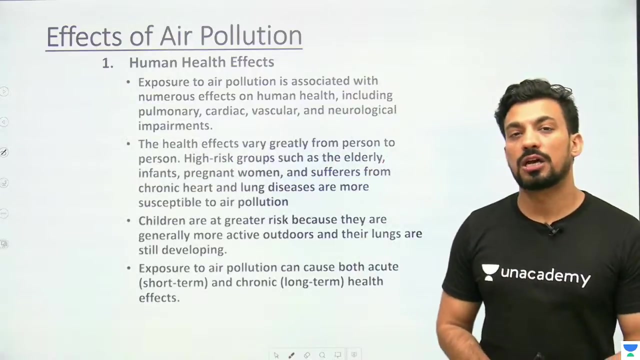 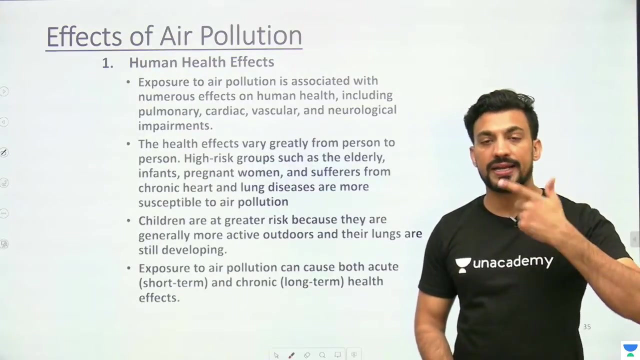 so it means it is unhealthy, it is in red condition? it is not clear. see it clearly, friends. let's talk about the effects of air pollution. what are the causes of air pollution? if you are taking a simple breath, if you are talking about our nose, then whatever is the track, 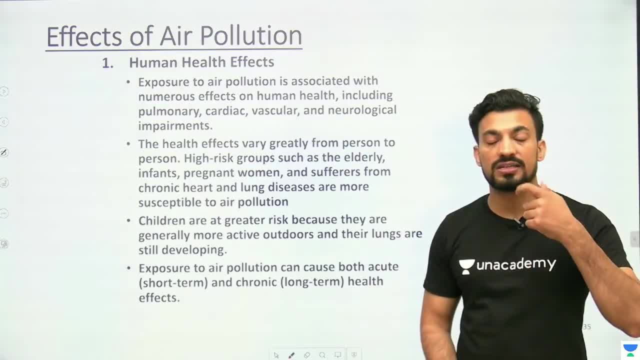 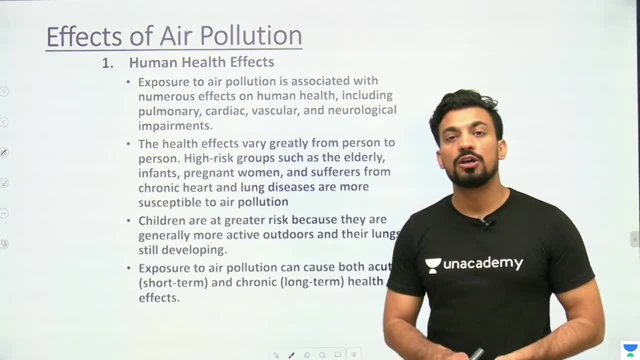 or whatever is your windpipe, or whatever is your windpipe or whatever is your windpipe, from where air and air is going, so the membranes inside it, it is like mucus, or you can say that they are sensitive. they will feel burning, they will start to get in problems. 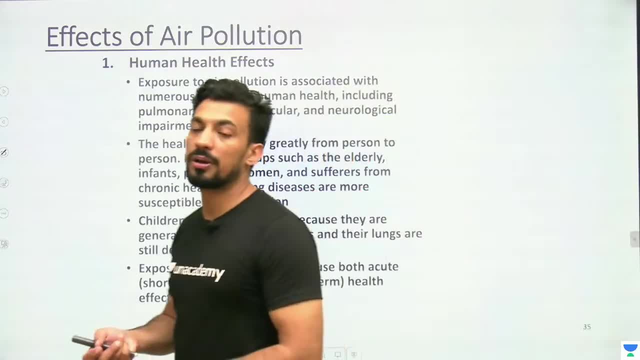 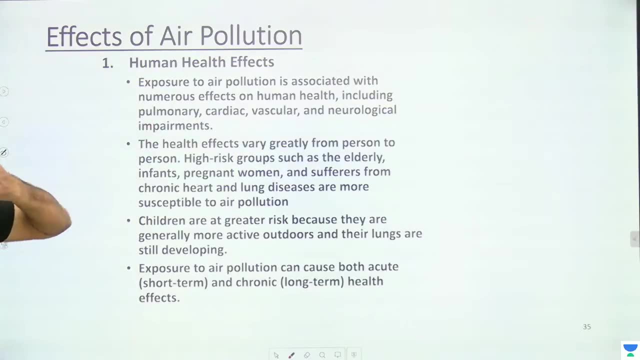 they will get burn in the lungs, they will get in problems. slowly more issues will come in the body which are related to lungs: pulmonary or lungs, cardiac, heart related, vascular, neurological impairments. it creates all these things. simple thing to say. Oxygen plays an important role in this. 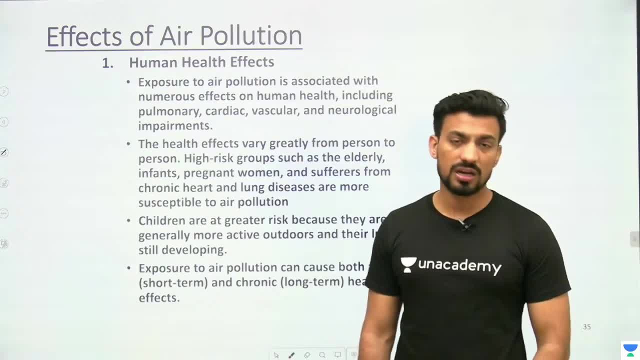 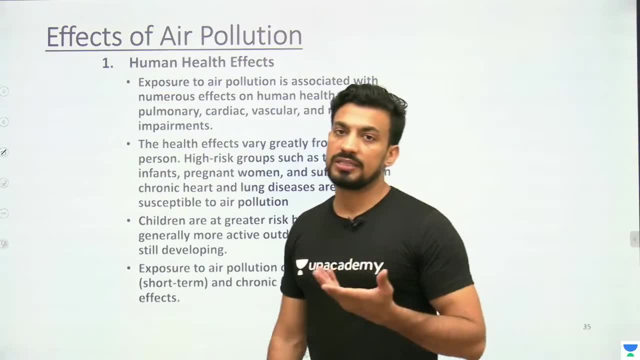 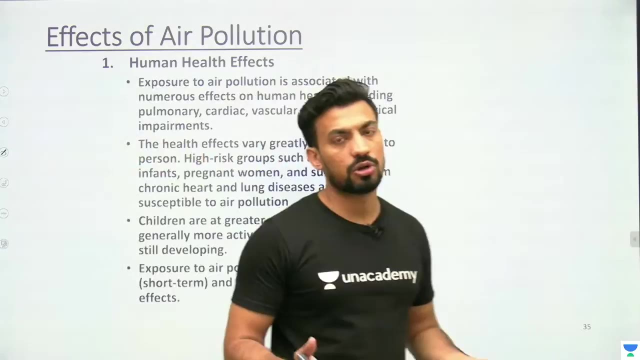 If blood is not properly given to the body, blood is not going properly to the brain. if you say that the blood is not going to the brain, there is no oxygen in the blood, then slowly your brain is controlling all your neurological activities. 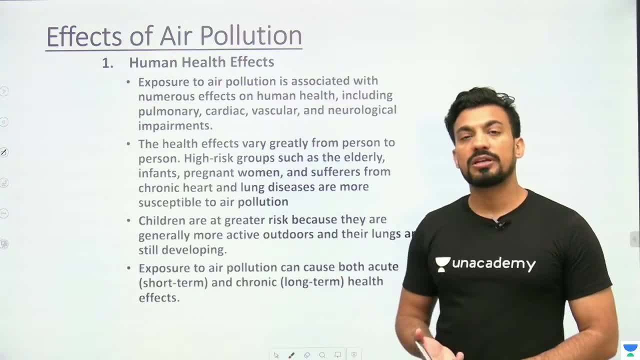 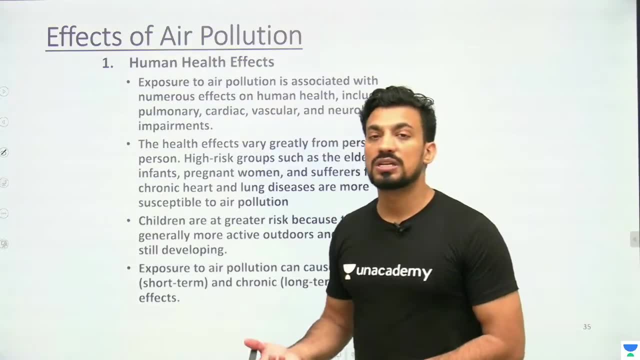 What happens with that? All this work gets affected. You must have seen that if someone has an accident and there is a lot of bleeding, then you must have heard later that that person went into a coma. Why does it happen? Because oxygen is not able to reach the body. 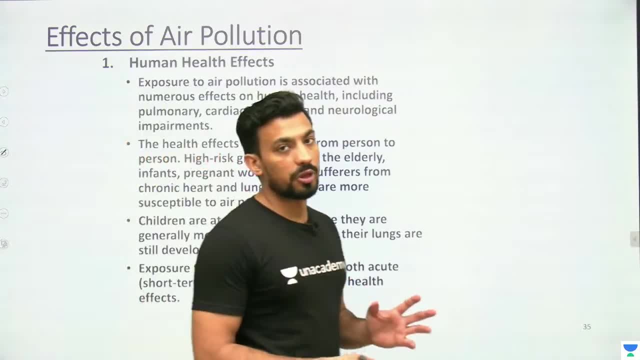 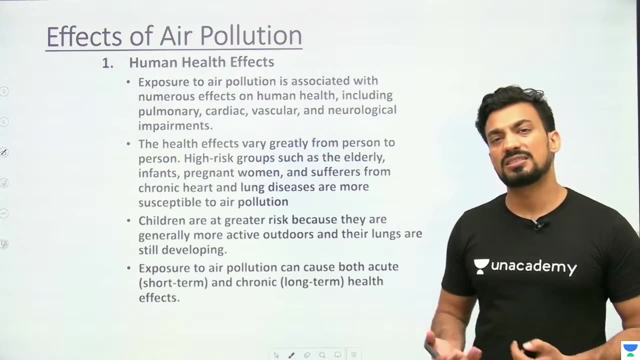 oxygen is not able to reach the brain, then its functioning will be impacted, Due to high blood loss. sometimes it happens that some parts of the body are not working, So all these reasons happen. Oxygen is playing the most important role. You know that we need it. 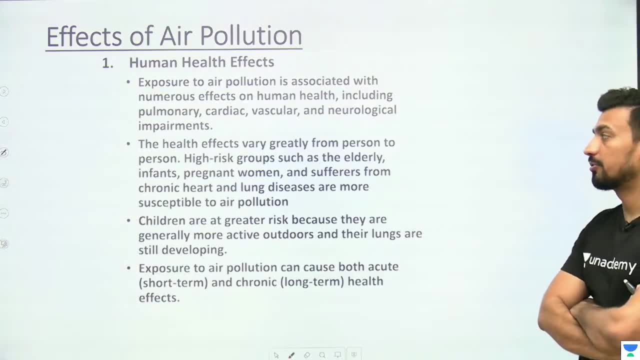 Now let's talk about the health effects may greatly vary from person to person. You may have a person to person change or health effects. Children are at greater risk because they are generally more active outdoors and their lungs are still developing. They may suffer more damage to children.